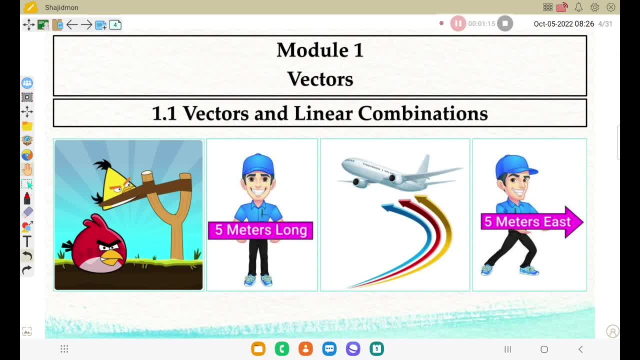 so let's start with some small example, live examples You can see here, for example, first one, you can see one game. you know the game Angry Bird, correct? So when we are doing this game, okay, we need to be careful about two things. First, 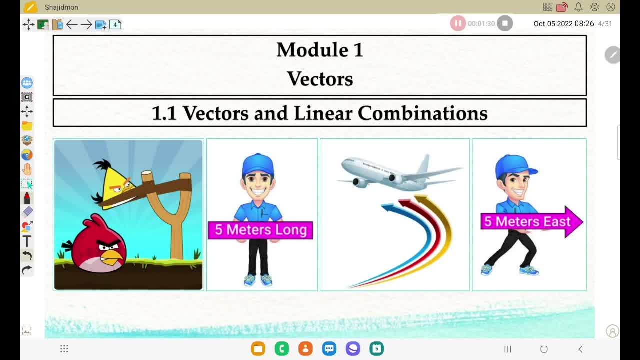 when we are stretching this bird and releasing that bird, it will hit on some bird correct Or some places. So when we are hitting, when we are concentrating this game, we need to think about what direction we need to move this bird correct, What direction And same. 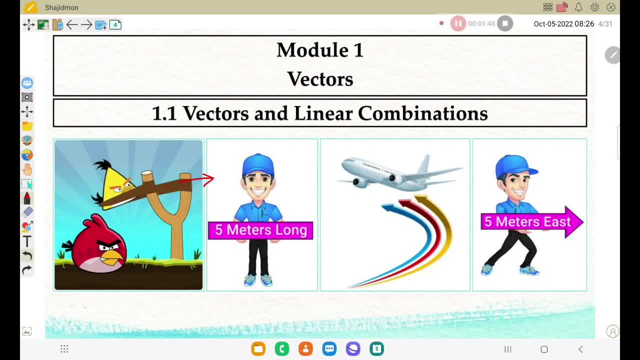 way, how much distance we need to travel, correct For hitting the bird. So two things are we need to be careful. One is about direction, correct One is about direction and second one we can say the distance or we are telling is magnitude correct. Now, the second one, see, you can see the second. 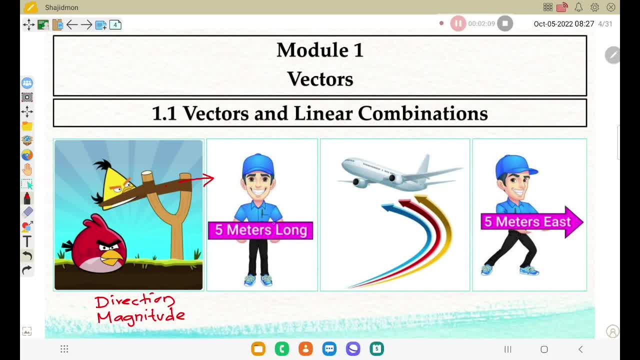 picture. Second picture: you see one person. he is telling 5 meters long. 5 meters long. He is telling about a number, correct, A length That means only he is telling about the magnitude, correct, Only he is telling about the magnitude of the. 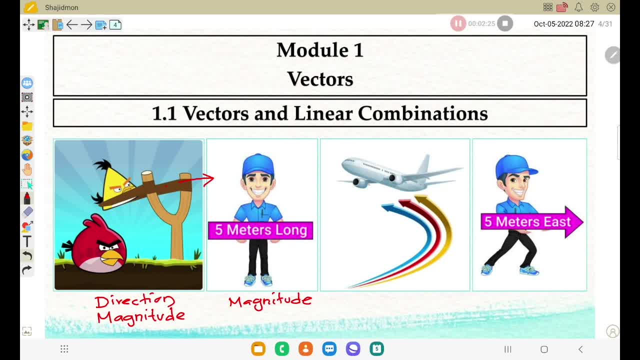 magnitude of the quantity, or 5 meters long, not direction. But in third picture you can see the flight movement. Flight movement means both direction as well as magnitude. Both are important, correct. D means the direction, M means the magnitude, So both direction. 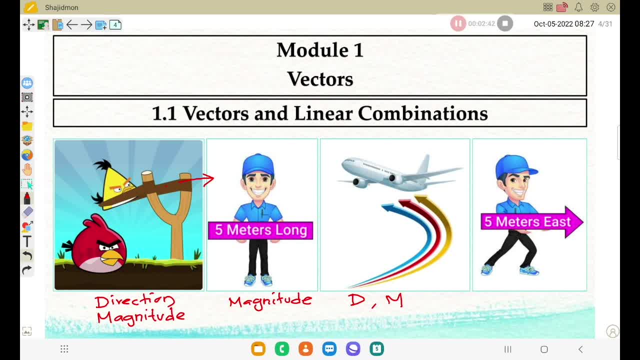 and magnitude. both are important in the flight movement because how much distance we need to travel, which direction correct? And the fourth picture: you can see what he is telling: 5 meters east. 5 meters means It is the magnitude and east means it is the direction correct. So out of these four, 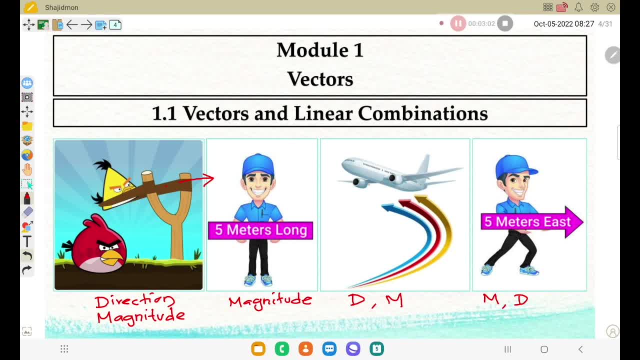 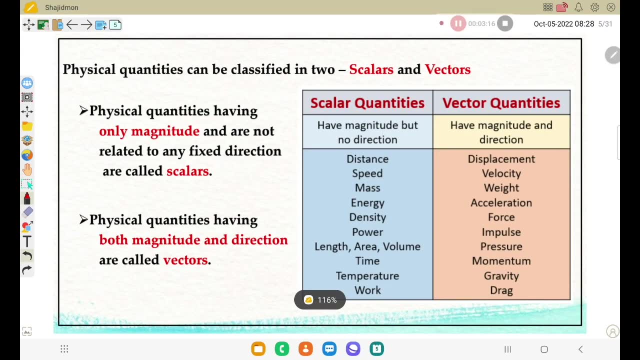 pictures. first, picture: direction and magnitude specifying. second, only magnitude, third also. fourth: also magnitude and direction is specifying. Now we will come to the point here: Physical quantities. we can divide it into two. okay, What are the two quantities? One is scalars. 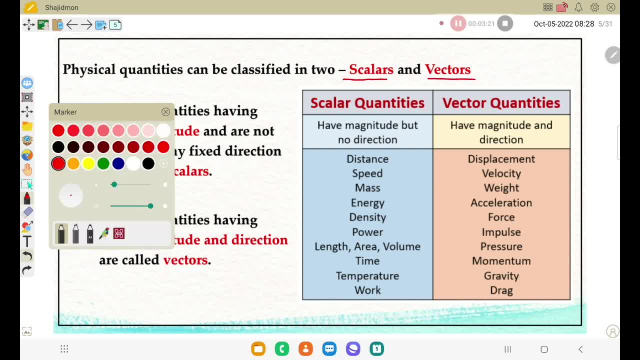 and second one is vectors. okay, First one is scalar, Second one is vector quantity. Now, what is the meaning of vector and scalar? Scalar means a physical quantity is having only magnitude. There is no direction. okay, No, fixed any. 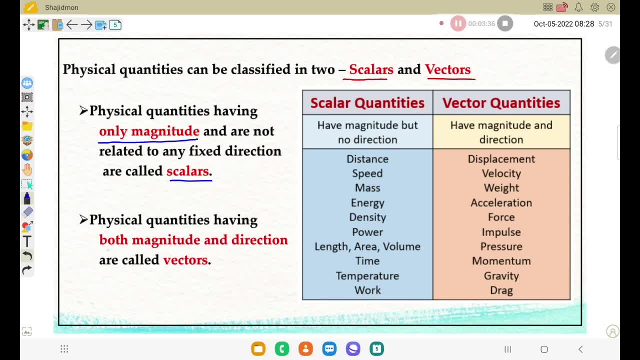 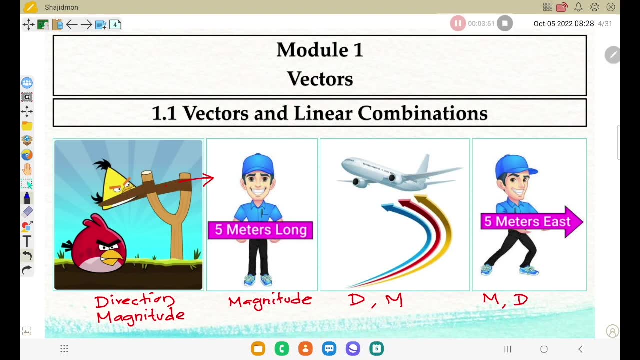 fixed direction is called scalars, Physical quantities having both magnitude and direction. we are calling it as vectors. okay, You can see on this side. okay, So in the before example, see, it depends on direction and magnitude. So it is, we can assume, like an. 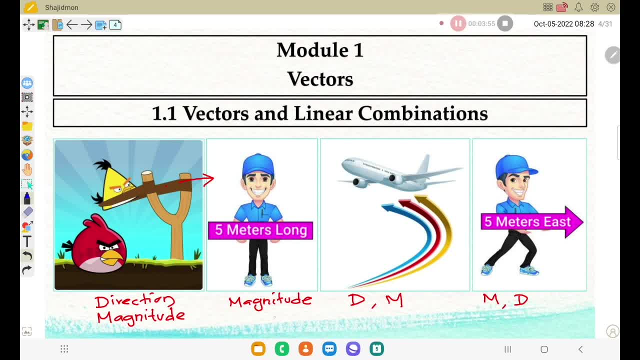 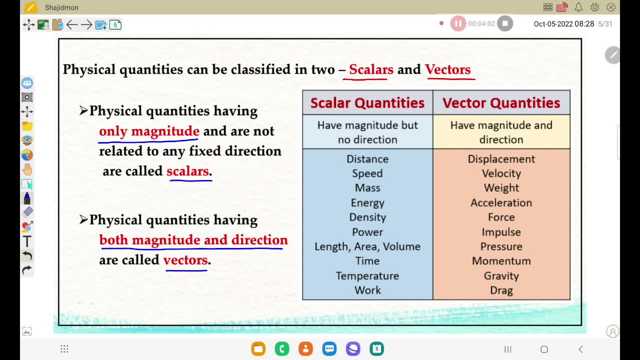 example for the vector quantity, for understanding purpose, okay. Second one is scalar quantity. third one is vector. fourth one, also vector. So scalar quantity means a quantity having only magnitude but no direction, correct? For example, distance is a scalar quantity Only. 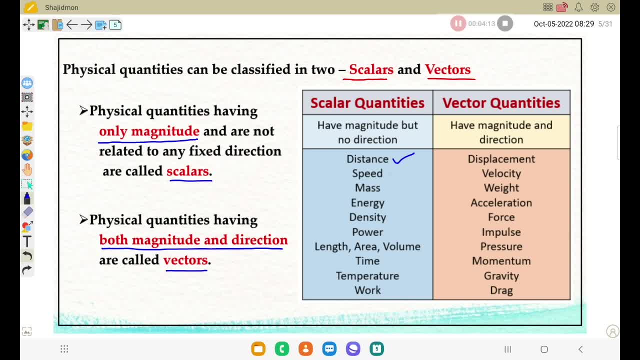 we have length, 5 meters, 6 meters, like that. correct, Speed is a scalar quantity: speed how your car is going on. correct, 30 kilometer per hour speed. okay, So only this is a vector quantity. okay, So we can assume like an example for the vector quantity: 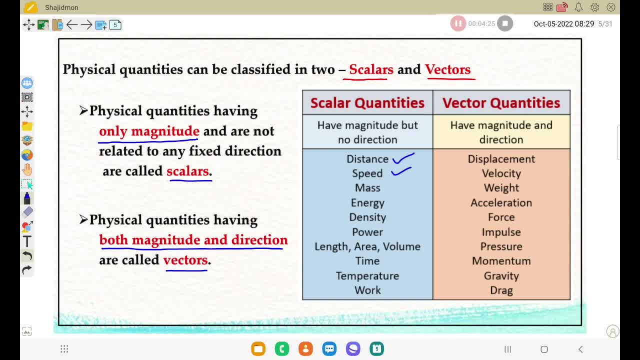 only the length, only the speed. it is telling some quantity correct Number. Now say mass. mass is a scalar quantity. energy- energy is a scalar quantity. okay, How much calorie? that is the meaning, energy correct. And density is a scalar quantity, power. power means 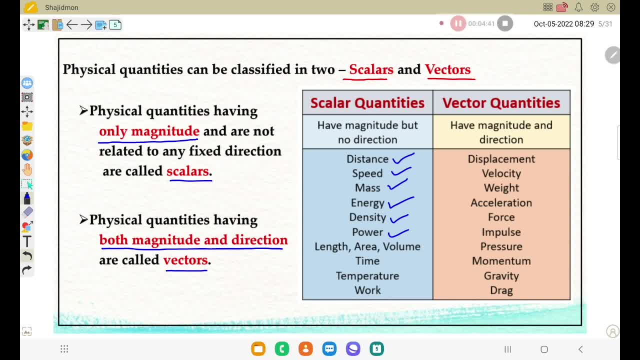 you know electric power watt- how much watt one electric bulb, something like that. Length, length means only a number, scalar quantity: area, how much square feet or meter square or centimeter square. And oleum, oleum is a scalar quantity: how much meter cube or centimeter cube, like that. 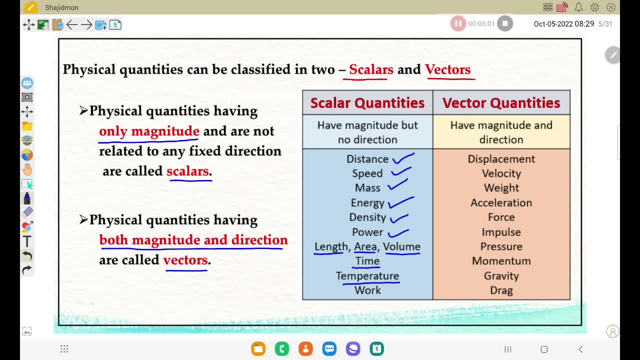 okay, Time is a scalar quantity. temperature is a scalar quantity. temperature, how much degree Celsius? or okay, That is a scalar quantity. work is a scalar quantity. Now, what are the vector quantities? you can see Quantities having both magnitude and direction. 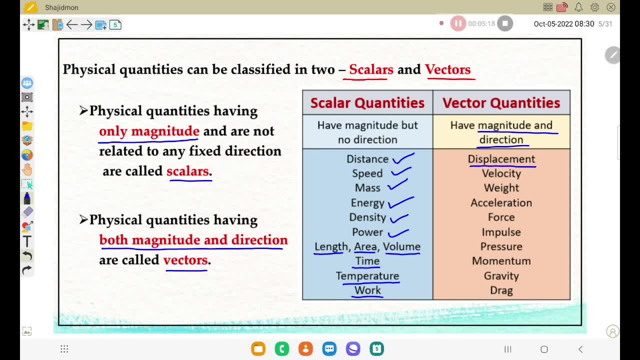 So displacement is a scalar quantity. Displacement means the directed distance, correct Distance with the direction displacement. Velocity is a vector quantity because velocity means speed with the direction correct. So we can say simply like that velocity is a vector quantity. weight is a vector quantity. 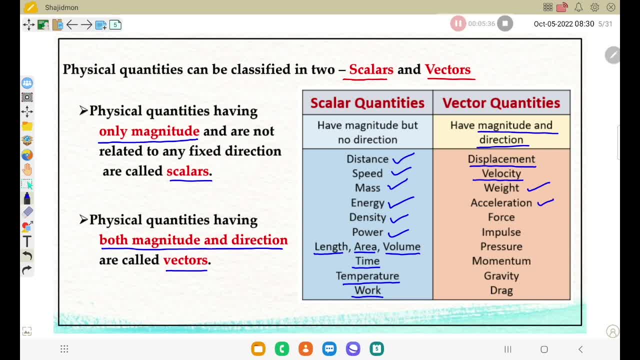 acceleration. one more time: velocity, that is acceleration, So it is a scalar, a vector quantity. force is a vector quantity. impulse, pressure, momentum, gravity, drag, these are all physical quantities or vector quantities. okay, So some examples. Already we are discussing 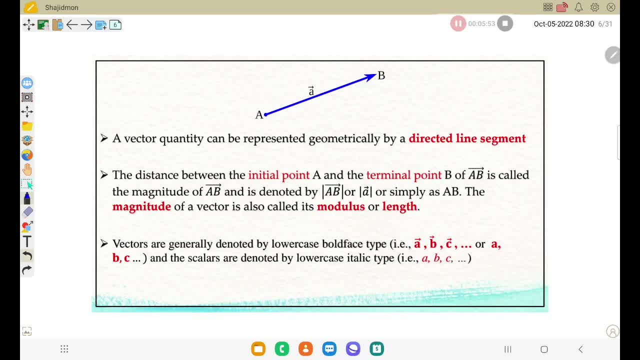 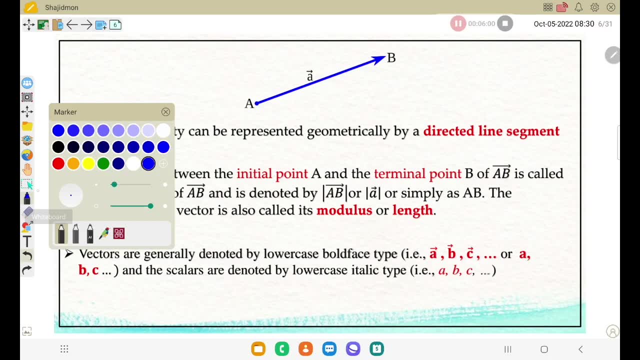 just a brief. I am giving the ideas Now how we are representing a vector quantity. okay, How we can represent a vector quantity, Vector quantity always, we are representing by using a directed line segment. That means we have a line segment. this point, A point we are calling initial point of the vector and this B. 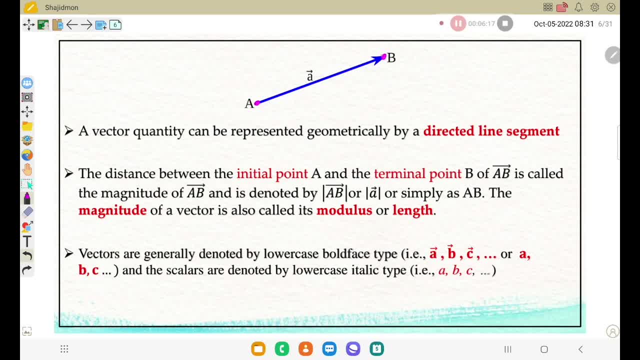 point we are calling the terminal point, initial point or starting point. B means the ending point or terminal point of the vector. Now how we are representing a vector quantity. We are representing a vector quantity. okay, So we are representing a vector. is that? first write the initial point. 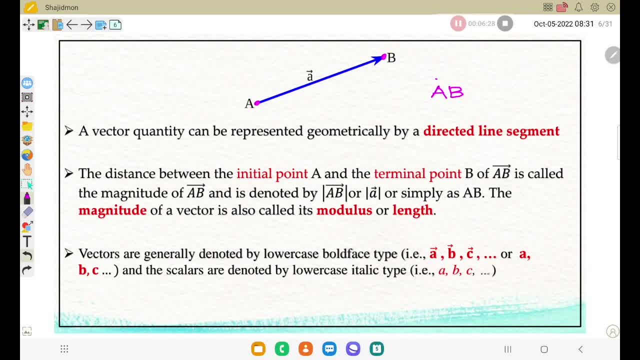 A and write the terminal point B. give a vector notation like this, So we can call it as vector A- B. So always represent by a directed line segment. that means a line segment with direction. okay, So vector A- B. Now, if you are using small letters, we can represent like this: 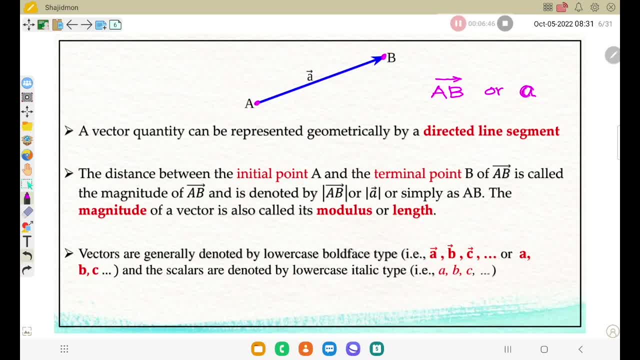 bold letter: okay, bold, bold letter. small letter, vector A. okay, Without initial and terminal point. you can represent like this: okay, So we are representing a vector quantity. okay, So we are representing like this, small letter, but bold font, with the vector notation: vector A. You can. 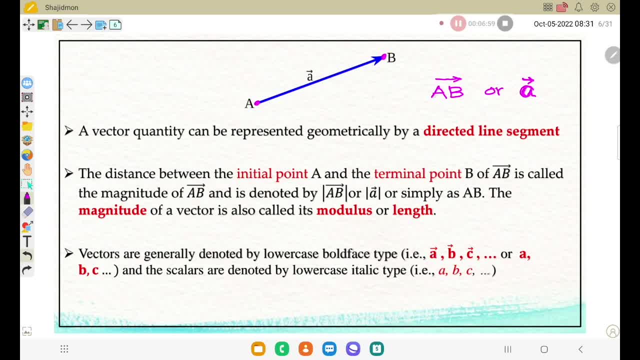 see this line, we are represented vector A. So either we can represent by initial point and terminal point, like this: vector A- B, or small letter, vector A, with the bold font. Now, what is the meaning of magnitude or modulus or length? okay, Length of a vector. Length of a vector means: 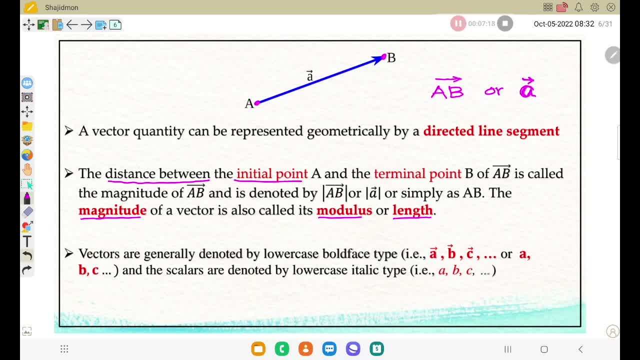 the distance between the initial point and terminal point. that means from A to B. how much distance is there? okay, How much distance is there from A to B? This is what we are calling the magnitude or length of the vector quantity, okay, Length, or we can say magnitude, or we can. 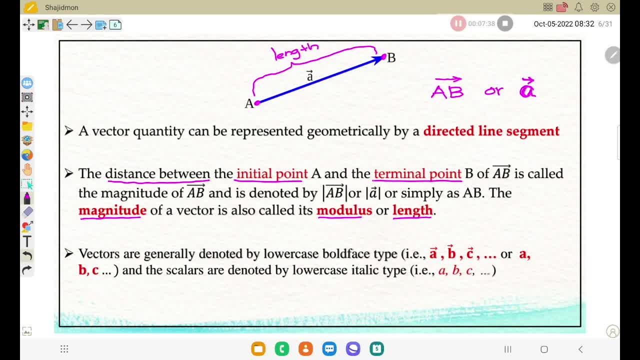 say modulus of that vector. I hope you understood that one And magnitude of a vector. always we are representing, using the absolute symbol, magnitude of vector A- B. like this, magnitude of vector A- B. Otherwise, if you are using the small letter, vector A. 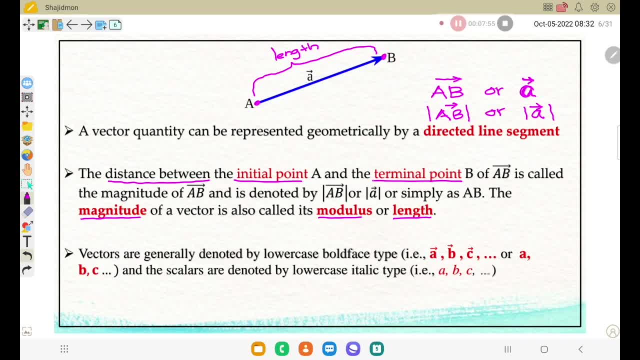 we can use like this magnitude of vector A. okay, So magnitude we are representing by using the absolute symbol. I hope you understood that one. Now we are coming to the third point. Vectors are generally denoted by lowercase. that means small letter, bold face type. 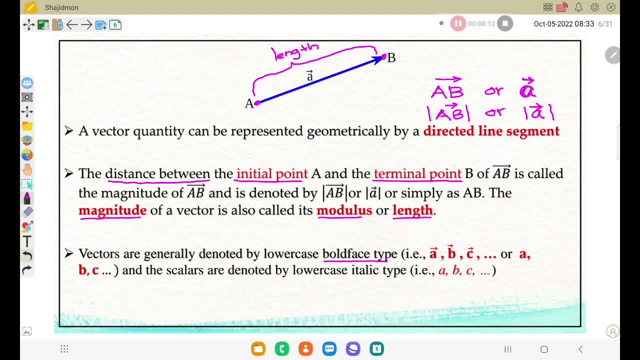 bold letters like vector A, vector B, vector C, vector U, vector V, like that, okay. Or we can say bold letter A, B, C, like this, without vector notation also bold letter, bold font. you can use A, B, C like that, But scalars we are denoted by italic type small letter A, B, C without bold. 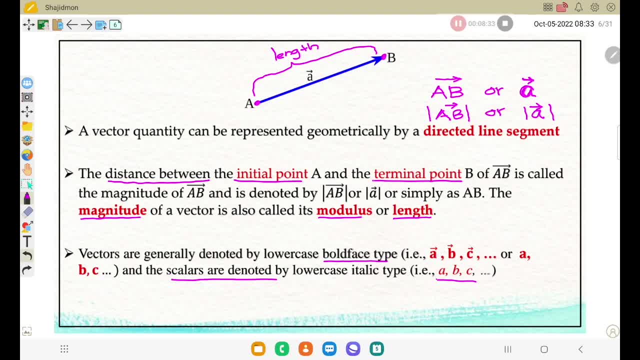 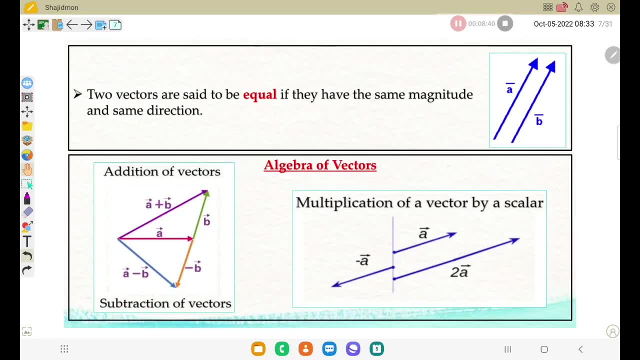 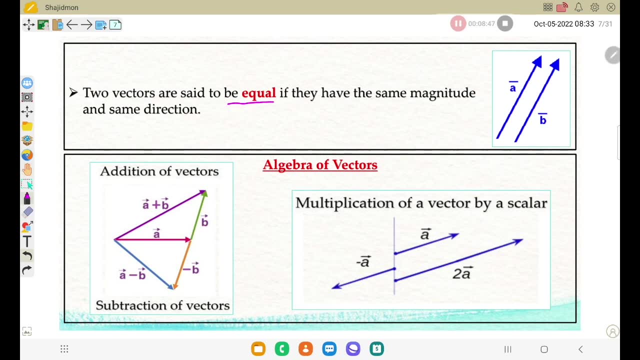 okay, Like this we can represent. So this is the representation of a vector. Now we will come to the next point, When we are telling two vectors are equal, when we are telling two vectors are equal vectors. Now, two vectors are said to be equal. okay, Equal That, both vectors having. 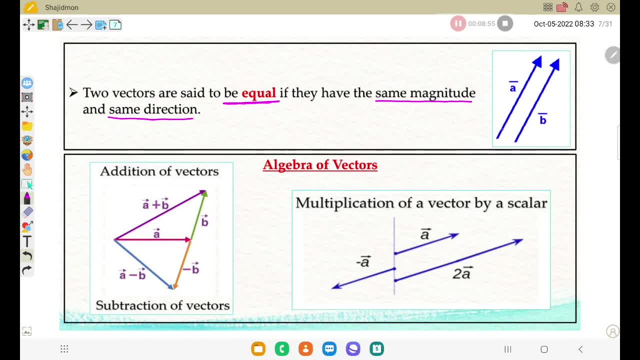 magnitude and same direction. That means we, for example. this is the first vector, vector A, starting point. this is the ending point. Now, this is the second vector, starting point, ending point. Both vectors should have same magnitude. that means: from here to here, distance from here. 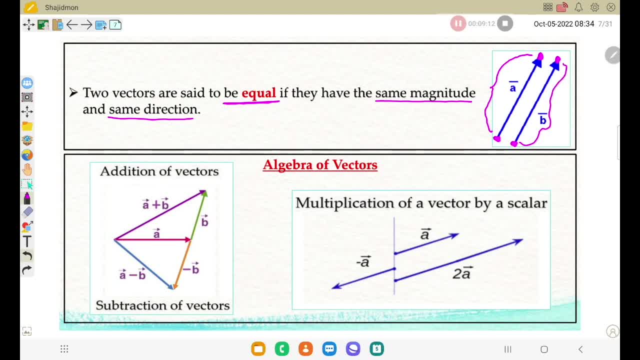 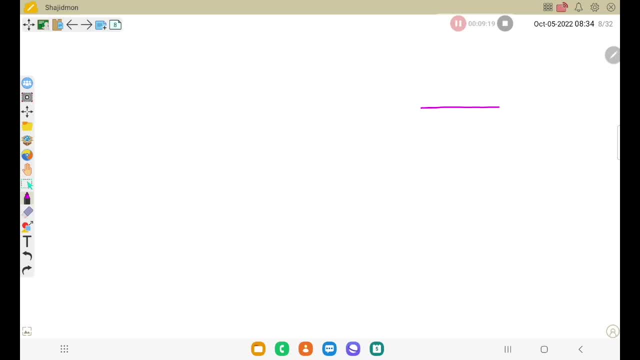 to here, distance. both should be same and same direction also. okay, Same direction also. that type of vectors we are calling equal vectors. I hope you understood okay. For example, one vector, vector A, okay- And another vector like this, vector B. See, both are having same magnitude. 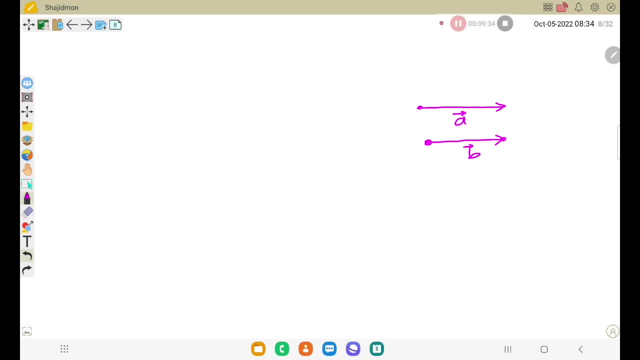 same direction, So we can say: equal vector. Now, for example, vector A is this one. How we are writing: minus vector A. Minus vector A means the vector takes same magnitude, but opposite direction. For example, see starting from here, ending at here. okay, Now see what is minus vector A Minus. 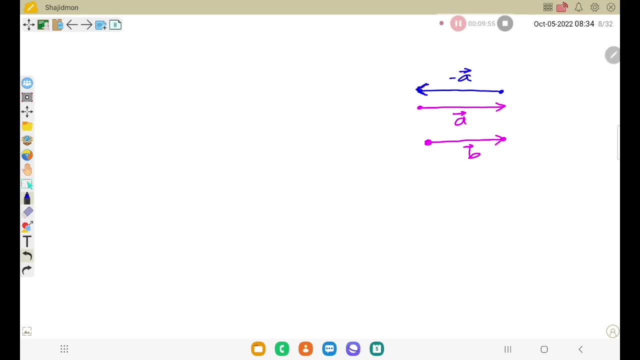 vector A. That means vector A take in opposite direction. This is the meaning. minus vector A: okay, Same magnitude, but direction is opposite. Now, minus vector B: see like this: B direction, just to reverse that one. That is what we are calling. minus vector B: okay, Opposite direction. 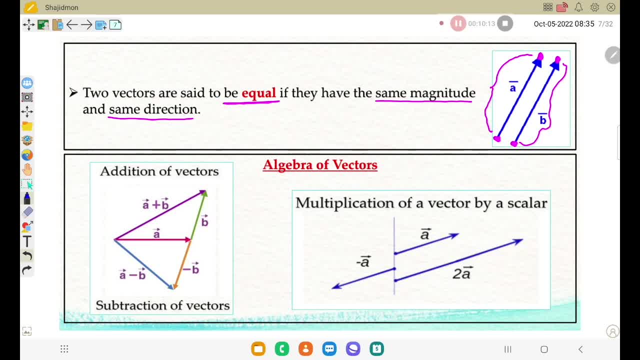 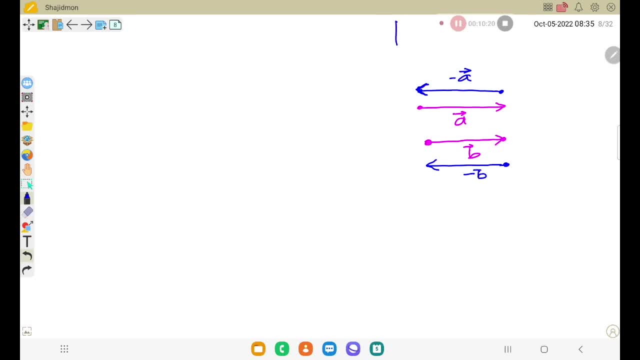 Now we will come to the next point. What is the meaning? Addition of vector and subtraction of vector and multiplication of a vector by a number, For example. see here I can tell you small examples. For example, I have a vector, vector A, like this, okay, And I have a. 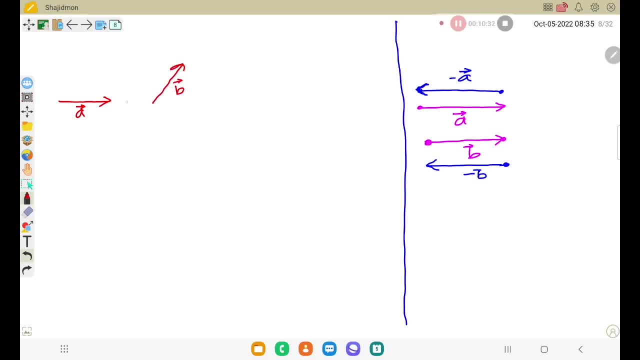 vector, vector B. like this: I want to add these two vectors, vector A plus vector B. How can we do vector A plus vector B? So what you do is see this is vector A, Same vector I am drawing. 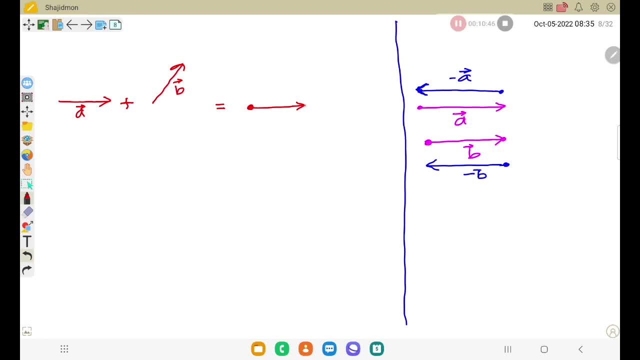 again. So this is the initial point of the vector. This is the terminal point. Now, second vector, B vector, we are shifting. We are shifting to the terminal point of this B, the A vector. terminal point of the A vector. 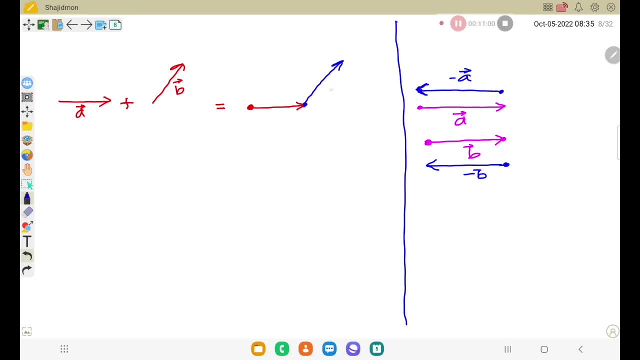 like this Same vector. we are copy paste here. So this is vector B, correct? And already I told this is vector A. Now how to add these two vector? Just start from the initial point here and terminal point here, Just to draw a line joining these two. point This vector we are. 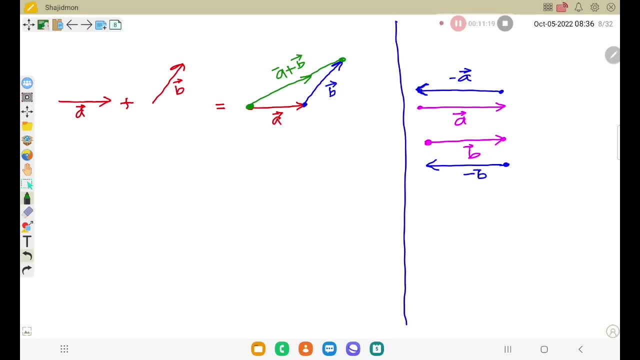 calling geometrically A plus B vector. So how to add two vectors geometrically? You can see the starting point here, initial point and terminal point: joining a vector, That is the A plus B vector. I hope you understood Now when we are going to subtraction of vector A minus B vector. 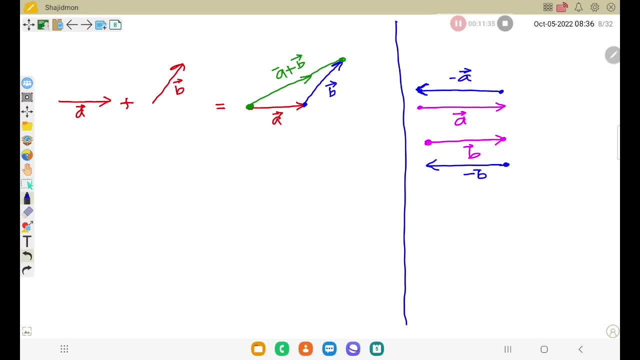 okay, So A is same. Now minus B means, as I told, B vector just take in the reverse direction, correct? That is minus of vector B, correct Now what I am doing? see A vector here, same. 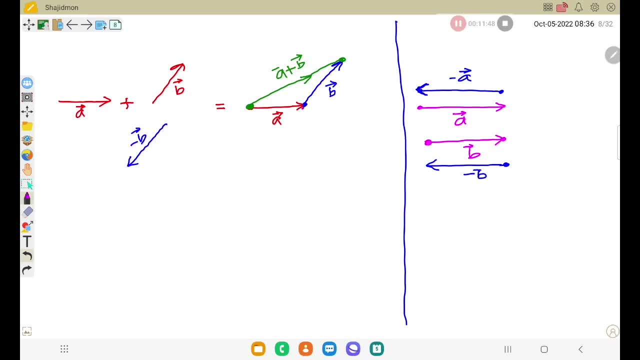 Now I am just drawing what is minus B vector here. That means B vector, draw in the opposite direction. That is minus vector B, correct, Minus vector B here. I hope you understood Now what we do just here, from starting point up to the ending point. we are just 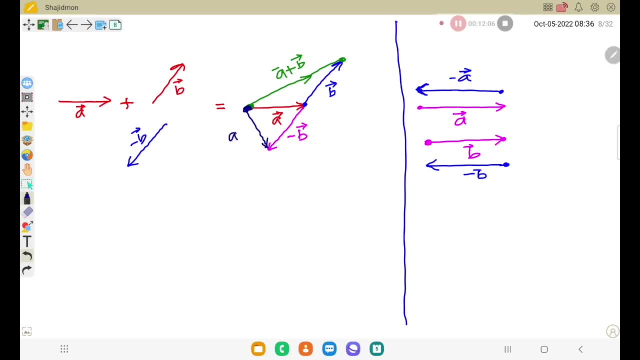 drawing a line, a directed line. That is the vector A minus vector B here. So I hope you understood how we are adding two vectors geometrically, How to subtract two vectors geometrically correct. Now we are going to discuss 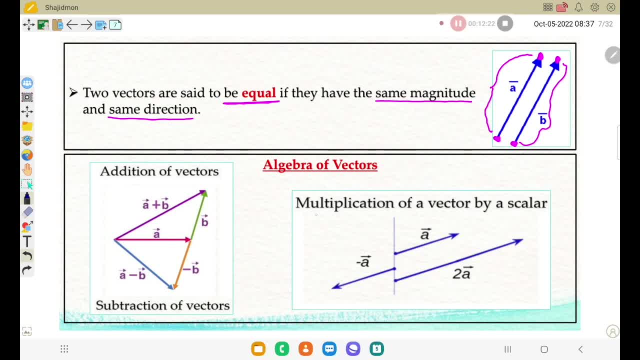 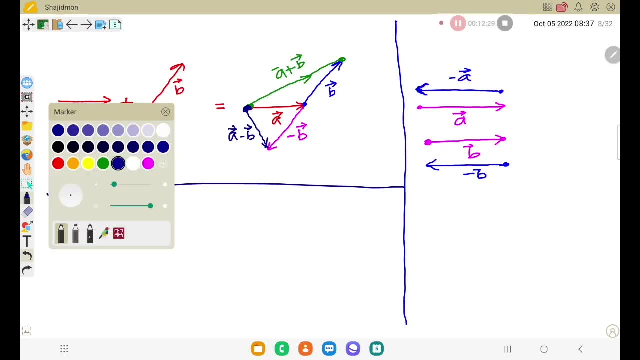 So equal vector, discussed addition, subtraction. Now multiplication of a vector by a scalar, by a number. Scalar means a number, For example. okay, I have a vector, vector A here. This is vector A. Now what is the meaning of two times vector A? See a number. multiply a vector A. 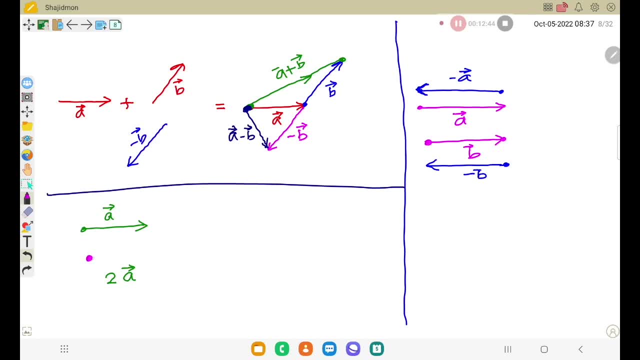 number multiply a vector. So what you do, Take this vector two times, like this: okay, One time here, one time here. So you have two vectors here. So you have two vectors here, So you have. so this is the vector 2 times vector a. okay, i hope you understood now. same way, minus 2 time vector a. 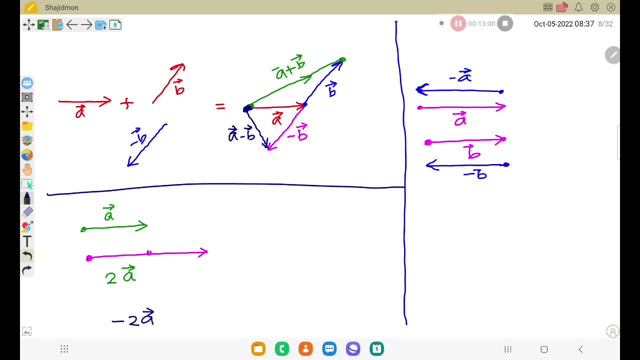 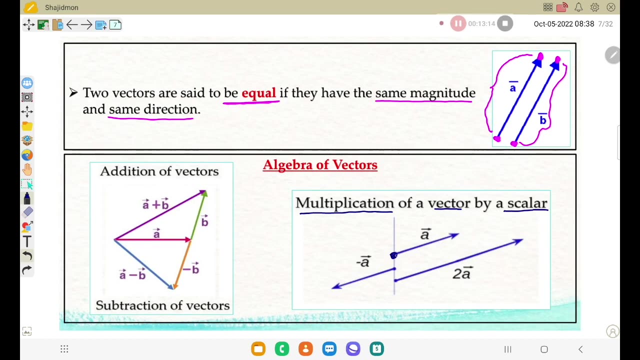 if you want minus 2 times vector a, how we do the same vector in the reverse direction, starting here, correct? this is minus 2 time vector a. like that we can multiply a vector with any number. you can form that one. see this picture. this is vector a. you can see this is starting, ending here now. if 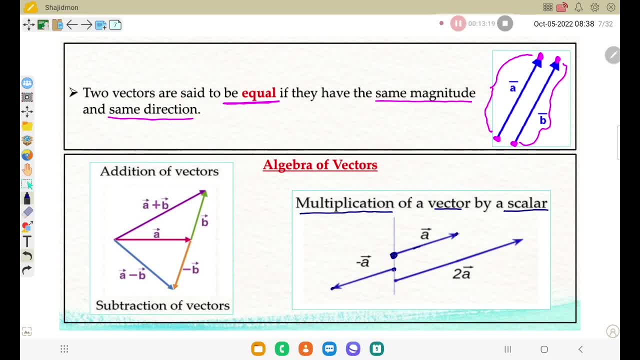 you want minus vector a, taking the reverse direction, correct. same magnitude 2 times vector a means 2 times we are taking vector a. so this is the geometrical idea behind multiplication of a vector by a scalar, by a number. i hope you understood. now we are going to the practical. 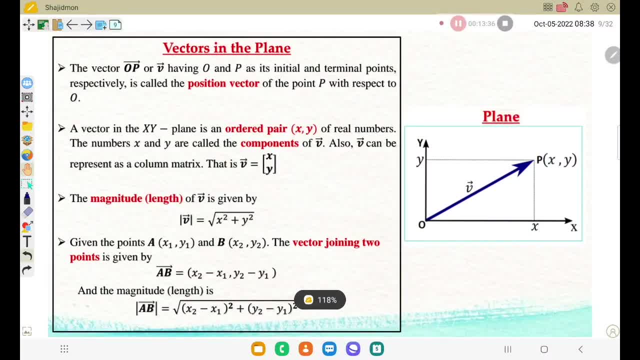 questions. okay, now see, we discuss how to represent a vector in plane. how to represent a vector in plane. how can we write a vector in plane and after that we need to study how to write a vector in space. correct now. plane means what is the meaning plane? plane means it is two. 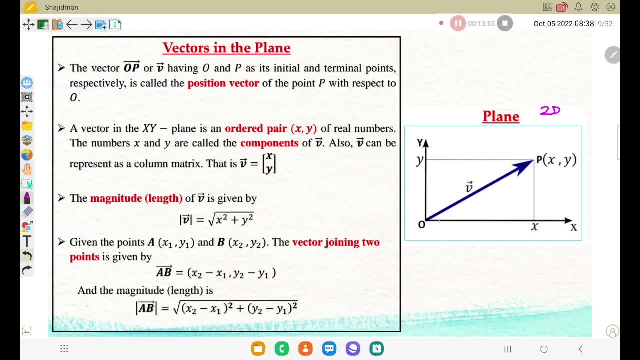 dimension, correct, two dimension. two dimension means we have x axis and we have y axis, x y plane. we are telling it as x y plane or two dimension. okay, now see, in the x y plane, you know this point. this point is center, origin, zero o point. o means zero, comma zero, correct. now, if i am taking a point, 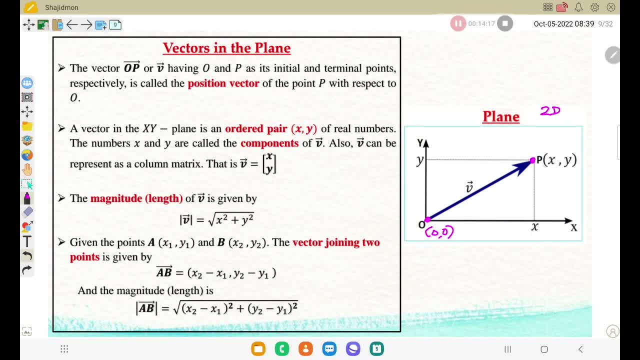 here. this point is p, p, x, y, because in plane when we are taking a point it is like x number will be there, y number will be there like ordered pair. pair. we are telling two number. pair means two number: x, y. ordered pair means should have an order. first number for x, x number. second number is y. 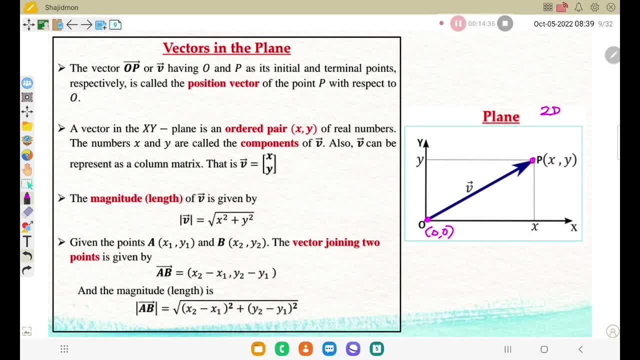 number. so this is zero point, o point or this is p point. now, if you are joining a, if you are drawing a line, okay, starting from o up to p. okay, this is the vector. you can see one vector i drawn here. okay, starting from zero. keep in our mind: starting from zero up to p, that means initial point is o, final point is p, vector op. this. 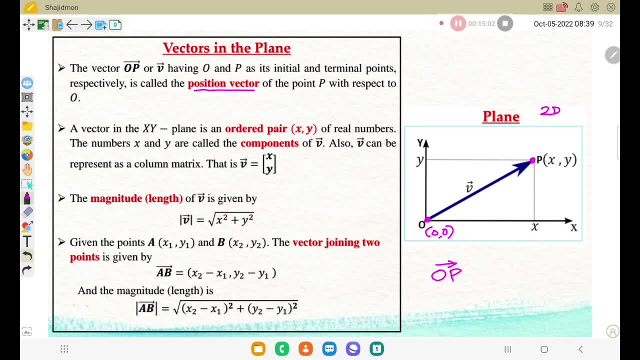 vector. we are calling a special name, that is, we are calling position vector of the point p, position vector of the point p with respect to the origin o. okay, but that means what is the position vector? position vector means vector starting from the origin center: zero, zero point. okay. so vector op, vector op is the position vector of the point. 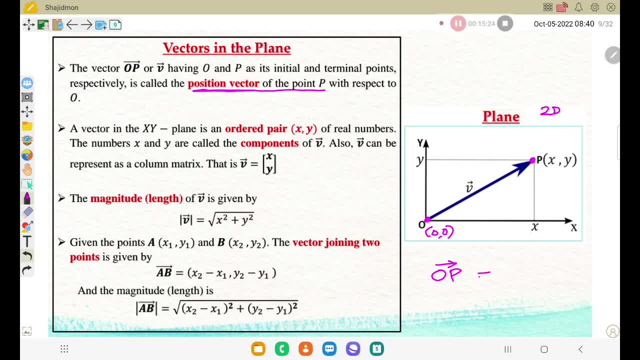 p with respect to the origin, and this vector we can represent as a ordered pair in component form, like this: first, x number and y number. okay, vector op means just mark this point. see x and y. x means we are calling x component, y we are calling y component. this is the component form of a. 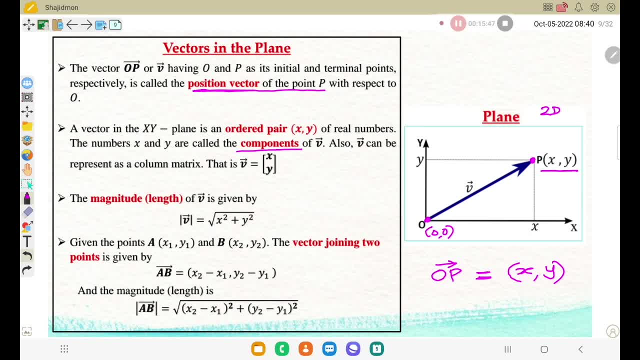 vector. vector o, p. okay, so this is ordered pair. x, y means it is ordered pair. ordered pair means x, first number, y is the second number, first component, second component, x component, y component. ordered means should have one order: x should be first, y should be second pair pair. 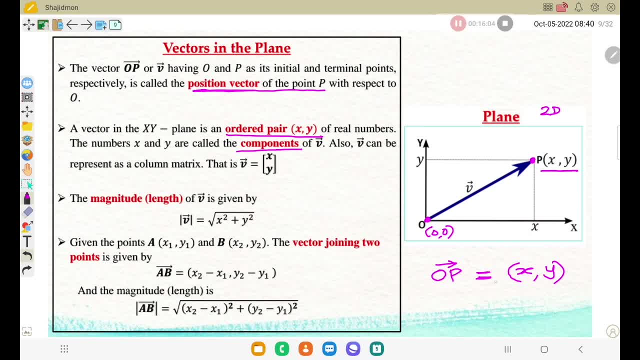 means two number. now this vector op we can represent like this ordered pair: x, y. other ways we can represent by matrix, like this: x, y, just represent like a column matrix. column matrix x, y, andまた we can turn it into a Fang y. okay, so this is the position vector of the point p with respect to the origin: o okay vector. 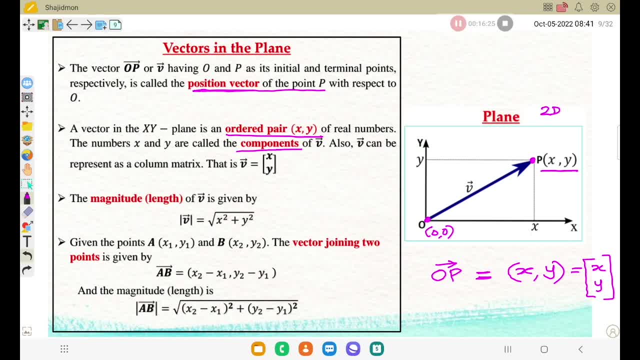 o p. so position vector means always keep in your mind, starting with o, point now zero, point now magnitude or length of a vector. how can we calculate the distance from zero to p? okay, magnitude of that vector, o p, we can calculate by using the rule: this: one: root of x, square plus y. 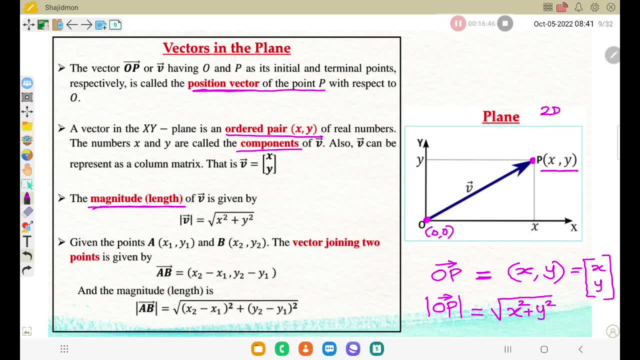 square. that means this vector x component square plus y component square, root of x square plus y square. this is the magnitude of the vector. vector o- p. position: vector vector o- p. i hope you understood. this is the second rule here. now we will come to the vector joining two points two. 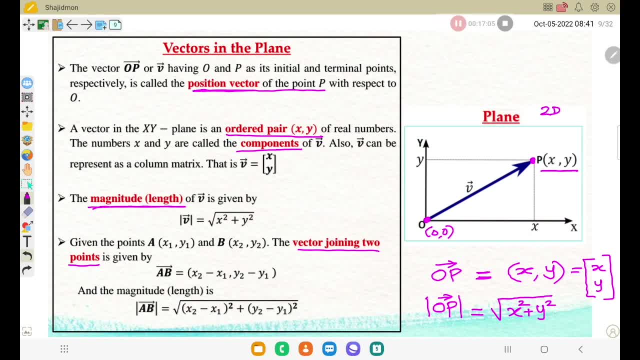 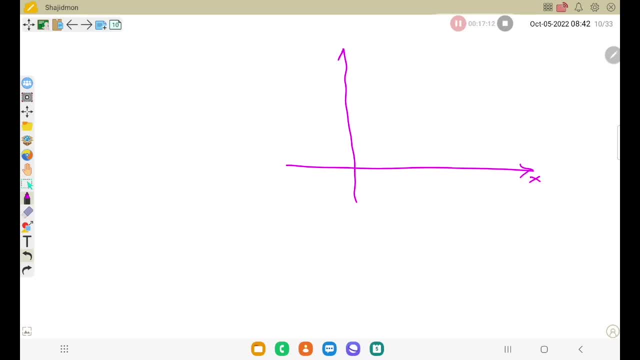 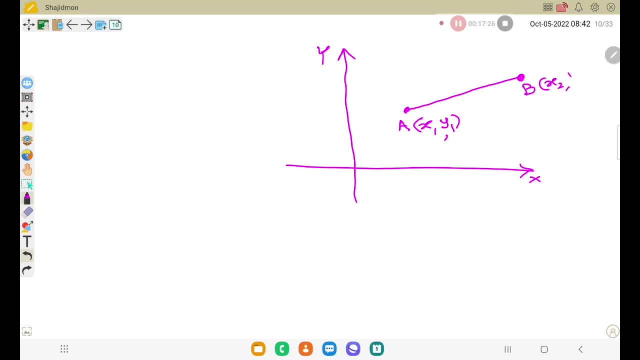 taking second point here, b x, 2 comma, y 2. okay, now the vector joining. see, i am giving the vector notation. it is not starting from the center, correct vector. starting from the center means we are calling it as position vector. now here, it is not starting from the center. vector a, b: 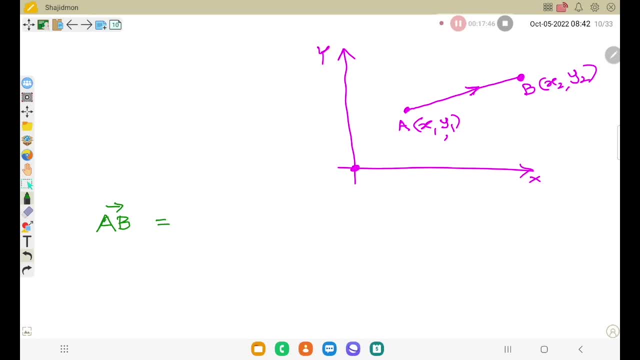 we find the component form of vector a, b equal. that means vector joining two points. okay, two points. now how we are calculating is ordered pair should be ordered pair because x y plane. correct ordered pair: second: x number minus. first x number x 2 minus x 1 comma. second: y number minus first. 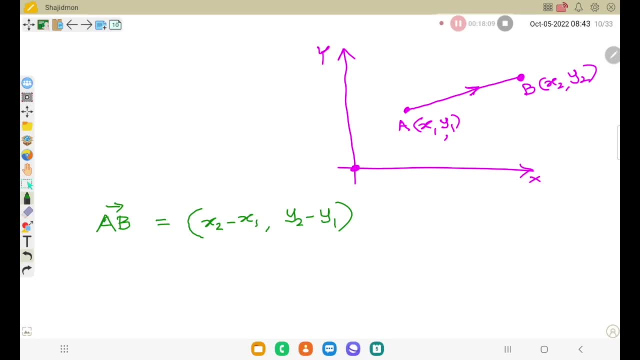 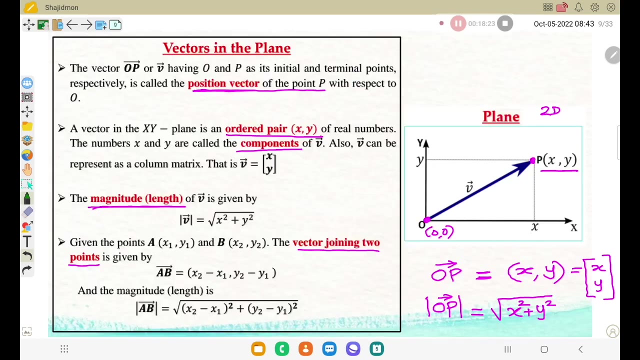 y number. that means y 2 minus y 1. okay, this is the vector joining two points. okay, keep in your mind: vector, point, op vector mean position, vector, vector means only x, y, but if it is two, point means x 2 minus x 1 comma, y 2 minus y 1. so keep in your mind this one, this okay, important rule. given points a, x, 1, x, 2, y, 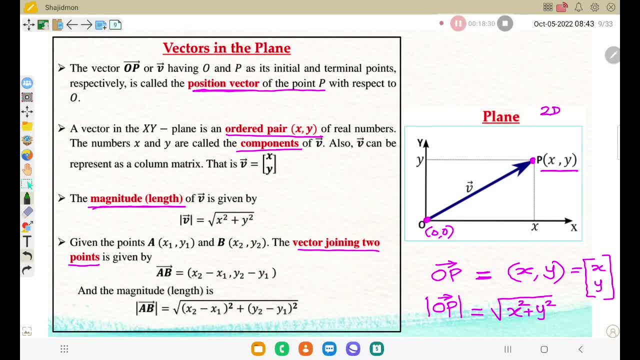 2 vector joining two point means vector a, b equal to, equal to x 2 minus x 1. comma: y 2 minus y 1 and this magnitude means same. what rule we are studied here? root of x square plus y square. here x number is x 2 minus x 1, y number is y 2 minus y 1, so x 2 minus x 1 square plus y. 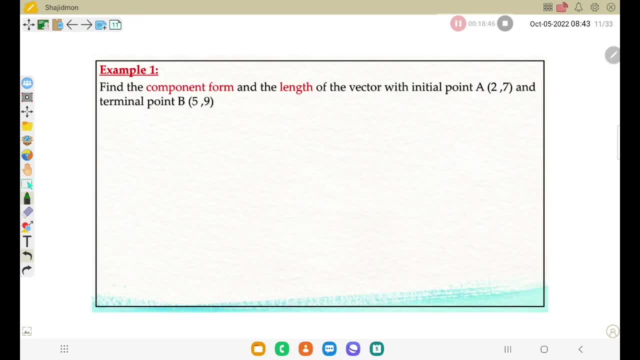 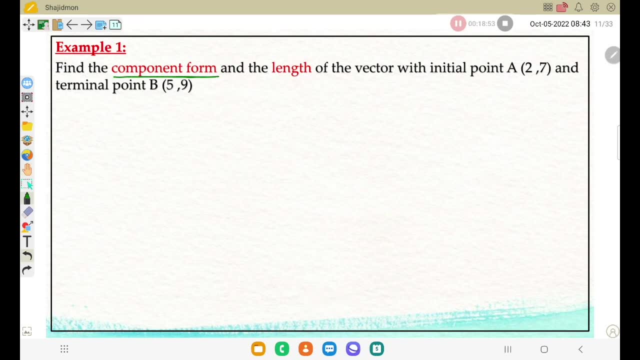 2 minus y, 1, square. now we will do one question, one example here. more question we will do in exercise. okay, find the component form. what is the meaning component form? component form means we need to calculate x component and y component, x, y correct and length of the vector with the. 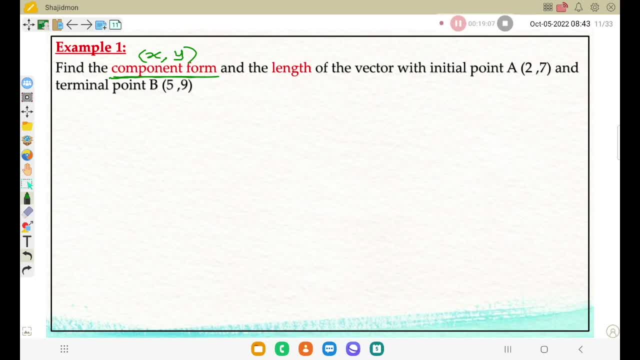 initial point a, 2, 7 and terminal point b, 5, 9. okay, this is the first question. so a vector starting with a, 2 comma 7 and terminal point, ending point of the vector is 5 comma 9. the point is b correct. what is the vector? what is vector a, b in component form? that 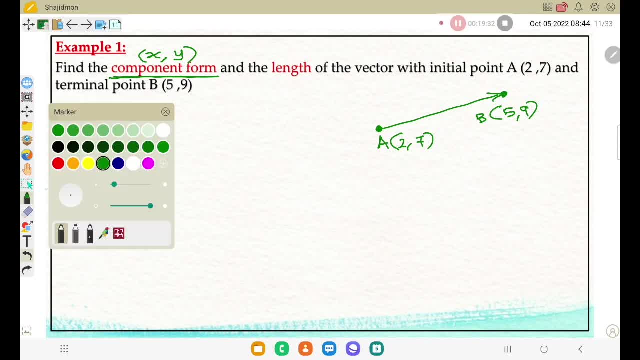 is the question. vector a, b in component form. you remember we are studied just before, okay, for example- this is the first point- x 1, y 1. this is x 2 and y 2. now what we are studied. vector a, b in component form: x 2 minus x 1 comma, y 2 minus y 1: apply the number. what is the x 2 number? the 5 minus. 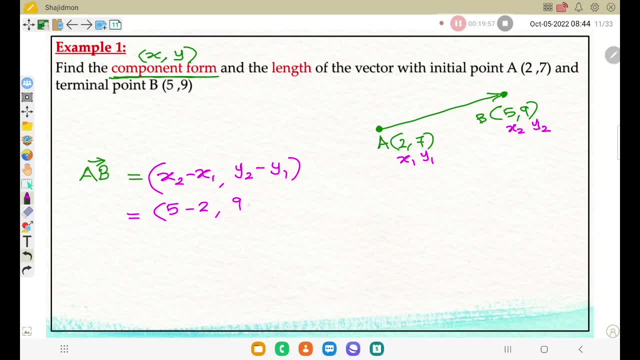 what is x 1, 2 and y 2 number? 9 minus y 1 number is 7, so you can get it. the answer equal to ordered pair should be ordered pair: 5 minus okay, 5 minus 2. that means 3. 9 minus 7 means it is 2, 3, 2. this is: 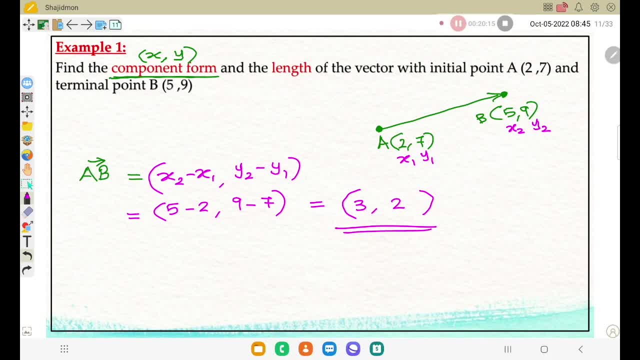 the vector component form: x 2 minus x 1 comma, y 2 minus y 1, apply the number. what is the x 2 number, x component and y component. okay, the first number is x component, x value and second is y component. that is y value. now what is the next question? find the length of the vector. length means: 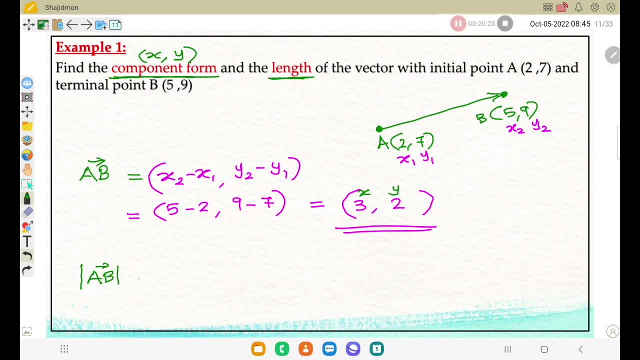 magnitude of vector a- b. absolute of vector a- b, equal. what was the rule root of x power 2 plus y power 2, correct, now, equal to root of what is x x component. we calculated here what is the x, what is the y component? 2. so 3 power 2 plus 2 power 2. so that you will get from the calculator. 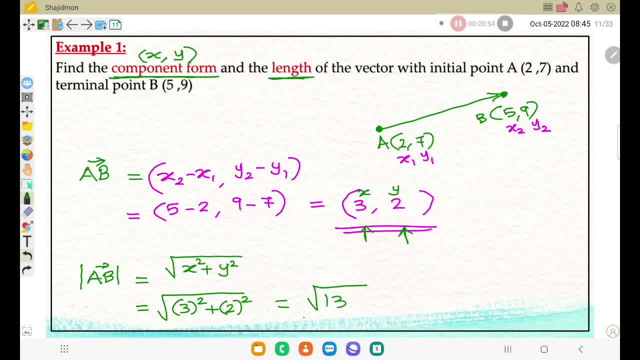 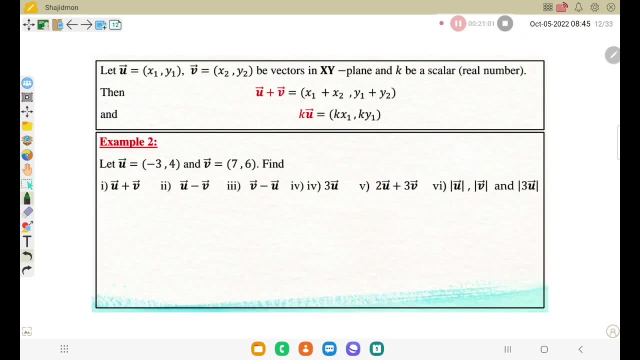 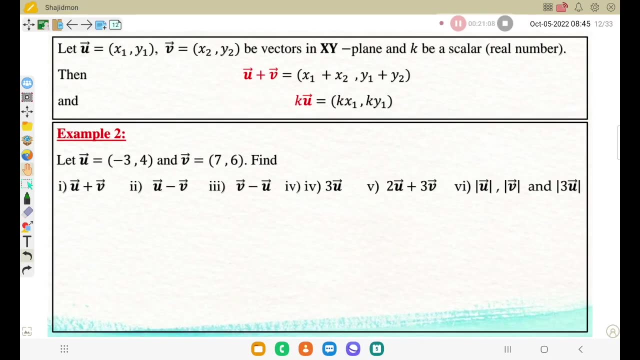 it is equal to root of 9 plus 4, that is root 13. this is the magnitude of that vector. i hope you understood that one. okay, now we are going to discuss about how to add two vectors, how to subtract, how to multiply two vectors. okay, for example, you can see the rule: first, let u equal. 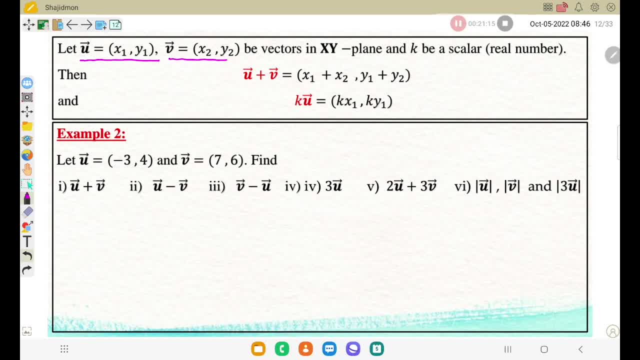 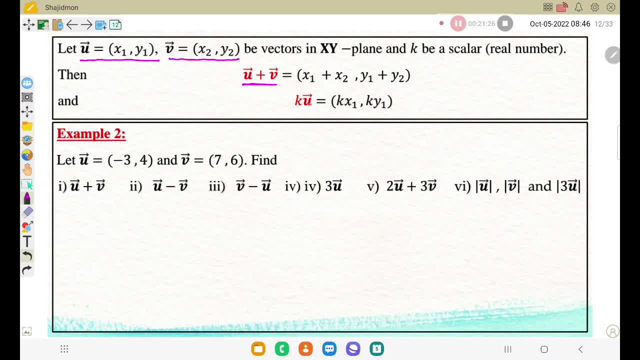 x 2 comma, y 1 plus y 2 and k multiply vector u. that means a number multiply a vector means number multiply each numbers in the ordered pair: k multiply x 1 comma. k multiply y 1. okay, k x number k. x 1 k comma. k y number, k, y 1. adding means x 1 plus x 2 and y 1 plus x 1 comma. y 1 plus x 1 and y 1. 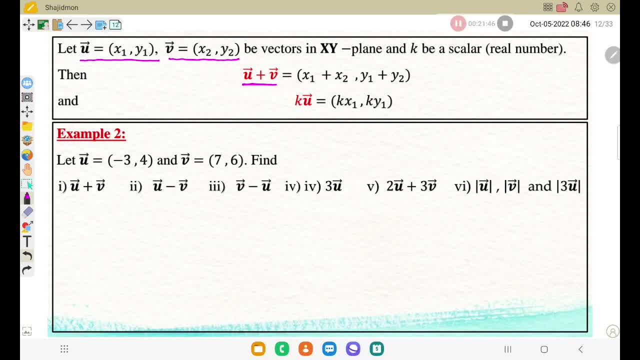 x numbers add plus y numbers add. so this is the easier way. geometrical definition. we studied what is the meaning of addition of vector, subtraction of the vector. this is the practical example when we are getting two vectors in component form: how to add two vectors and how to multiply the vector. 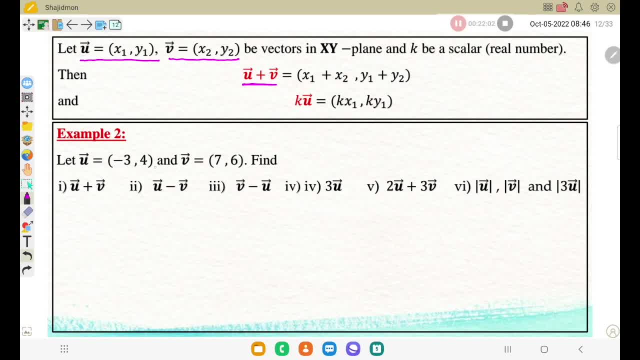 for example see: vector u equal to minus 3 comma 4, vector v equal to 7 comma 6. okay, find u plus v first part. okay, find vector u plus vector v. here vector u means minus 3 comma 4, plus vector v means 7 comma 6. correct now how to add as i told. 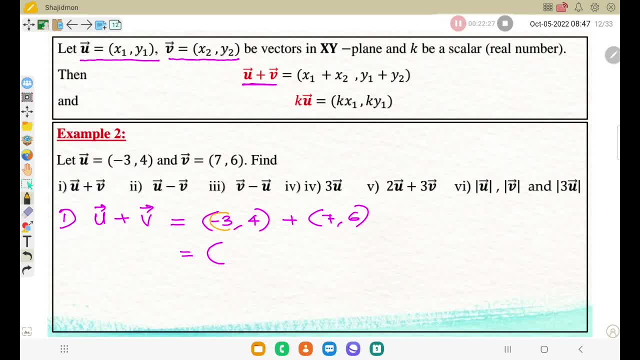 x numbers add. what are the x here minus 3, here 7, correct. so minus 3 plus 7, minus 3 plus 7 comma. what are the y number here? 4 and 6, so 4 plus 6, so that you will get the. 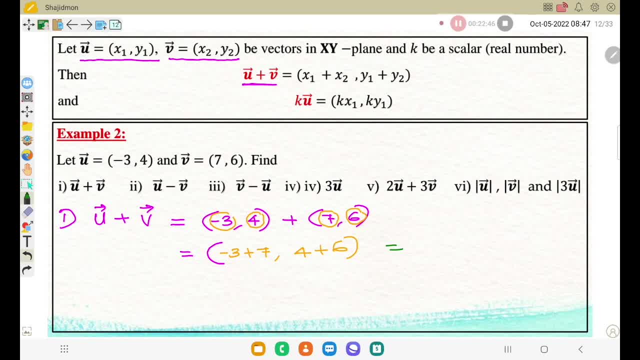 answer: equal to minus. 3 plus 7 means 4, 4 plus 6 means 10. so this is the u plus v vector. now the second part: u minus v vector vector. u minus vector v. equal to same. we are subtracting u vector means. 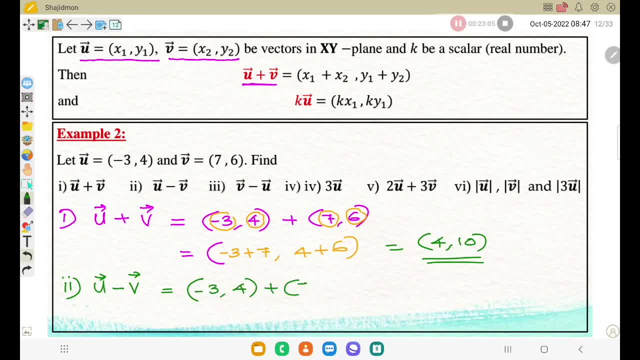 minus 3 comma 4 plus v vector means 7 comma 6. so when we are subtracting what value we got minus 3 minus 7, correct comma 4 minus 6: x number subtract, y number subtract. so we will get minus 3 minus 7 means. 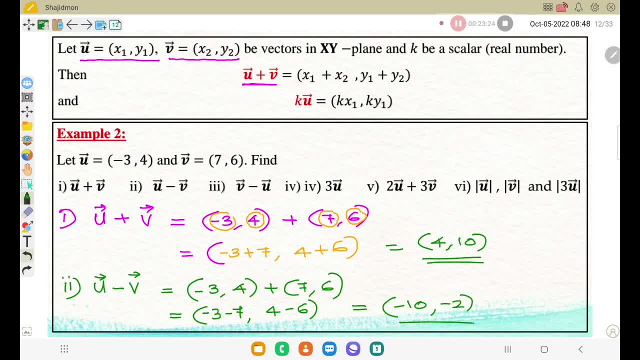 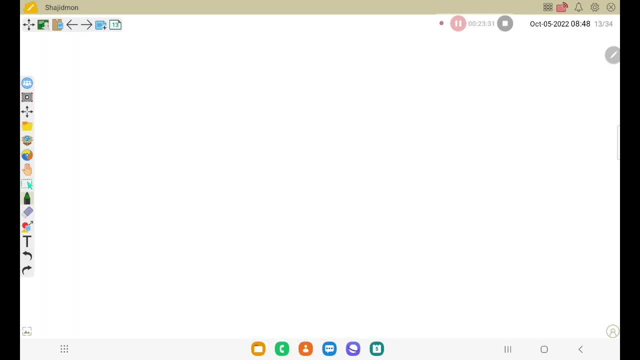 minus 10. 4 minus 6 means minus 2, so this is the u minus v vector. now we can do what is v minus u 3. multiply u all this part first. we will do third part. that means 3 times vector u equal to sorry. 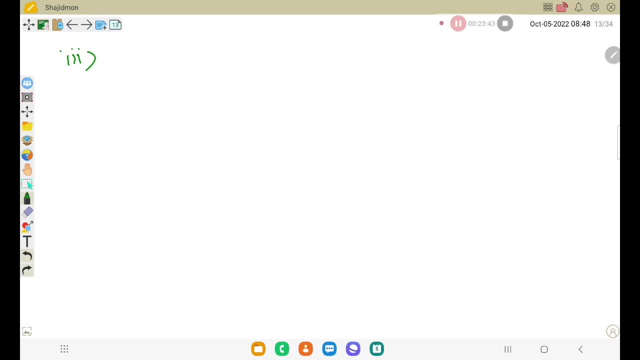 before that we need to do v minus u, third part. vector v minus vector u, equal to what is vector v 7 comma 6 minus what is vector u minus 3 comma 4. subtraction time: very careful, you will get equal to 7 minus minus 3. 7 plus 3, that is 10. 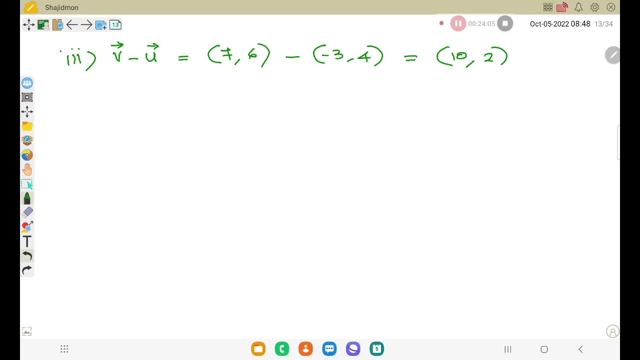 6 minus 4. that means 2 subtraction. correct now the fourth part of the question. what is the fourth part? 3 times vector u equals. that means 3 times what is vector u minus 3 comma 4. correct now how we are multiplying this one, just. 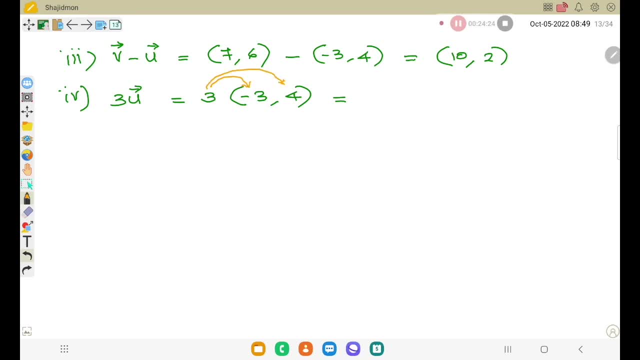 multiply with the first number comma, multiply with the second number, so we will get 3 multiply minus 3 means minus 9. 3 multiply 4 means 12. correct now okay, fifth part of the question. 2 times vector u plus 3 times vector v equal to that means 2 times vector u plus 3 times vector v equal to that means. 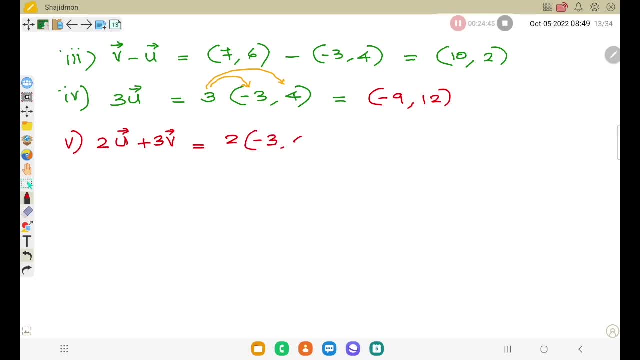 2 times what is u minus 3, comma 4, plus 3 times what is vector v, 7, comma 6.. Now you can multiply: that means vector 2 times minus 3 minus 6, 2 times 4, 8 plus 3 times 7, 21 plus- sorry- comma 3. 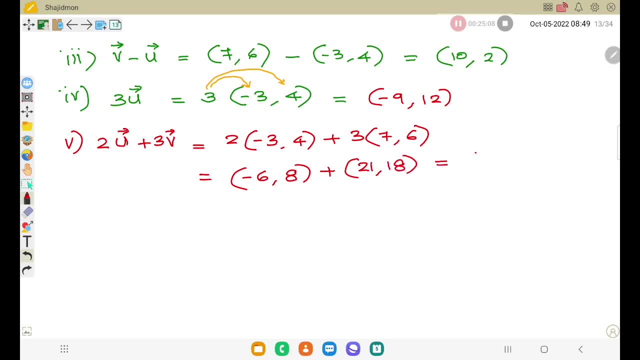 multiply 6 means 18.. So, adding time, you will get 15 comma 26, because minus 6 plus 21, 15 and 8 plus 18, 26.. Now we will go to the sixth part of the question. We need to calculate what. 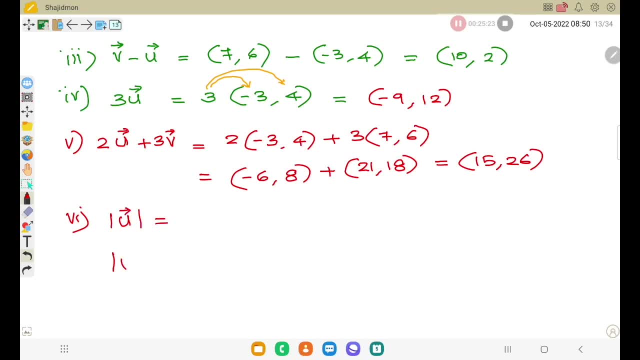 is absolute u vector and magnitude of vector v and magnitude of vector 3 u. These are the question in sixth part. So first we will do what is magnitude of vector u? What is the rule we are studying? magnitude root of x power 2 plus y power 2.. So root of 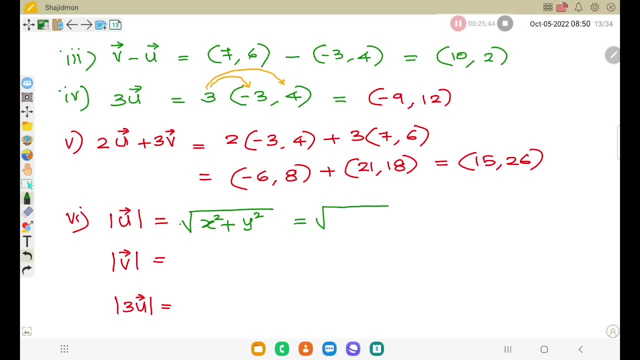 you can see u vector. u vector means minus 3 comma 4.. So x number is minus 3 power 2 plus y number is 4 power 2, correct. So you will get equal to 5 from the calculator. 9 plus 16. root means root: 25. 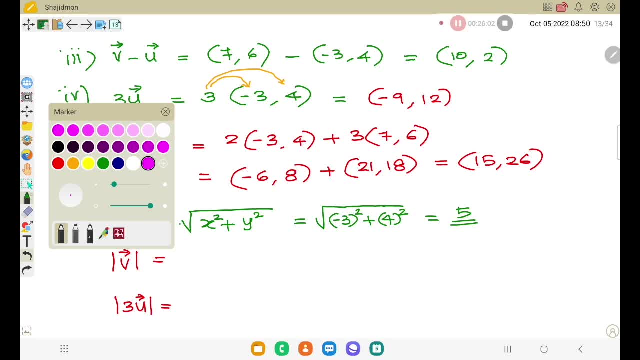 is 5.. Same way we can do magnitude of vector v. that means root of x square plus y square V vector means 7 and 6.. So 7 power 2 plus 6, power 2. So we will get equal to 7. power 2 means 49, 6 power 2 means 36.. So totally, we will get root of 85.. Hope you. 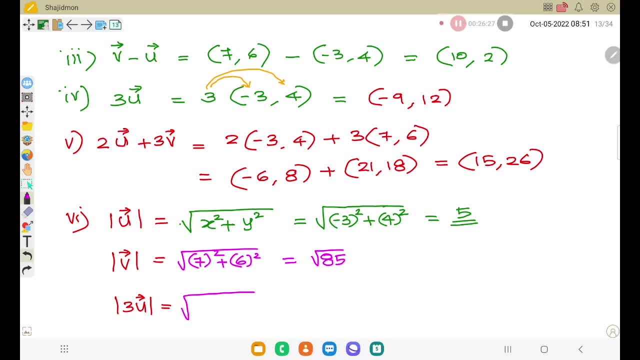 understood Now magnitude of 3 times vector u, root of 3 times vector u. we are calculated here: What is 3 times vector u minus 9 and 12.. So x number is minus 9 power 2 plus 12 power 2.. Y number is 12. 12 power 2. That means we will. 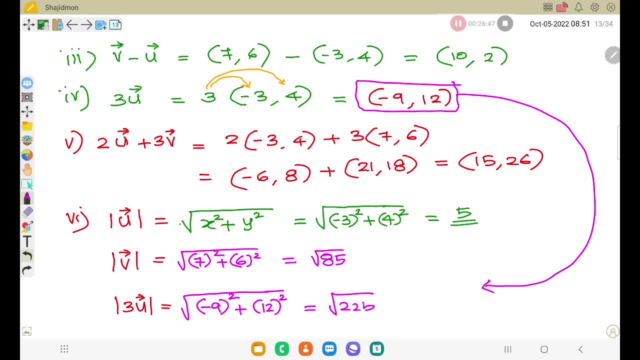 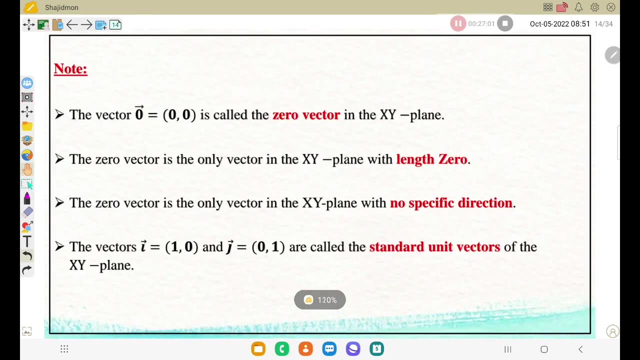 get root 2 to 5 or equal to 15 from the calculator. Okay, Equal to 15.. So this is the magnitude of 3 times vector u. I hope you understood this question. Now we will discuss some small points here, Small nodes. Now you know in x, y plane what is the. 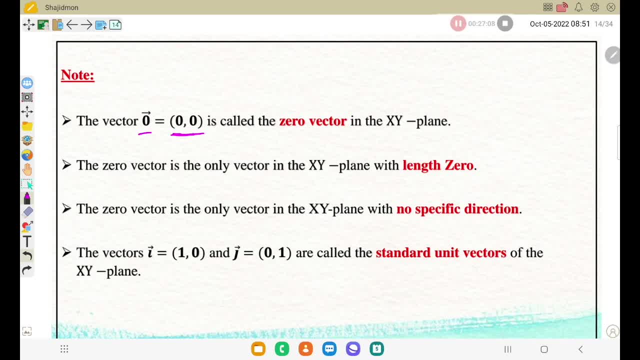 vector. I told 0: 0. correct This point. we are calling 0 vector, 0 vector. notation: 0 vector. That is calling 0 vector in the plane x, y plane. Okay, Now the 0 vector, always. the length will be. 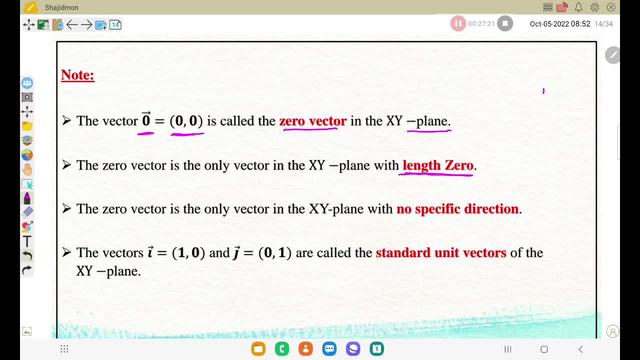 0.. Okay, The 0 vector means nothing. One point correct In x y plane. this is the 0 point. O point 0 comma 0, correct. So distance is 0.. Length is 0.. And 0 vector is the only vector in the x y plane. 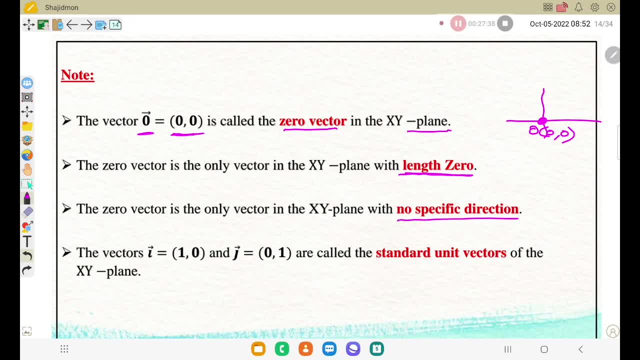 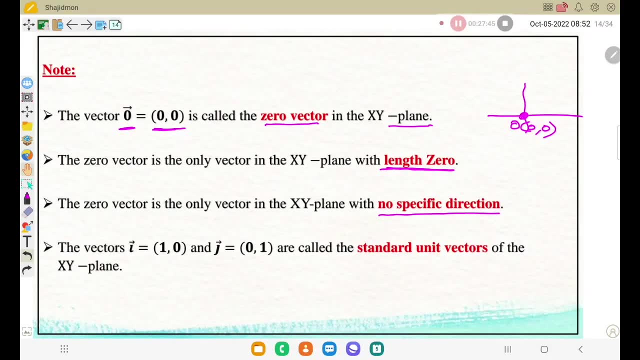 Specific direction, because single point, Any direction, correct Specific direction. no Specific direction, It is 0 vector. Now another important point: we need to be standard unit vector. This is very important, Standard unit vector. Standard unit vector means, for example, you can see x axis. 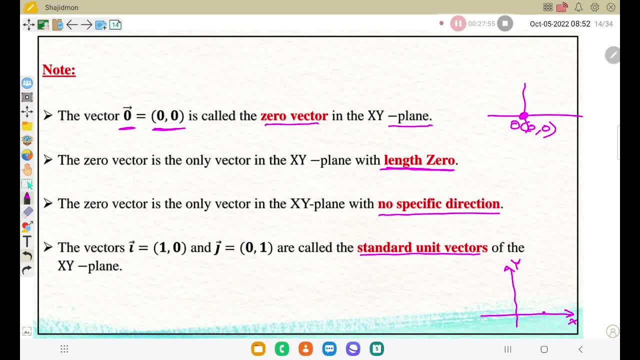 and y axis. Okay, Now x axis, if I am taking a point 1.. Y axis: also take the point 1.. Okay Now, what is this? 1 actually? x? 1 means 1 y, 0.. Audit pair: 1- 0.. So this vector we are calling a special name, Vector i, Standard vector. 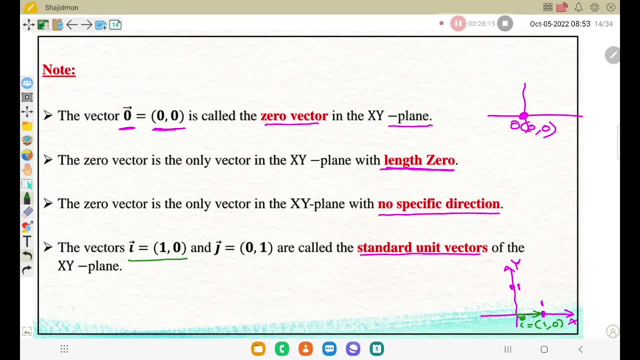 i equal to 1, 0.. See vector i equal to 1 comma 0.. Now same y axis When we are taking a point 1.. What is that? point x, 0, y, 1. Correct, So that vector starting from center, Correct, Origin. 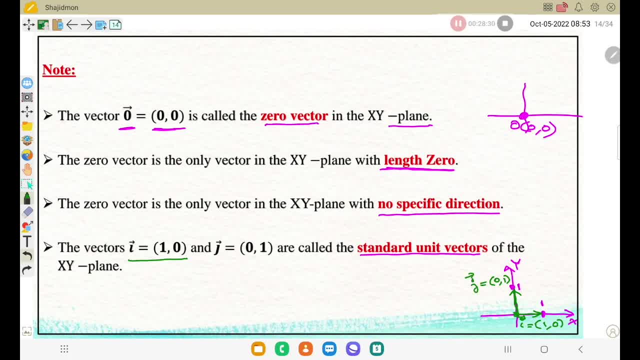 That vector we are calling a name, vector j. Okay, Vector j equal to 0, 1.. These are the standard unit vectors in the x y plane: 2 vectors: Okay, Vector i and vector j. So this is very important. 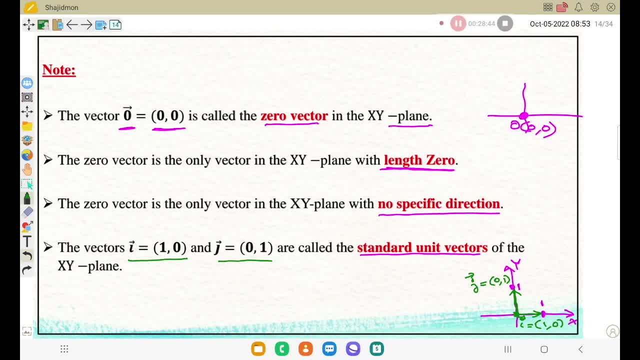 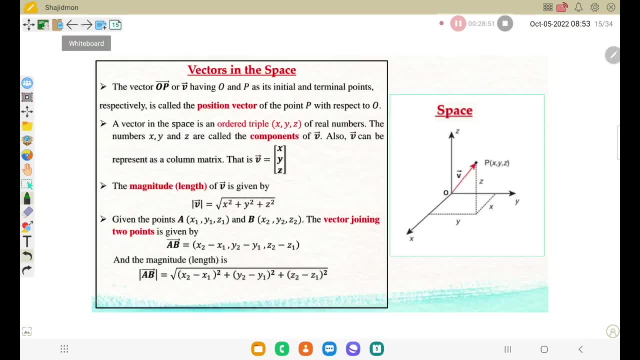 You can just to note: Standard unit vector in the x y plane: Vector i 1: 0.. Vector j: 0: 1.. Hope you understood. Now we will go to in space The same idea we are discussing in space now. Okay, Space. 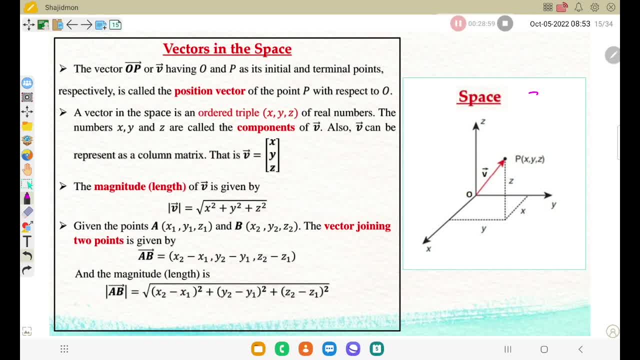 Okay, Space means What is the meaning space 3 dimension, Correct, 3 dimension, That means we can see x axis And here see y axis And here see the z axis, 3 dimension figure. Okay, So if you. 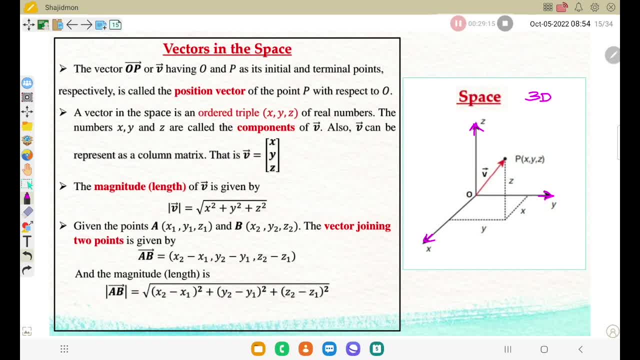 are taking a point in space. How many number will be there? x, y, z, 3 number, Correct, We have x number, y number and z number. x number will be there, y number will be there, z number will be. 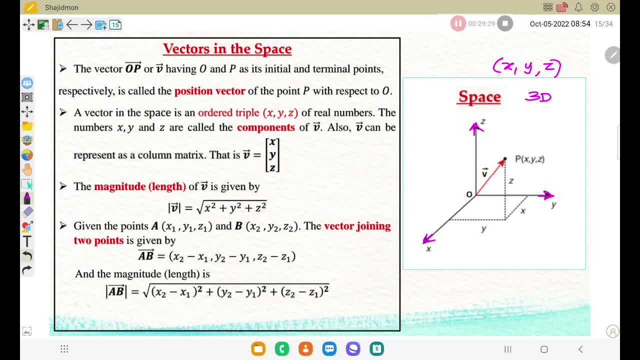 there. Plane means only x, y, Space means x, y and z. Okay, We are calling this as triple Okay. In plane we are. We discuss Pair, But here triple or triad Ordered, triple Ordered, triple Okay. Order should be there x. 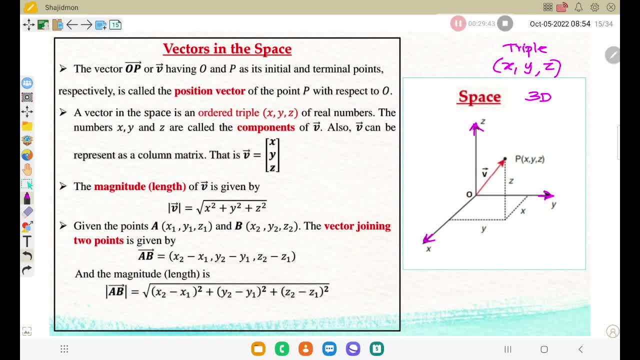 first number, y second number, z third number. Now, when we are taking a point center here, O, O point, O point is what? 0 comma, 0 comma 0. Because x 0.. y 0.. z 0.. Now, if you are taking a, 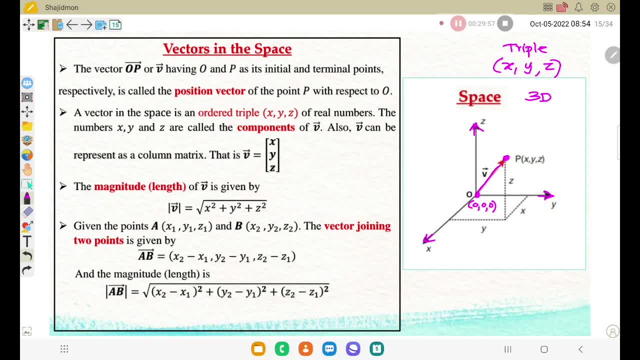 p here, x, y, z, And we just to join a vector like this, Starting from o Up to p. So vector o, p, O is the starting point, p is the terminal point, ending point, this vector we are calling position vector in the space. 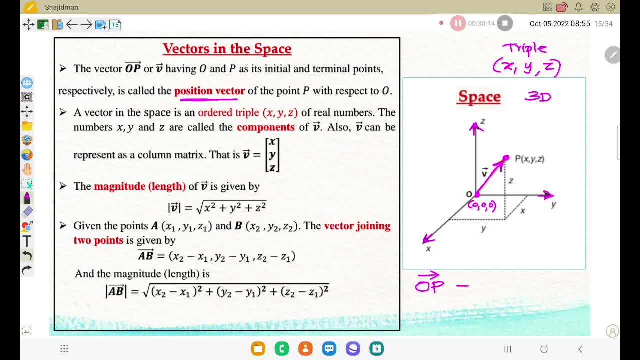 same, like in the plane what we discussed. so vector op equal to how we are representing in component ordered triple three number, how three number x, y and z, correct, otherwise we are representing matrix notation column matrix x, y and z. okay, like this, vector op equal to. so this is what we are. 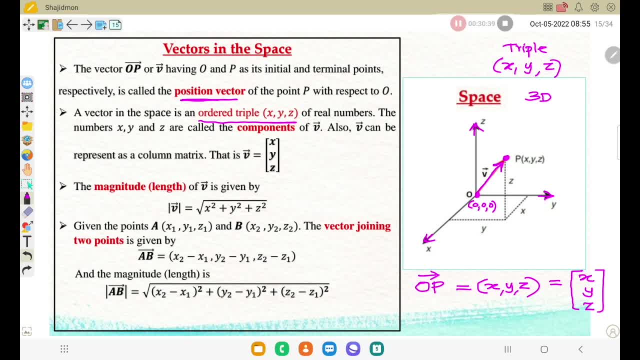 calling position vector in the space starting from o point. okay, zero point. that is the position vector x, called x component, y, we are calling y component and z we are calling z component. okay, now what is the magnitude or length of a vector? magnitude of a vector starting from o up to p. 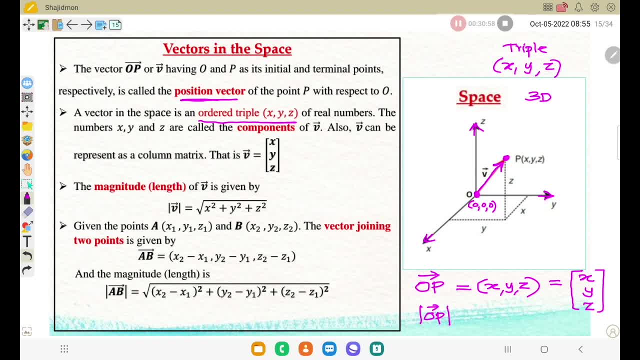 what is the distance? what is the magnitude of vector op in plane? what we have studied? root of x square plus y square- here one more component extra will come. so root of x square plus y square plus z square, that is the magnitude of the vector, vector op. so you can see, here magnitude or length means, okay, root of. 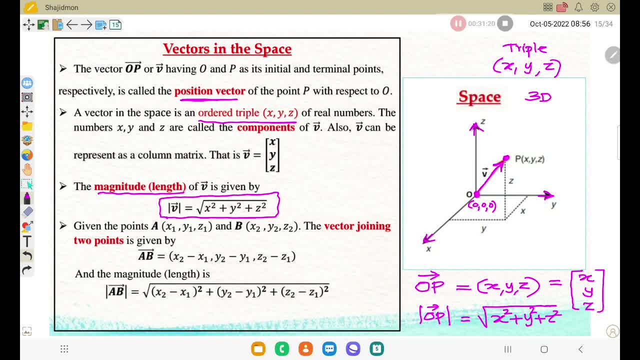 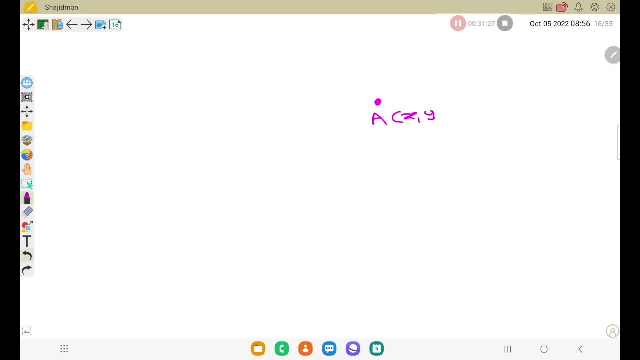 x square plus y square plus z square. now same way vector joining two points. for example: a is one point, a is one point, x 1, y 1, z 1, because three number correct. now the vector ending point b: b means x, 2 comma, y, 2 comma. 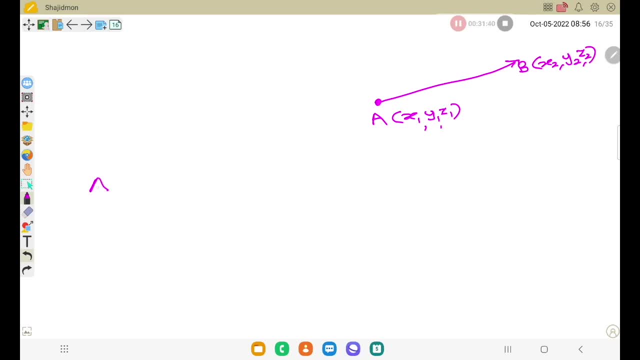 z 2. okay, now, what is the vector joining two points? vector a, b equal to- okay. not starting from the sender. as i told you, if you starting with the sender means position vector, it is vector joining two point. so, vector joining two point: vector a, b equal to x, 2. 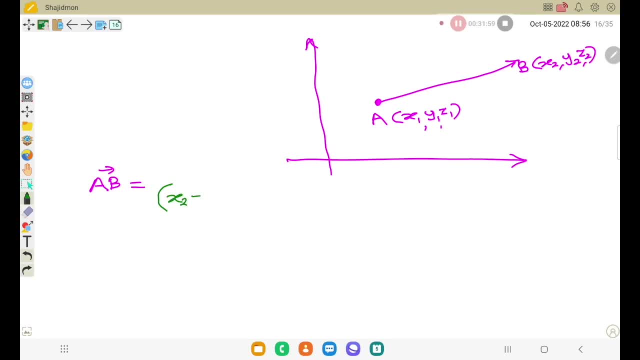 minus x 1, same like in the plane: x 2 minus x 1, y 2 minus y 1. comma now in the plane means one more component will come: z 2 minus z 1. so whatever we are studying in plane, just extend that into the. 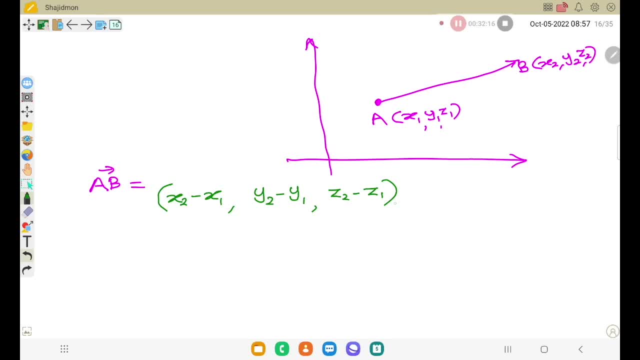 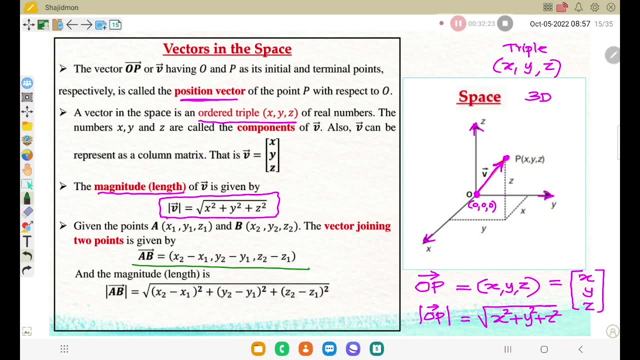 space. okay: x 2 minus x 1. y 2 minus y 1. z 2 minus y 1. okay, so this is the vector joining two point in the space. so vector a, b, you can see here: x 2 minus x 1. y 2 minus y 1. z 2 minus y 1. z 2 minus y 1. 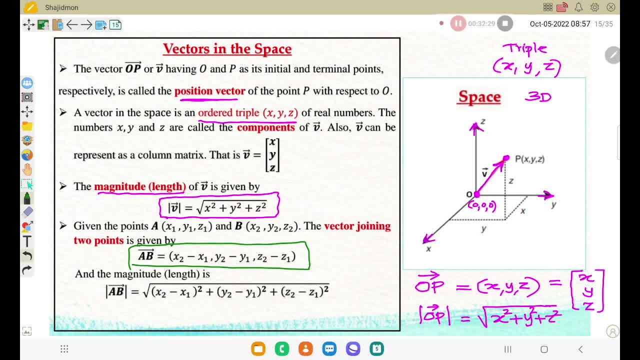 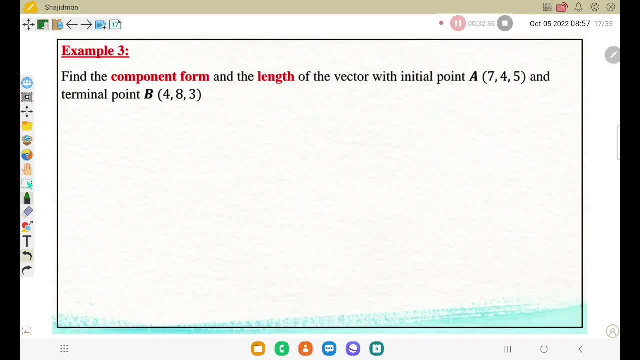 and z 2 minus z 1. now we will go to one question here. example three: find the component form or length of a and length of a vector with initial point a point is 7, 4, 5 and b point, terminal point, b point is 4, 8, 3. okay, so first point, it is given. 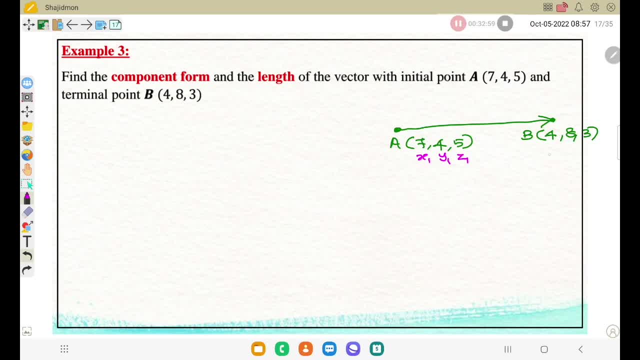 x, 1, y, 1, z, 1. second point: x, 2, y, 2, z, 2, x value, y value, z value like that. now what we need to do, our question: component form of the vector. component form means we need to find x, y, z of that vector. 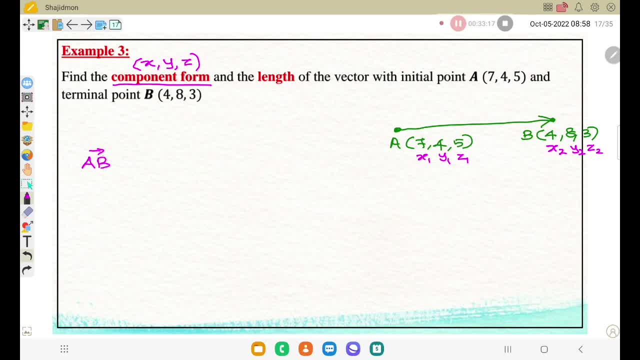 vector a b. what is the x component? vector a- b: what is the y component? vector a b: what is the z component? is that value correct? so what was the rule we are studied? vector a b: equal x, 2, y 2, z 1. x 2 minus x 1. comma. y 2 minus y 1 comma. z 2 minus z 1. correct, just apply the number. what is x 2? 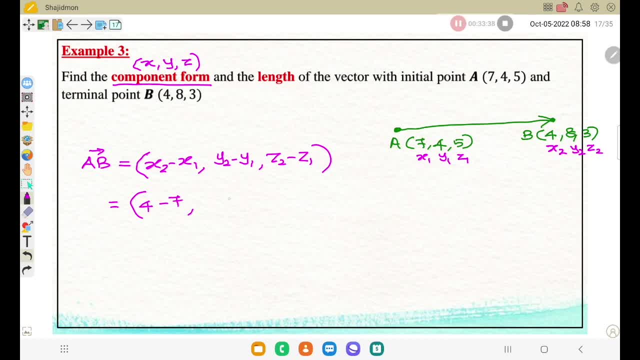 x, 2 means 4 minus 7, y, 2 minus y, 1, 8 minus 4, z 2 minus z, 1, 3 minus 5, correct? i hope you understood that one. okay, how to do that one now? what is the answer? we are getting equal to 4 minus 7 means. 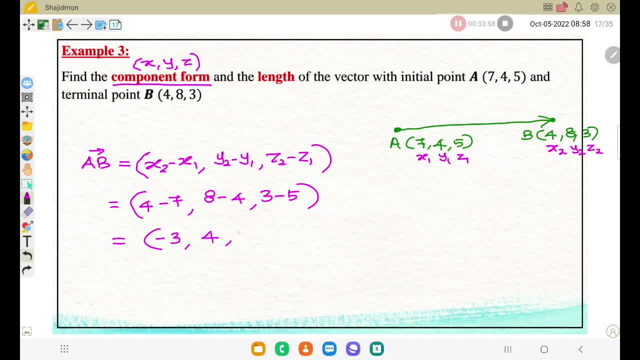 minus 7, and we are getting 4 minus 7, and we are getting 4 minus 7 and we are getting 4 minus 7 and 3, 8 minus 4, 4, 3 minus 5 minus 2. this is the component form x. component form vector a, b. first, 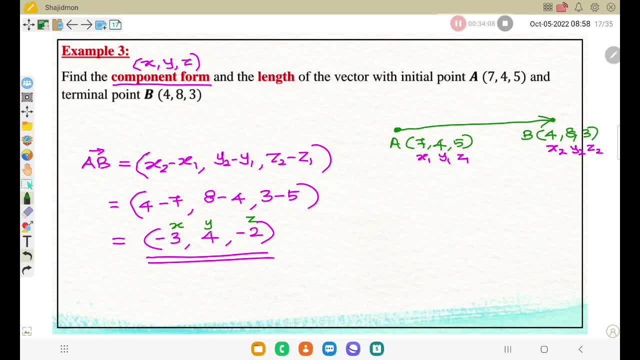 component x. second component y. third component z. now what is the second question? find the length of the vector, length or magnitude. so magnitude of a b, vector a b equal to what is the rule we are studied? root of x square plus y square plus z square, correct? 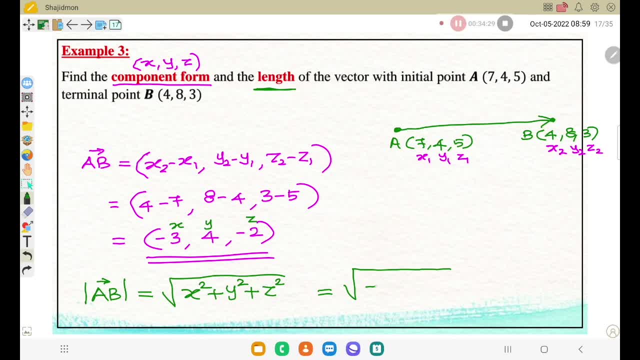 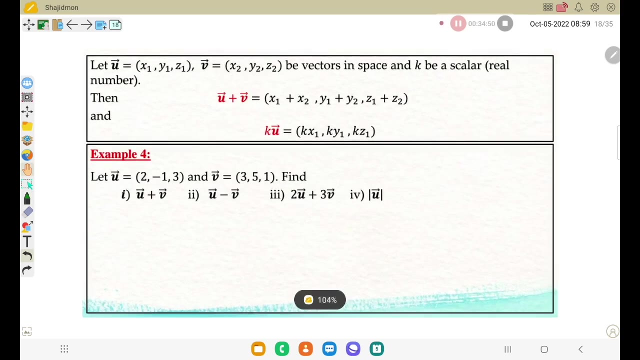 that means root of a b. vector x, component minus 3. just now we calculated: power 2 plus y means 4. power 2 plus z means minus 2 power 2, so that you will get the number root 29. i hope you understood this question in space. okay, now we will go to how to add two vectors, subtract two vector multiply. 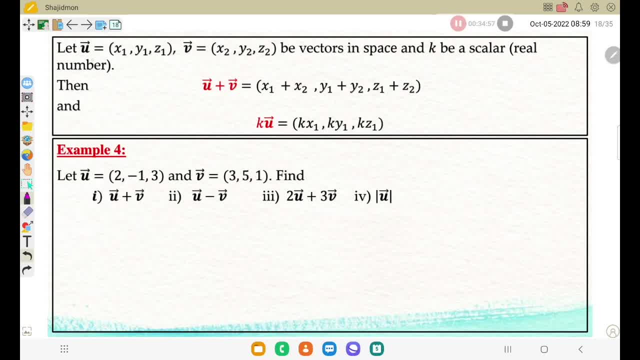 number with vector in. you can see, for example, we have a vector x1, y1, z1, vector v, x2, y2, z2, then u plus v vector means we add two vector x components, add y components, add z components, add x1 plus x2 comma, y1 plus y2. 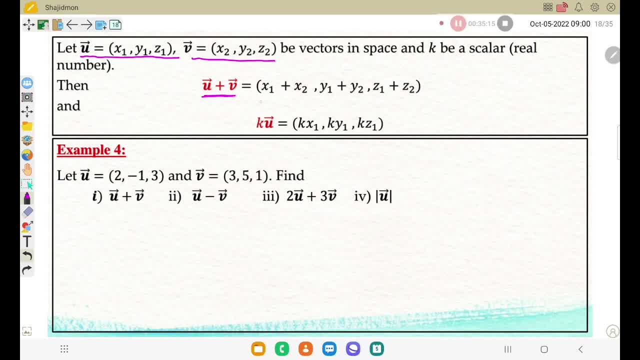 comma, z1 plus z2 and k multiply u. a number multiply a vector means k multiply x1, k multiply y1, k multiply z1. we will go one example, for example: vector u equal to 2 minus 1, 3, vector v equal to 3, 5, 1. find u plus v. first vector u plus vector v equal to what is u, 2 minus 1, 3 plus what is vector. 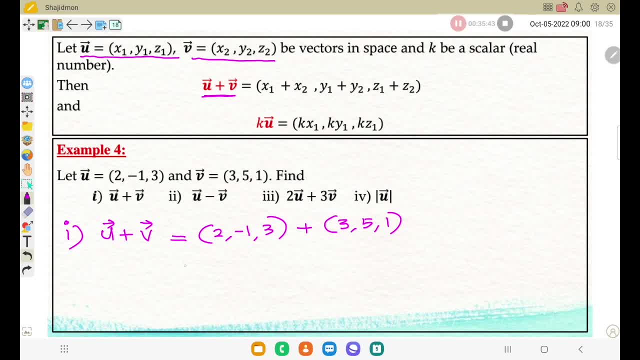 v 3, 5 and 1. now add the numbers same like in the plane. first numbers: add 2 plus 3. hope you understood. first x number here, x number here add. okay, so we will get 2 plus 3. that means 5 minus 1 plus 5. 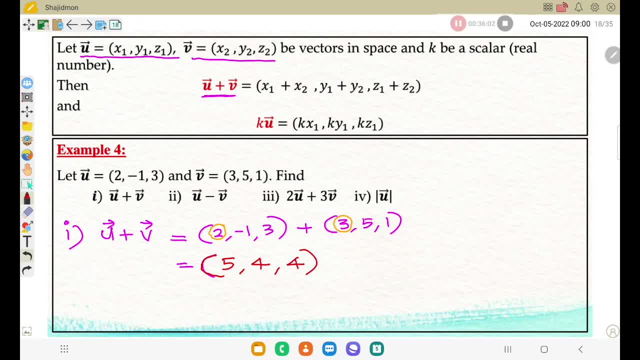 4, 3 plus 1, 4, 5, 4, 4. that is the a plus u plus v vector. now second question: what is vector u minus vector v equal? okay, vector u means 2 minus 1, 3 minus subtract. okay, vector v means. 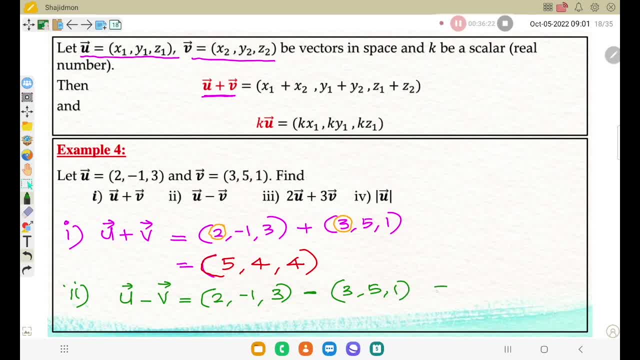 3, 3, 5 and 1. so what answer we go to? just to subtract the first number first: 2 minus 3, 2 minus 3 means okay, same like subtraction minus 1 minus 1. minus 5 minus 6: okay, and 3 minus 1, that is. 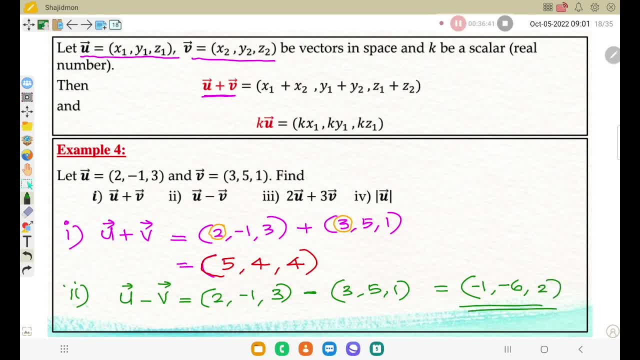 2, so this is the a minus v, u minus v vector. hope you understood. now the third part of the question. okay, we will do 3 and 1, so we call it this: 3 minus 1 and 1. so we will do 3 and 1, so v minus 1. that is two kirchhoff and manual vector. we would need where I will take this and slightly tomato, so we will do 3 and 2 here. since the 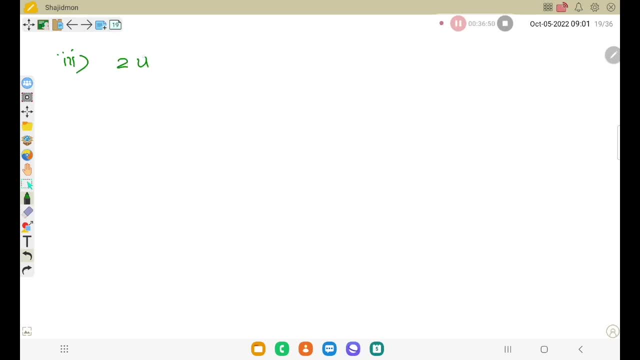 we will do: 2 times vector u plus 3 times vector v, equal to okay. that means 2 times what is vector u: 2 minus 1,, 3 plus 3 times what is vector v. that means 3,, 5 and 1.. Now you know how to multiply. 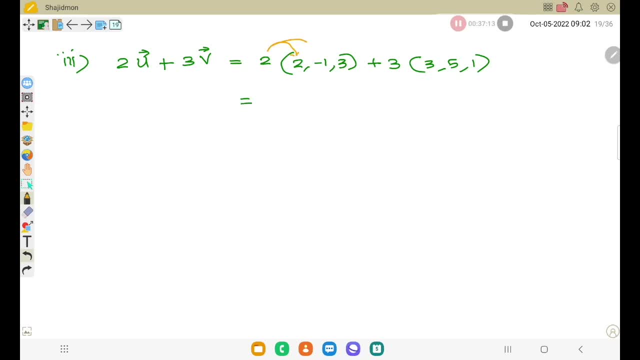 that number 2 inside, Multiply 2 with here here and here Same here also, multiply 2 inside. So you will get 2 multiply 2, 4 minus 2, 2 multiply 3, 6 plus 3 multiply 3, 9, 3 multiply 5, 15,. 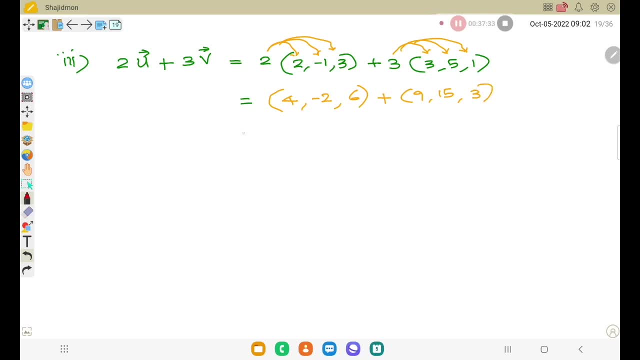 3 multiply 1, 3.. Now, when we are adding these two, you will get 13 comma, 13 comma, 9, correct First number: add 4 plus 9,, 13, minus 2 plus 15,, 13,, 6 plus 3, 9.. So this is the value of that vector. 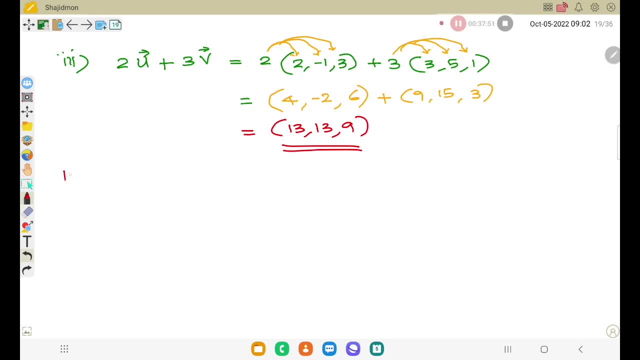 2u plus 3v. Now we will go to the fourth part of the question. that means magnitude of vector u. magnitude of vector u. that is the fourth part of the question. What is magnitude of a vector? we studied Root of x power. 2 plus y power. 2 plus z power. 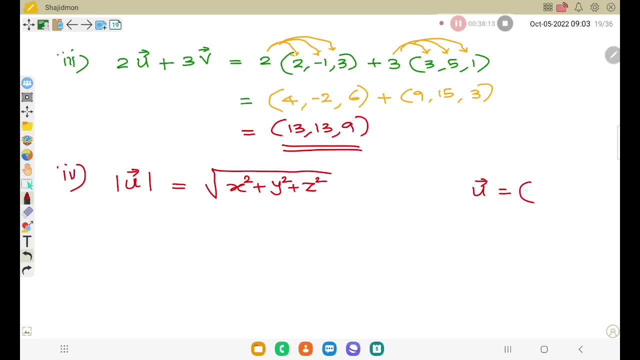 2.. Now you know what is u vector, What is the u vector given 2 minus 1,, 3.. So what is the magnitude root of x: power 2,. x means 2, power 2 plus y minus 1. power 2 plus z: 3: power 2.. So 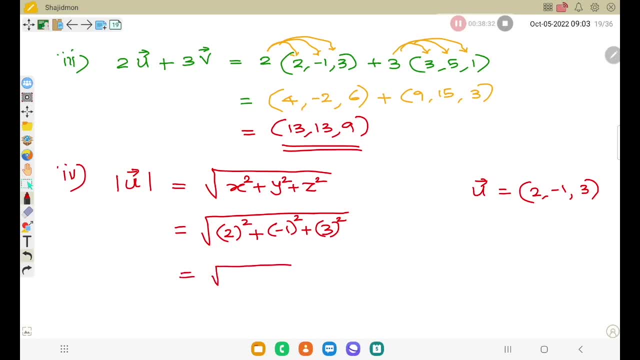 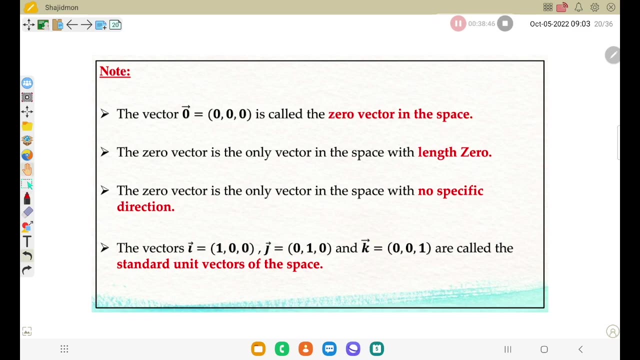 you can check by calculator. It is 4 plus 1 plus 9 root. that means root 14.. That is the magnitude of vector u. I hope you understood How to add, subtract and multiply in space. Now there is some nodes same like in the. 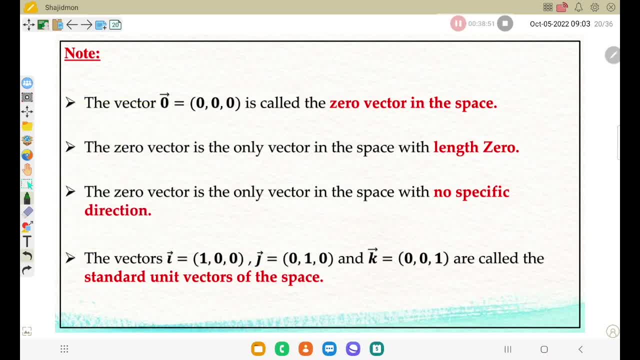 plane The vector in the space: 0 vector 0. comma 0 comma 0, x number 0, y number 0, z number 0.. This is called 0 vector in the space, vector 0, 0 vector notation And this: 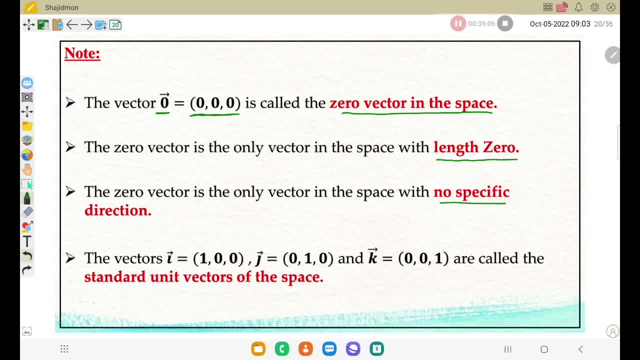 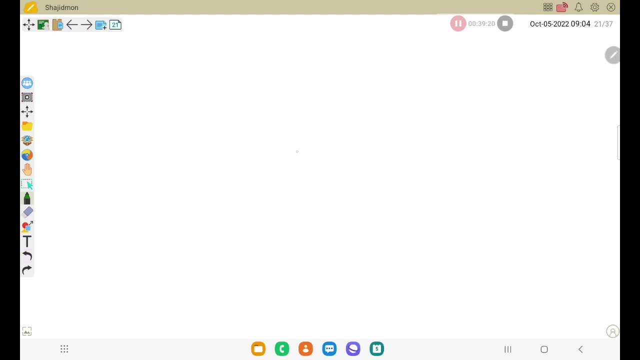 vector 0. vector length should be 0 and there is no specific direction for the 0 vector. Now, what are the standard unit vectors in the space? This is what important. What are the standard unit vectors in the space? Okay, So we can see. we have in space x axis is there? 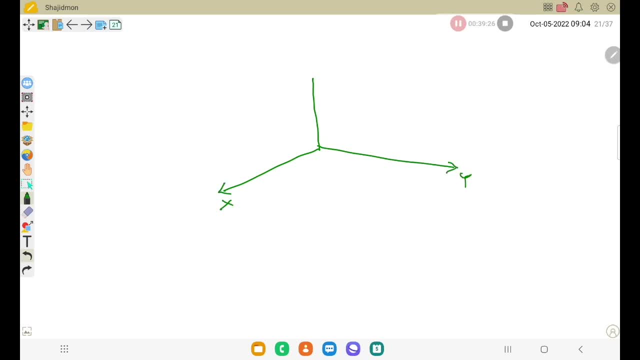 y axis is there, This is x, This is y axis and this is z axis, correct? Now when we are taking the number x, axis number 1, y axis 1, z axis 1, standard unit vector: 1 vector. okay, 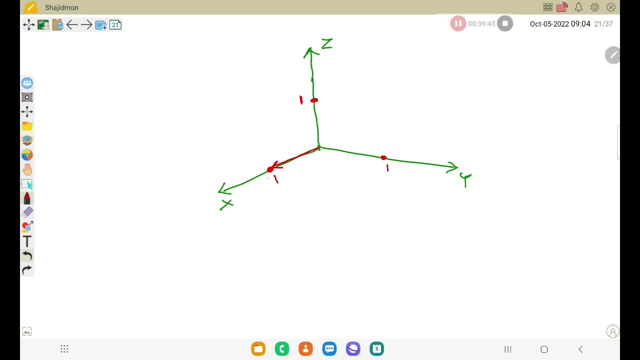 So this vector, what is this? vector 1 means, what is the meaning? x1, y0, z0.. This is what we are calling vector i And here, okay, x0, y1, z0.. This is we are calling vector j And here. 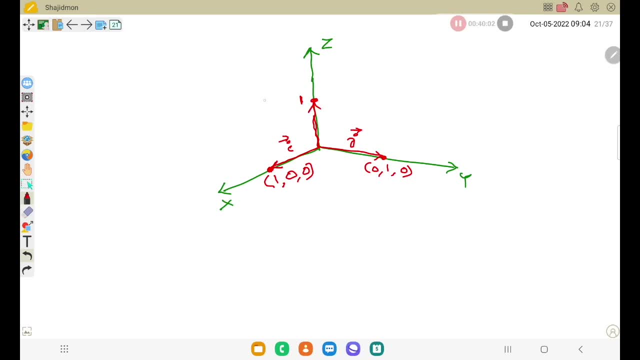 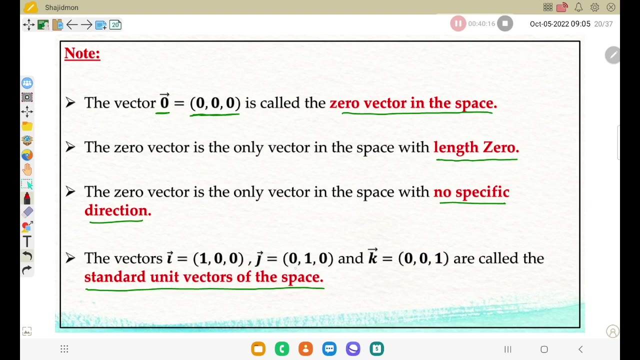 if you are taking a vector here, what is this point? x0, y0, but z1.. This is we are calling vector k. So what are the standard unit vectors In the x, y, z space three dimension? vector i means 1, 0, 0.. Vector j means 0, 1, 0.. Vector k: 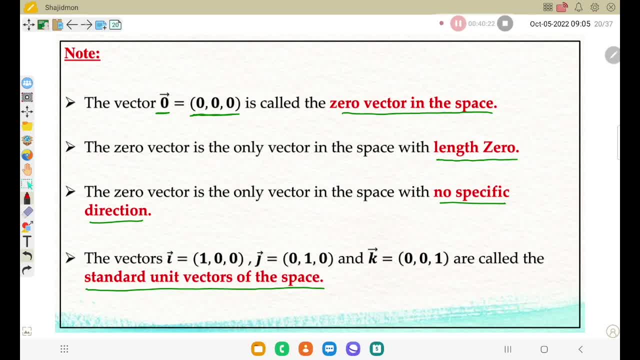 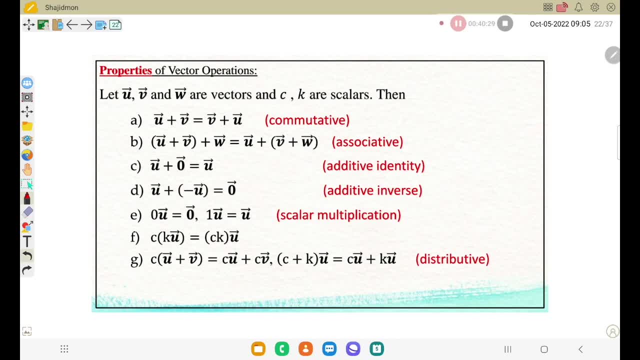 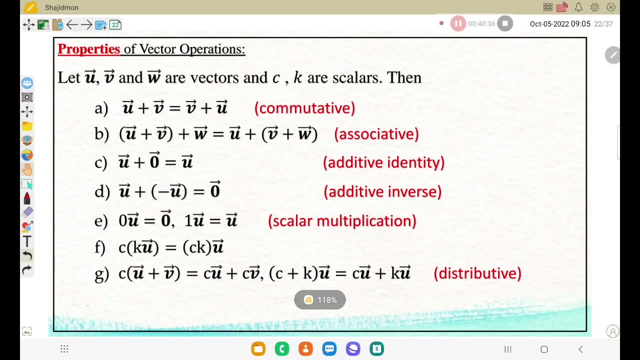 means 0, 0,, 1.. This we are calling the standard unit vectors in the space. I hope you understood. Now there are some properties here. You can read this one: u plus v and v plus u- always same commutative And associative property. u plus v plus w means u plus v plus w. 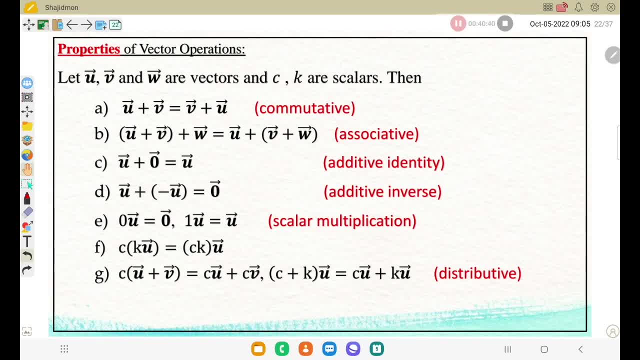 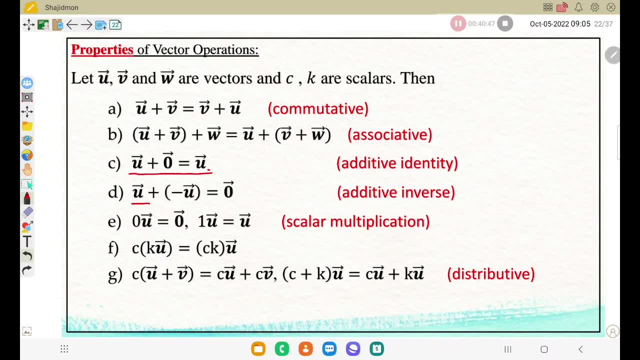 same And additive identity: 0 vector and u vector. when we are adding, always you are getting same vector vector, u, u vector and minus u vector. when you are adding, you will get 0 vector And when we are multiplying 0 with a vector, always answer with a 0 vector And same with. 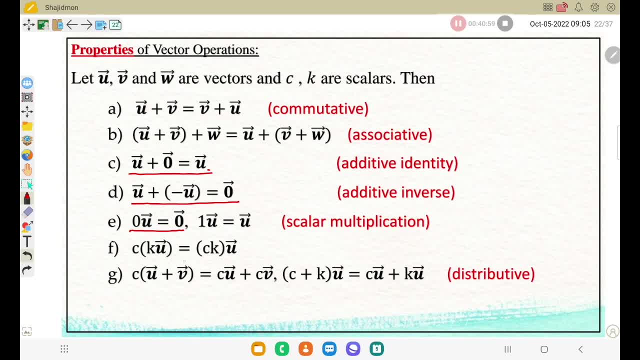 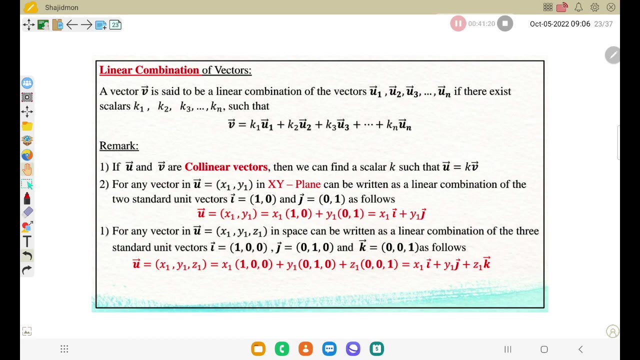 c multiply k multiply u equals c, k multiply u vector And the distributive property. here also we can say: c multiply vector u plus vector v means c multiply vector u and c multiply vector v. That is the distributive property. Now we will go to this one linear combination. What is the meaning of linear combination of? 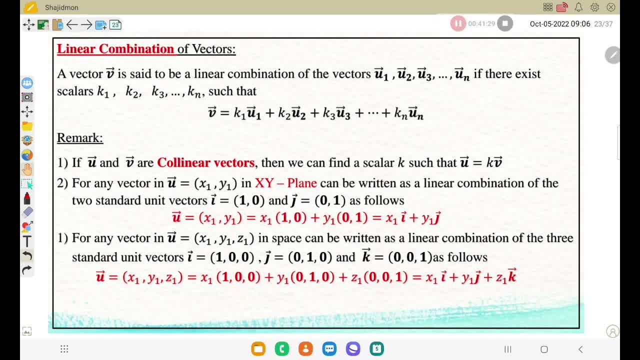 vectors, How to combine the vectors? What is the linear combination? For example, we have a vector: vector v is said to be a linear combination of u1, u2, u3 and un, When we are telling there exist some scalars, c1, c2, c3, up to cn, such that 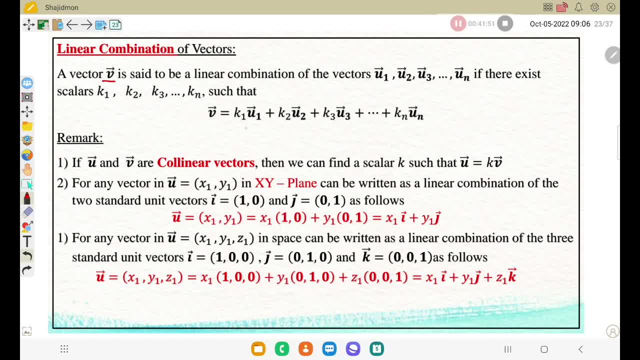 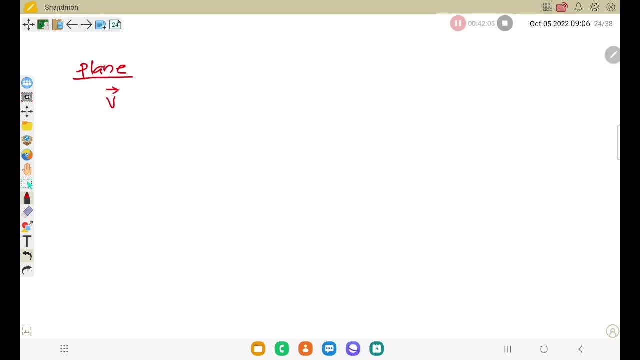 vector v equal to c1 multiply vector u1, c2 multiply vector u2, and c3 multiply vector u3 up to cn multiply vector un, For example. Steve, in plain, I'm just taking a vector, vector v, and another two vectors, vector u1, and vector u2.. So vector v is just going. 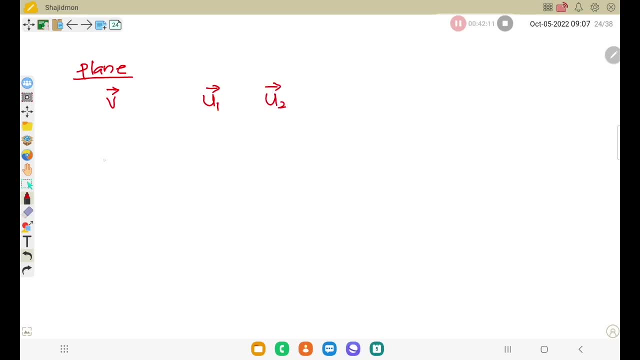 to be a vector V is multi vector. vector v is the number of vectors. But when we go to and vector u2.. When we are telling this vector is a linear combination of u1 and u2, okay, in the plane we can take two scalar numbers. Scalar number- I am taking x and y. okay, scalar. 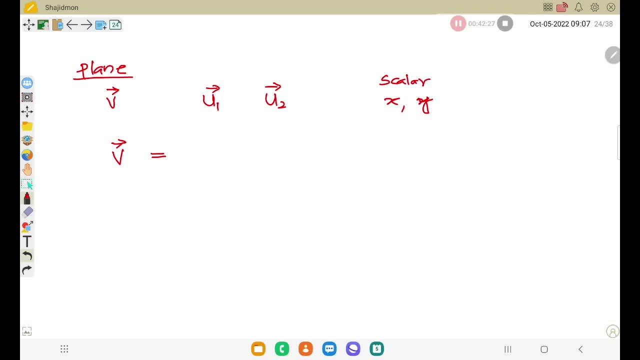 Scalar number x and y. So vector v is a linear combination of u1 and u2. means a scalar multiply vector u1, a number multiply vector u1 plus another scalar, another number, y multiply vector u2.. What answer? it should be: Vector v: x number multiply u1, vector plus number. 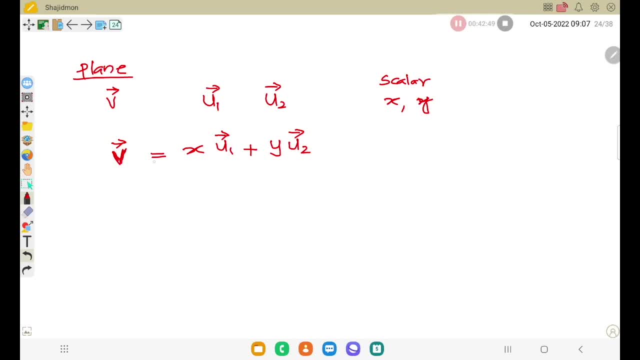 multiply u2 vector, You should get vector v. Then we are telling: v is a linear combination of u1 and u2.. Now same in space. for example, space, If I am taking the vector vector v and another vector is u1, u2 and u3 vector: three vectors, any three vectors. 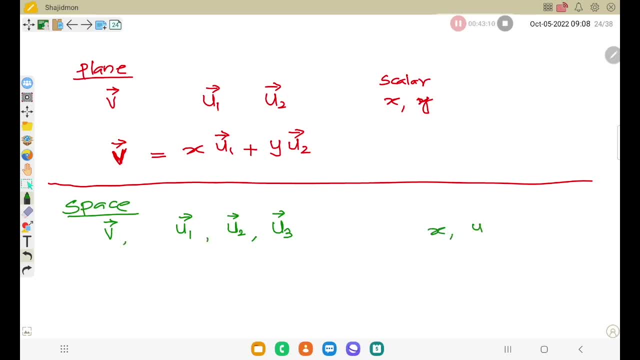 Now I am taking the scalars x, y and z. These three are scalars, for example. okay, Instead of k1, k2, k3, I am taking x, y, z, like. So, when we are telling vector v is a linear combination of: 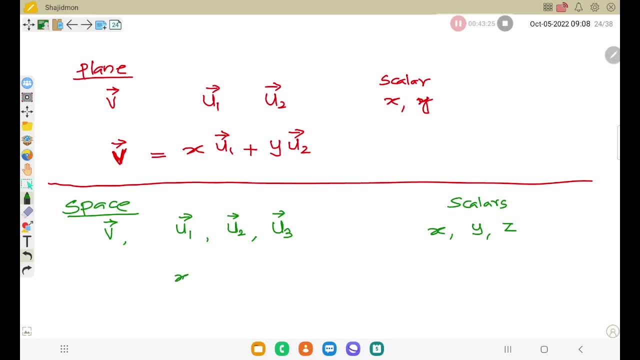 u1, u2, u3, just calculate x multiply u1 vector plus y multiply vector u2 plus z multiply vector u3.. You will get same as vector v. If you are getting same vector v, then vector v is a linear combination of u1, u2 and u3, okay, So finding this number, 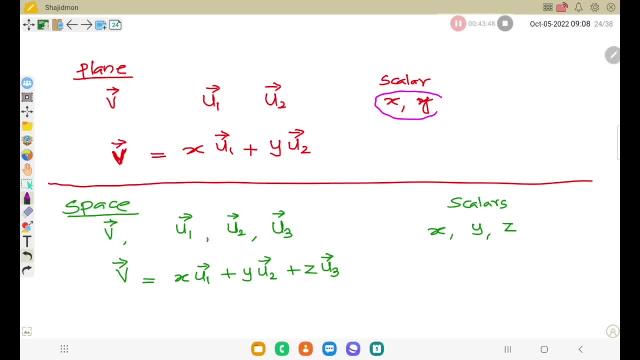 this is the important thing. okay, If you want to write the linear combination, we need to get this number, x and y, x, y and z here. okay, If this number we can find, then we can write the linear combination. Otherwise, linear combination not exist, okay. So this: 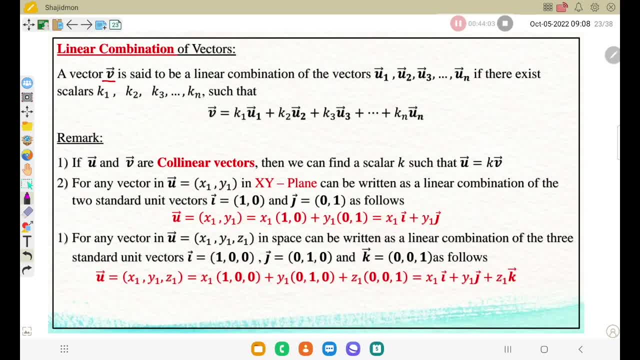 is the idea here. Combine the vector adding, multiply and add, So like this: This is the general Vector v equal to k1,, u1,, k2, k3, k4, k5, k6, k7,, k8, k9,, k9,, k10,, k11,, k12,, k12,, k13,, k13,, k14,, k14,, k14,. 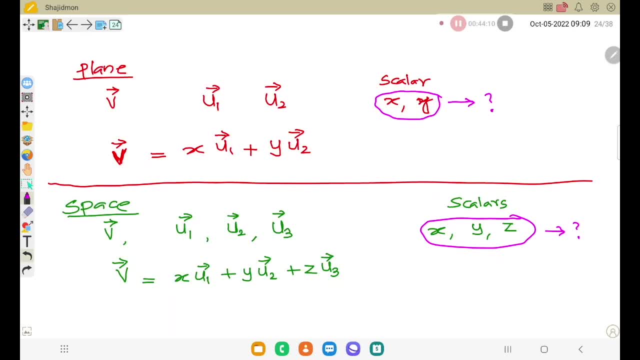 k15, k16, k15, k17, k18, k19,, k19, k20,, k21, k22, up to the last. So at least you can just remember these two plain. How can we write the linear combination space? How can we write? 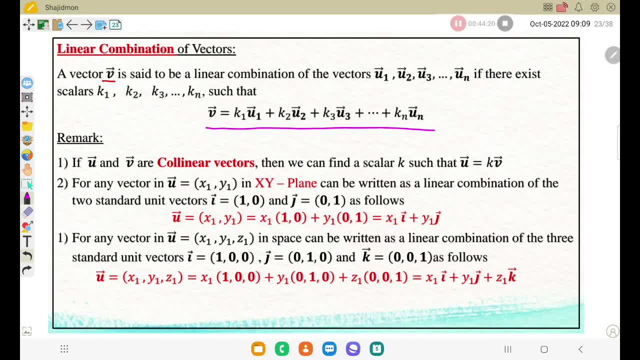 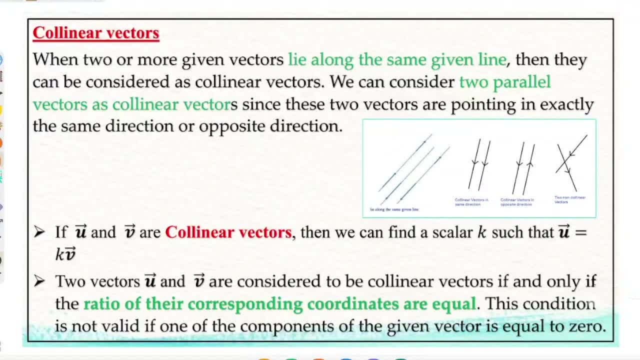 the linear combination. Now there is some point here we need to memorize or we need to know. It is easy: One, two vectors are said to be collinear vectors. So collinear means we will discuss here in detail, okay. collinear vectors: So when two vectors or more vectors lie along the same. 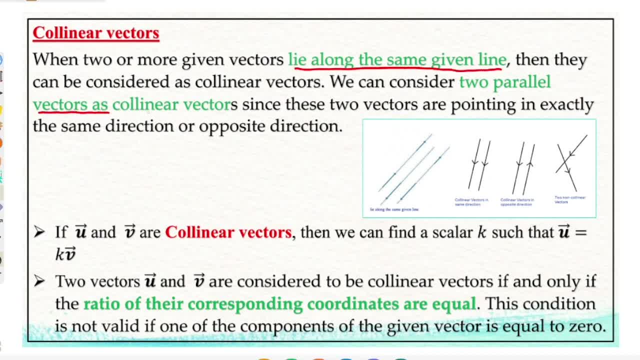 given line, okay. or the parallel vectors- okay, is said to be collinear vectors. for example, you can see some figure i shown here. see this example: this vector and this vector lying on the along the same given line, correct, so it is same direction also. but here you can see another. 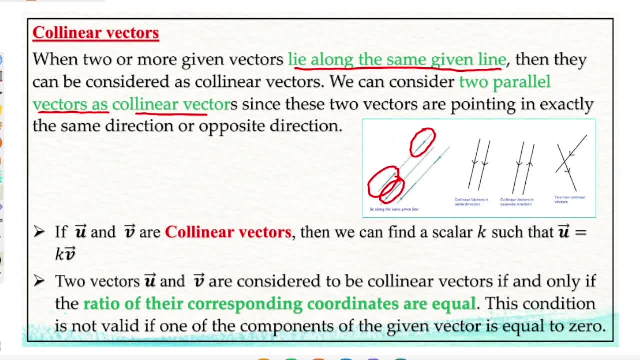 two vectors here, another two vectors here. if you are taking it is same line of action, correct, opposite direction, but along the same given line. so these two vectors are collinear vectors, correct? and another figure: you can see two vectors here, one vector and another vector here, parallel with. 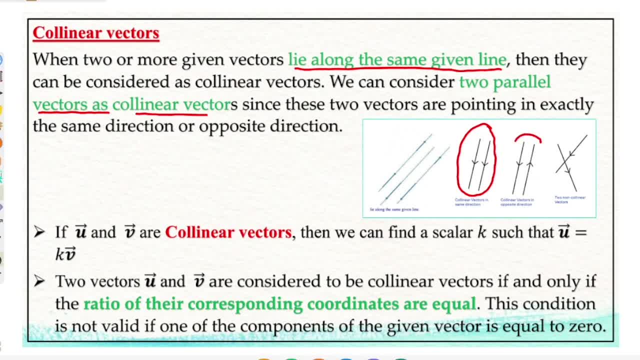 the same direction. so these are the collinear vectors. now, here see, two vectors are parallel but opposite direction. so that are the also collinear vectors. but in the last figure you can see these two are not collinear because they are not along the same given line, correct? 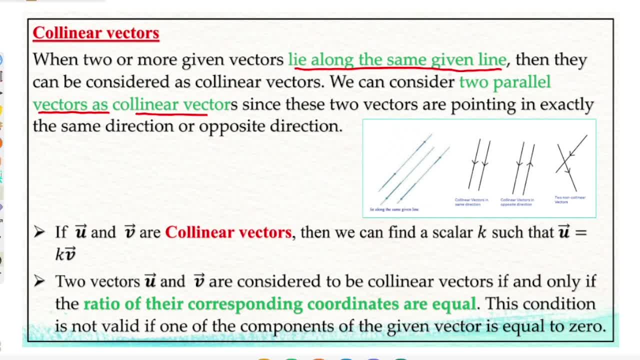 so two or more vectors lie along the same given line, or two parallel vectors, also collinear vectors. okay, So for example, here you see, this is vector u, for example, and this is vector v, for example. see these, both vectors are lie along the same given line, with same direction, so it is collinear vectors. 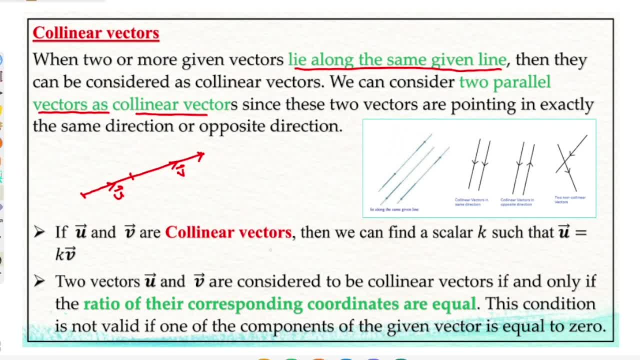 okay, Now what are the conditions for the collinear vectors? you can see here: If u and v are collinear vectors, then we can find a scalar number, k, such that vector u equal to k multiply vector v. that means one of the vector, vector u or vector v, equal to a scalar. 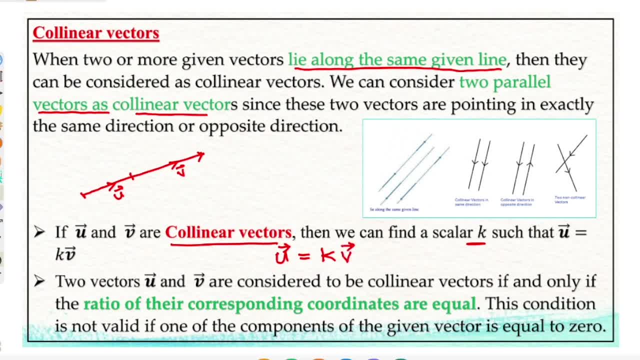 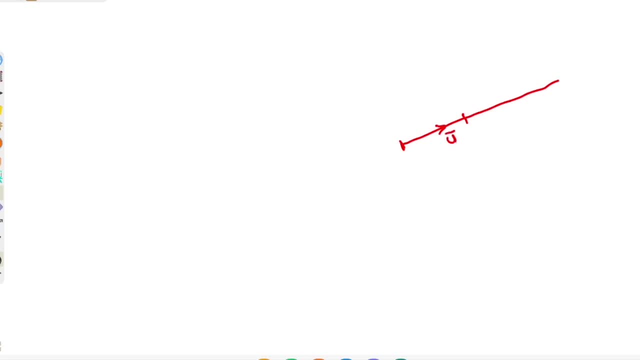 multiple of the second vector, vector u, equal to k multiply vector v. then these two vectors we are calling collinear vectors, correct? These two vectors are calling collinear vectors. okay, So what are the condition collinear? See, for example, one vector here, vector u, and another vector here, vector v. they are lying on. 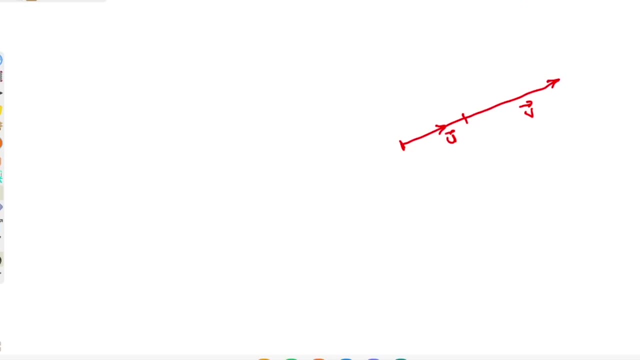 the same line, along the same line, so we can call it as collinear vectors. or if you are taking a vector u here and vector v, correct parallel vectors- this also collinear vectors we are considering irrespective of the direction. see here, it is same direction. Now, for example, if 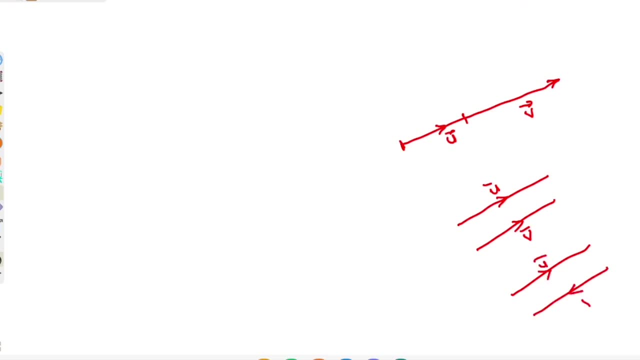 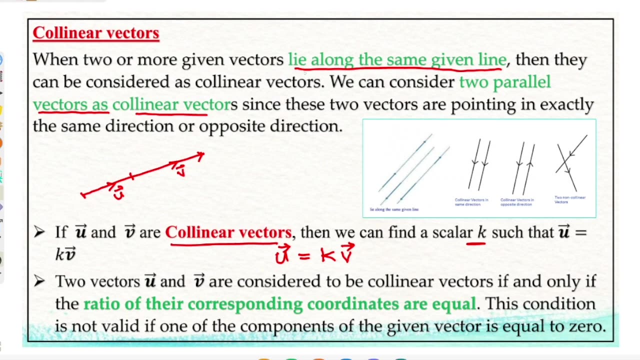 I am taking two vectors here. this is vector u and this is vector v, correct, it is opposite direction. Still, it is collinear vectors. So what is the condition? actually, collinear vectors lie along the same given line along the same given line. or you can say parallel vectors, also collinear. 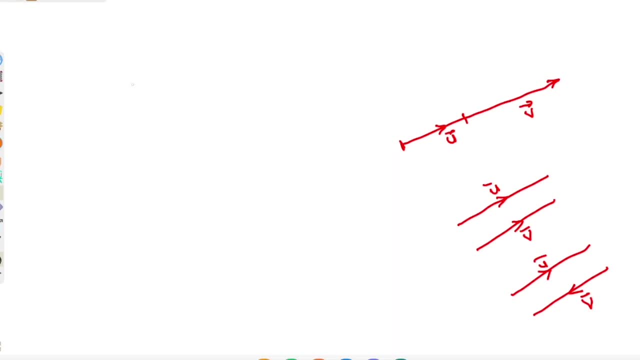 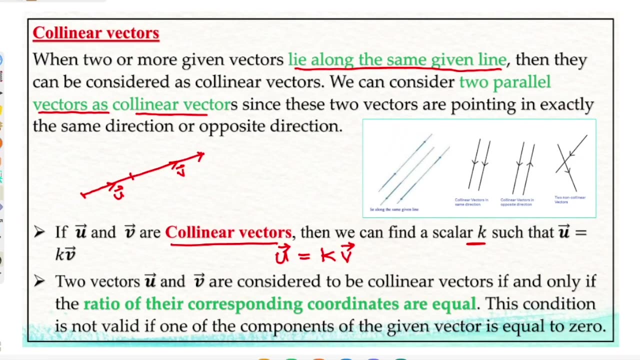 vectors. So what condition, we told, is one of the vector should be equal to a scalar multiple into multiply second vector, or vector v equal to vector v, equal to k multiply u, or u equal to k multiply vector v. Second condition we can check easily: two vectors are collinear. is the ratio of their corresponding? 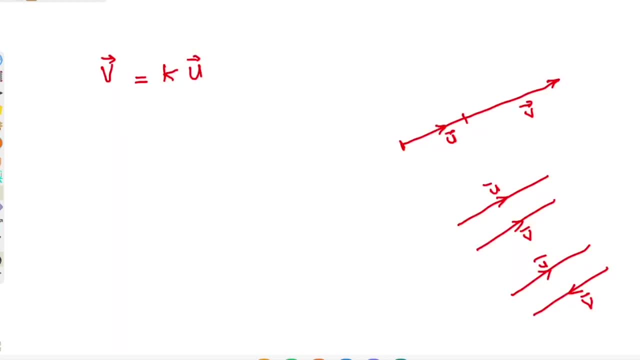 coordinators. coordinates are equal, correct. What is the condition? the ratio of the corresponding coordinates are equal. that means if you are getting a vector and another vector, this is vector u and this is vector v. okay, For example, here x component will be there. for example, 1, 2, 3, okay. 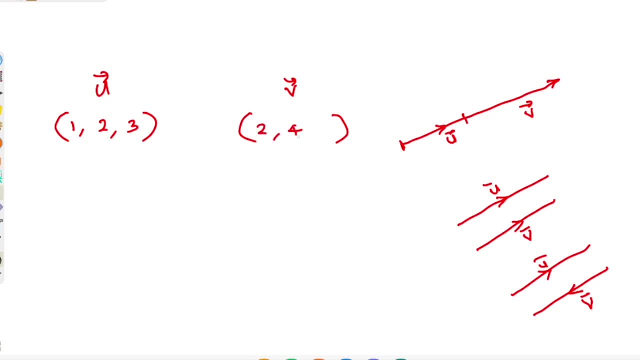 and here you can see for example 2, 4. And 6. So x component ratio. what is the? what are the x component? here 1 and here 2.. So 1 over 2 ratio means just 1 over 2. Then y component ratio: 2 divided by 4 and z component ratio, that means 3. 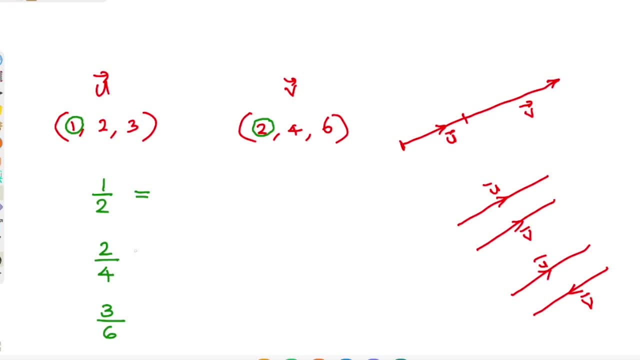 divided by 6. These two numbers will be same. actually see 1 over 2- 0.5. and 2 over 4, also 0.5. 3 over 6, also 0.5.. So we can say these two vectors are collinear vectors. 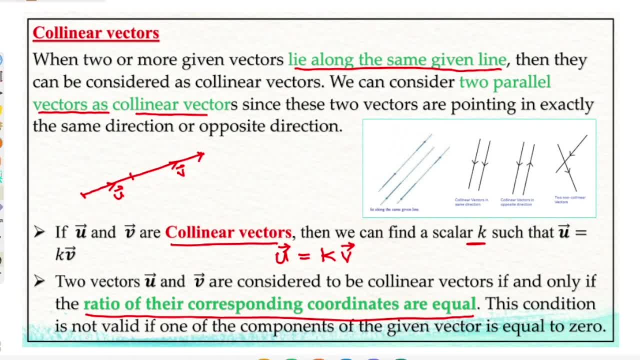 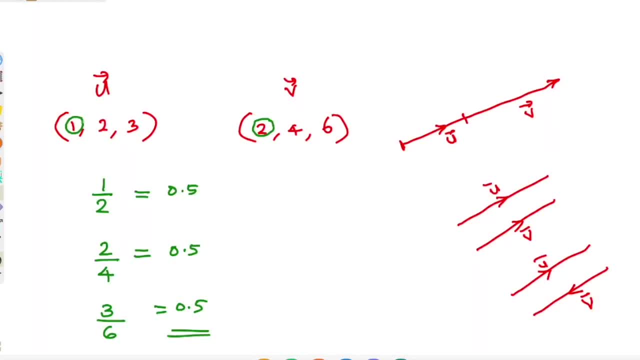 Now one condition here we can see that one. this condition is not valid if one of the component given vectors are equal to 0. For example, here one of the component, for example x, component 0 and second vector, also x, component 0. So we cannot use this ratio method because 0 divided by 0 it is. 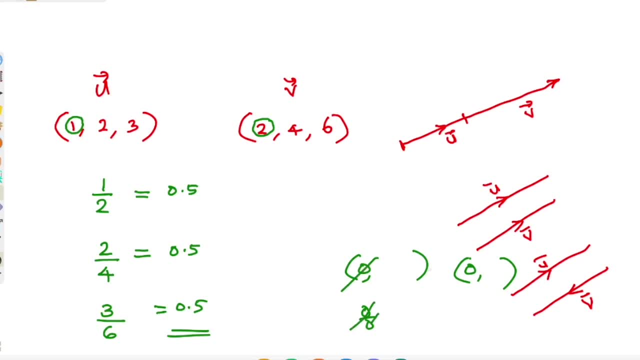 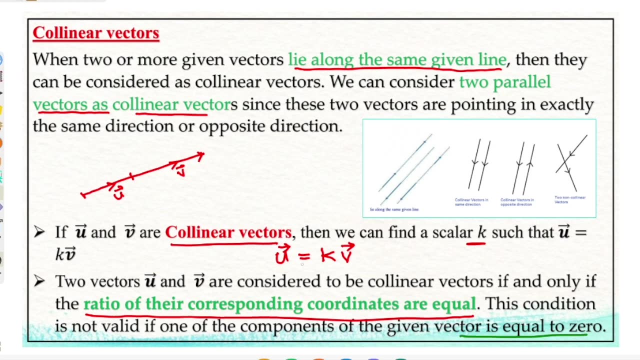 indeterminate form correct, We will not get value correctly. So one of the component 0 means we cannot use this condition. So that time we can use the first condition, One of the vector equal to a scalar multiple of second vector. We will consider some of the 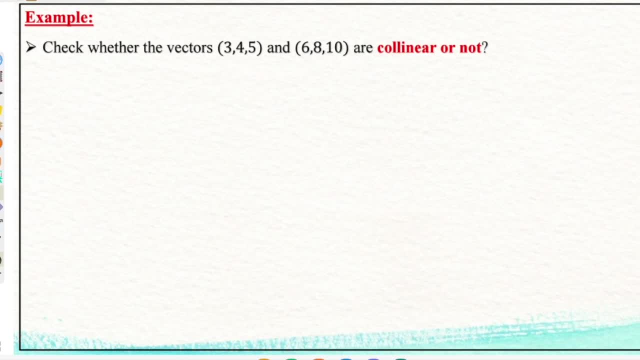 example: here You can see check the check whether the vectors 3, 4, 5 and 6, 8, 10 are collinear or not. okay, collinear or not. So here see none of the component 0, correct x. component 3. y. component 4. 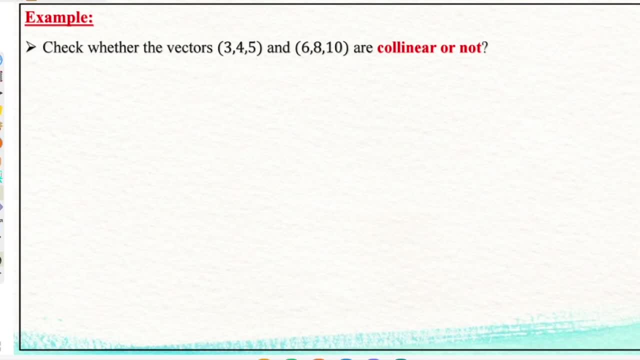 z component 5, second vector, x, component 6, y component 8, z, component 10. correct, not 0, not 0 numbers. So we can use the ratio. We can just check the ratio, okay, When we are telling two vectors are collinear ratios of the. 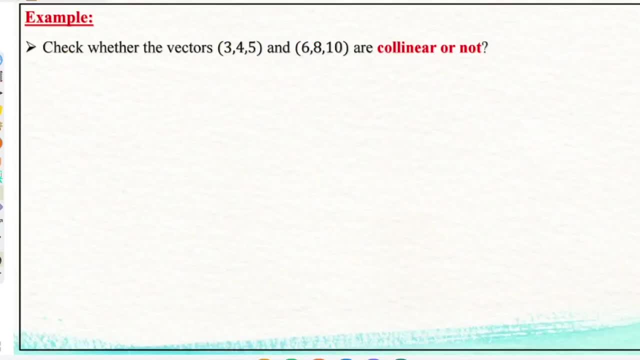 corresponding coordinates are equal. okay, For example, what is the ratio of the x component, x value here 3 divide x value, x component here 6, and y component 4 divided by 8 and z component 5 divided by 10.. We can check these three numbers will be same, correct: 3 over 6.. 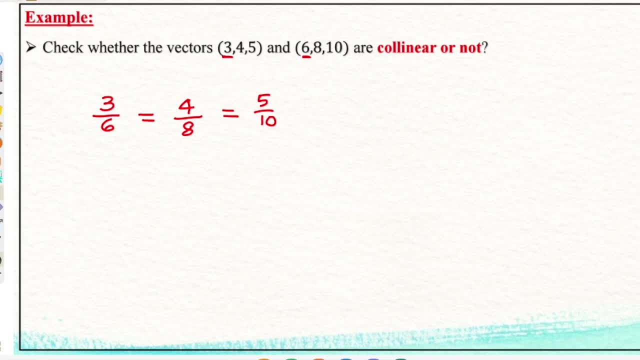 4 over 8, 5 over 10. both are 0.5, both are same, correct. Both all these ratios are same. that means 3 over 6.. 3 over 6 means 1 over 2, that means 0.5 and 4 over 8. you can see 0.5 and 5 over 10. 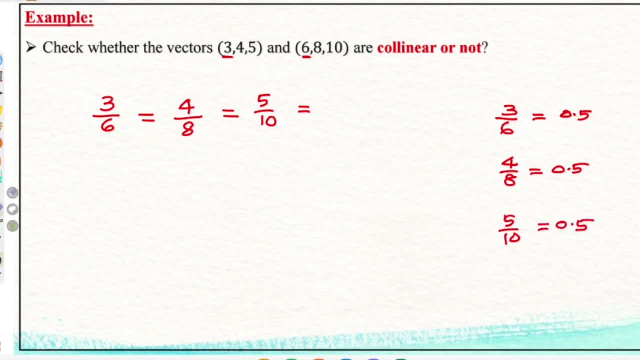 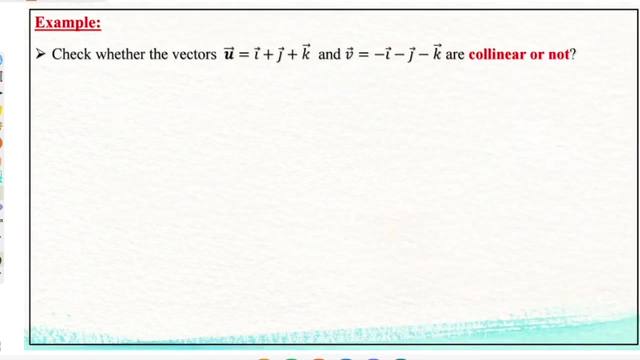 also 0.5.. So these three ratios are same. These three ratios are same means what we can say that two vectors are collinear vectors. Okay, so simply, we can check using the second condition. okay, Now, for example, another example you can see: check whether the vectors are collinear or not. okay, So what is the first? 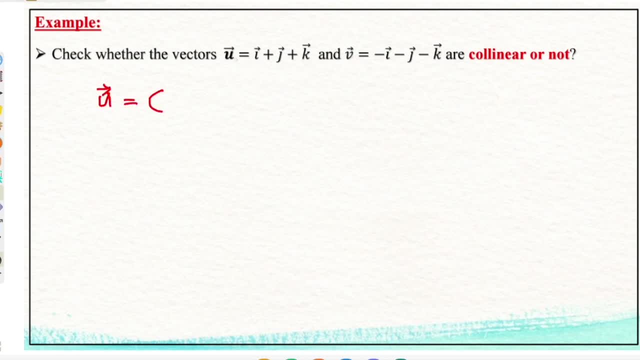 vector. Vector u: equal. We can write in component ways. What is the x component? x component means i behind number 1.. y component means j behind number 1.. z component means k behind number. that is 1, correct. Now same way vector v: we can write in component ways. What is the i component? 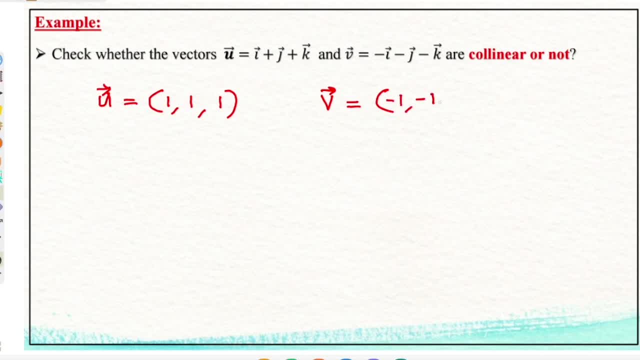 i component minus 1.. j component or y component is minus 1 and z component is minus 1.. Now check whether these two vectors are collinear or not. How we can do: Just take the ratios of the components: x component 1 divided by minus 1.. Here x component is 1.. Here x component. 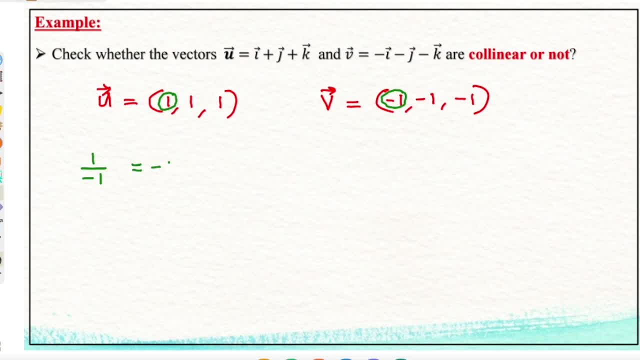 is minus 1.. So 1 over minus 1, that is minus 1. correct. Now y component: 1: again 1 over minus 1, that is minus 1.. z component also: 1 over minus 1, that is minus 1.. So the ratios are same. correct. So the ratios. 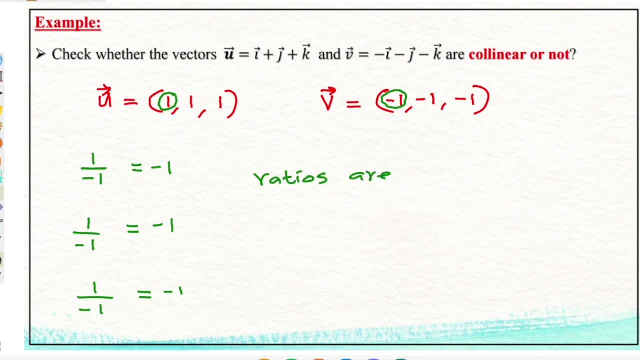 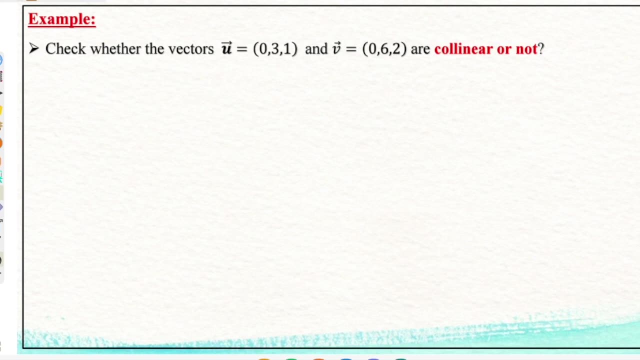 are same, We can say ratios are same. If the ratios are same means what? we can say that two vectors are collinear vectors. Hope you understood the meaning of the collinear. Now one more example we can see. check whether the vectors are collinear or not. okay, So in this, 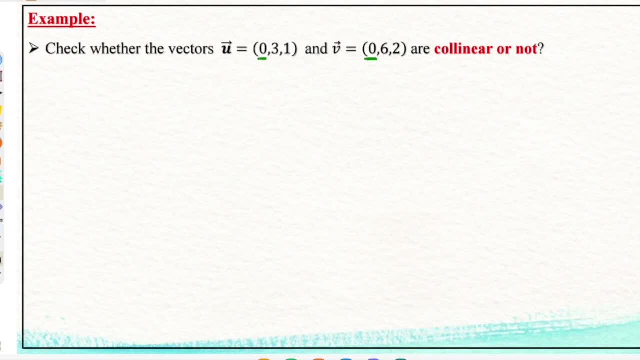 example, see: one of the component is 0. I cannot use the ratio. If you are using ratio, answer will not get it. Answer get it means it is 0 by 0 form will come correct. So this case, what we are doing using the first. 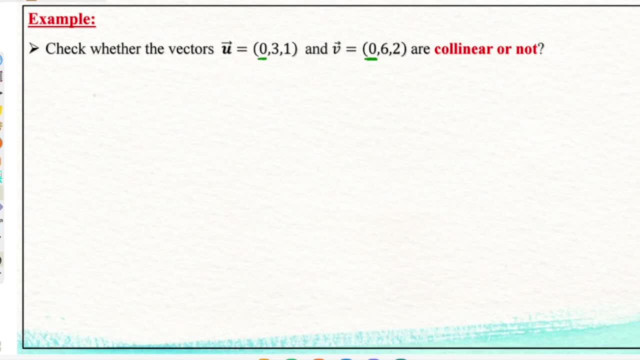 condition When we are telling two vectors are collinear, one of the vector- okay, either vector v or vector u should be a scalar multiple of second vector: okay, Vector v equal to k multiply vector u: okay. If we can write like this, we can say that two vectors are collinear. 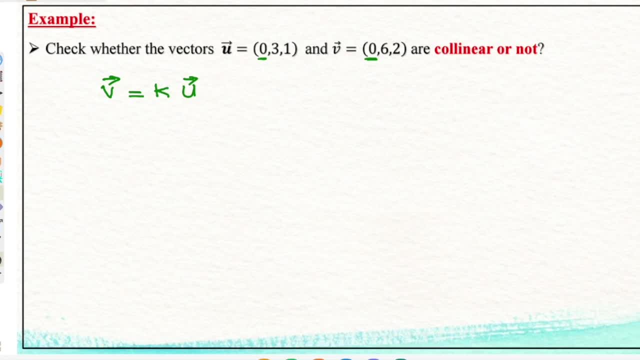 vectors. okay, For example. here we can see, for example, vector v. what is vector v? 0, 6, 2 equal to k times? what is vector u? 0, 3 and 1? correct, Now that means 0, 6, 2 equal to k multiply. 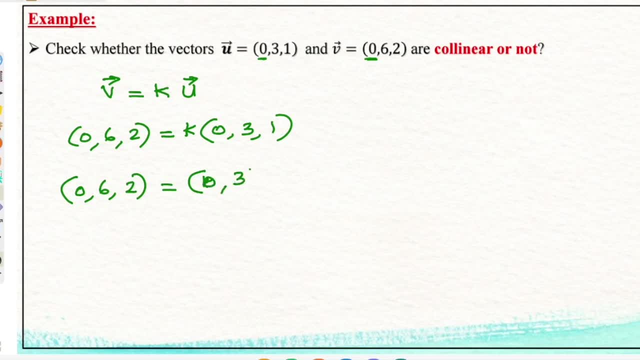 0, that is 0, and k multiply 3, 3 k and k multiply 1, that is k, correct Now. first vector equal to second vector means components are same. See the first component: 0, here also 0. same Second component here: 6, here 3k. So 3k equal to 6, correct. So what? 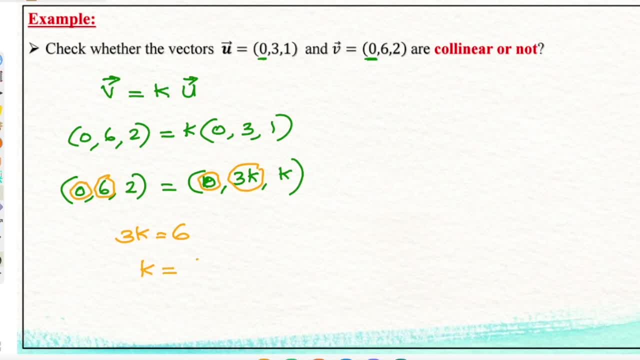 will be the k number. k number equal to divide both side by 3. 6 over 3, that means 2, correct? So what is the meaning of that one first vector? sorry, vector v. we can write it as k. k means 2 times vector u, correct? 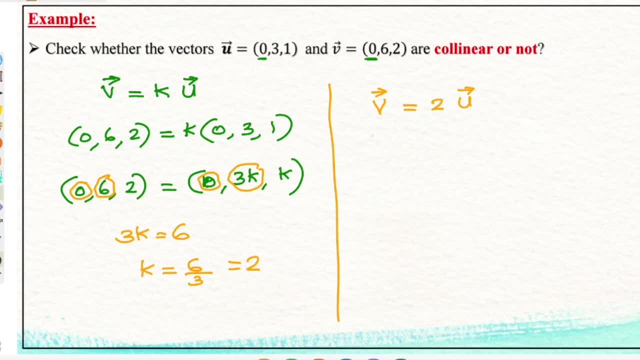 If we can write like this, that two vectors are said to be collinear vectors, okay, One vector equal to a scalar multiple of another vector. It is easy to understand this case. See, for example, vector u: 0, 3, 1. correct. I will show that one here. You can see vector. 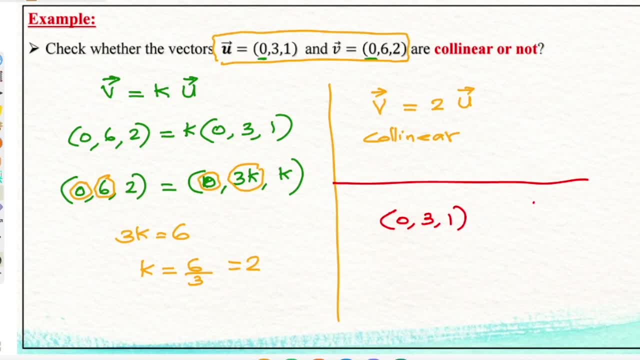 u means 0 comma 3 comma 1.. Vector v means 0 comma 6 comma 2, correct Now this. see the vector v. this is vector u. You can see the vector v, What number we can take it common. you can see 0, 6, 2, correct, So you can take 2 common. 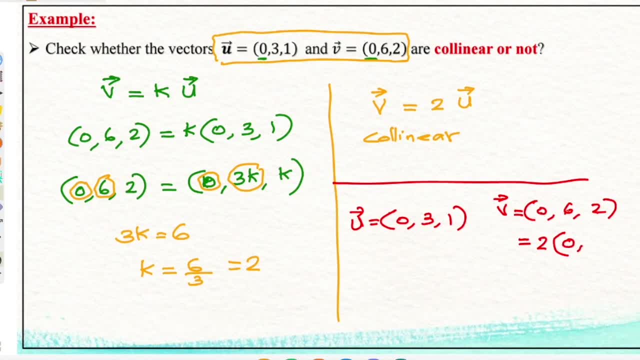 2. common means what will be the balance? 0 comma. 6 over 2 means 3.. 6 over 2 over 2 means 1. That means if, when we are multiplying that one, you will get the same: 2 multiply 0, 0, 2. 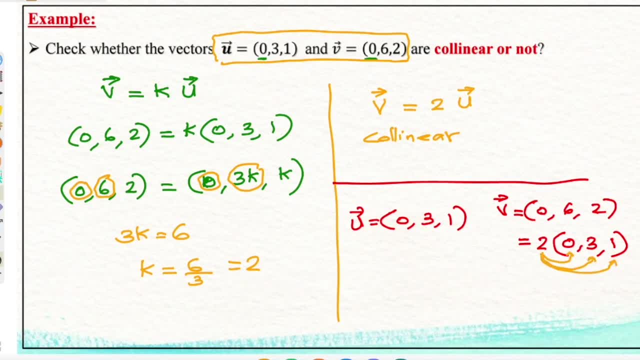 multiply 3, 6, 2. multiply 1: 2- correct. So what is the meaning of this one? 2 multiply 0, 3, 1 means what is that vector vector u correct? So 2 times vector u. So vector v equal to 2 times vector u. okay, So these two vectors. 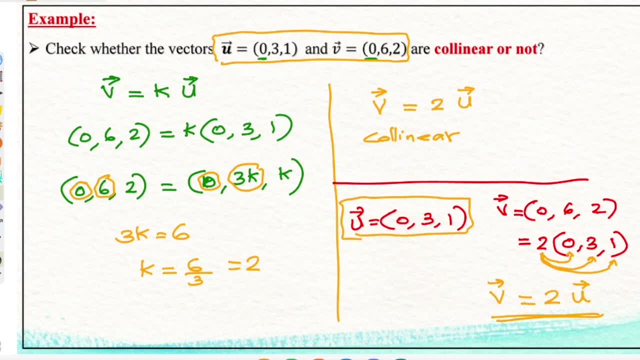 we can said to be collinear vectors. So two ways we can check. Either we can check by ratio, checking the ratios. But when we are checking with ratios, one of the components should not be 0. Other ways we can check it like this: One vector equal to a constant. 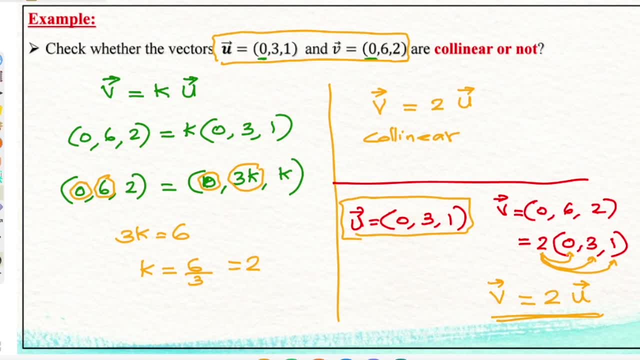 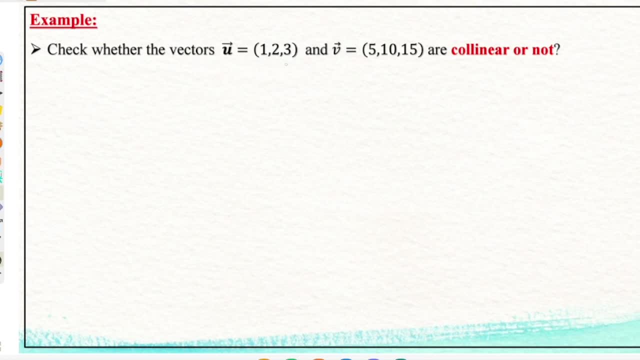 a scalar multiple of the second vector. So this is the idea here. Now one or two examples More we can discuss. For example, check the vectors: Vector u, equal to 1, 2, 3 and vector v, equal to 5, 10, 15 are collinear or not. Okay, collinear or not, Here you can see, here the 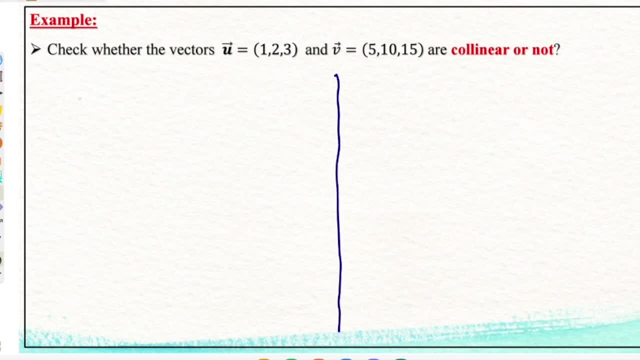 components are not 0. So we can use the ratio. For example, x component in the first vector is 1 divided by x component in the second vector is 5. 1 divided by 5. Y component ratio: 2. 3 divided by 10. Z component ratio: 3 divided by 15, correct 3 divided by 15.. Now you know. 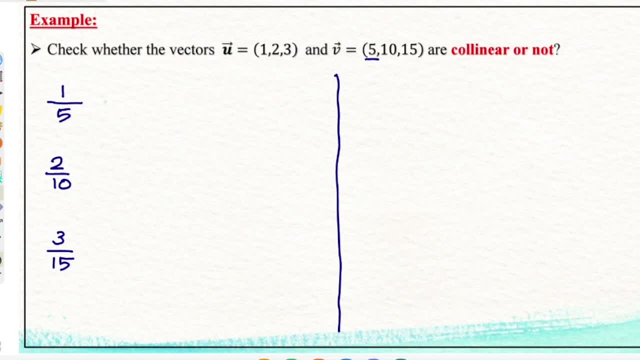 1 divided by 5 means 0.2, correct 0.2.. 2 divided by 10, also 0.2, and 3 divided by 15, also 0.2. here correct. So ratios are same, Ratios are same ratio, correct Same ratio. So this is. 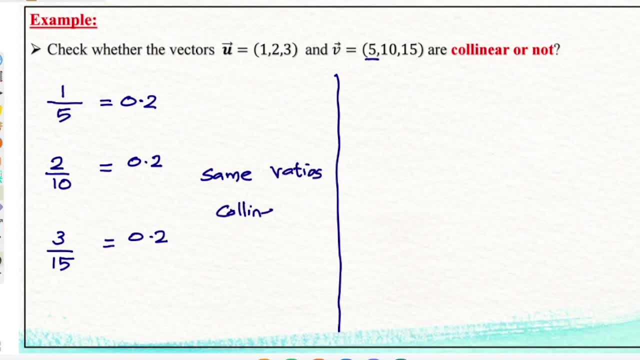 the answer. So what is the answer? That two vectors are collinear vectors. Hope you understood that one. Now, for example, the same question. Okay, depends on your understanding. You can do like this also: What is vector v? Vector v equals 5, 10 and 15, correct? What is the? 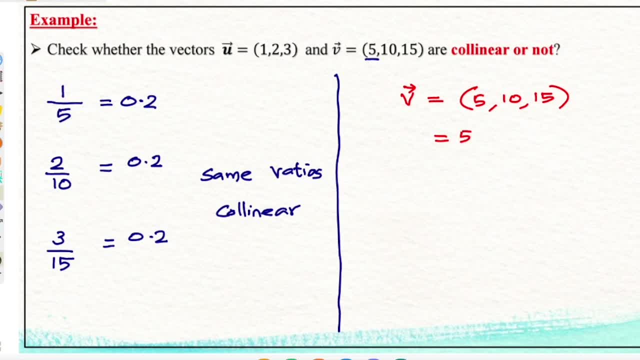 number we can take common here: 5, 10 and 15.. 5 we can take it outside. So what will be the balance? Okay, 5 divided by 5. 5 we are taken. So 5 divided by 5. 5 we are taken. 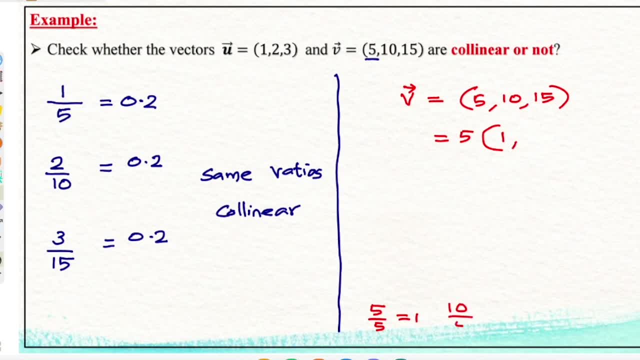 So 1 balance correct. Now, 10 divided by 5 means 2 balance. Now 15 divided by 2. 5 means 3 balance correct. So 1: 2, 3 correct, Because 5 multiply 1, 5. 5 multiply 2, 10. 5 multiply. 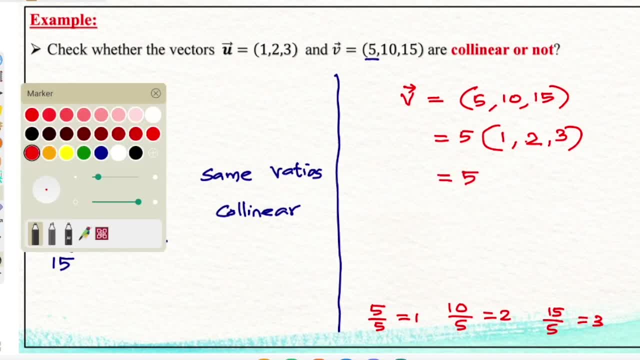 3. 15, we will get. That means 5 multiply. Okay, What is vector 1, 2, 3. This vector, Vector 1, 2, 3, means It is vector u, correct? So 5 times vector u, That means vector v equals. 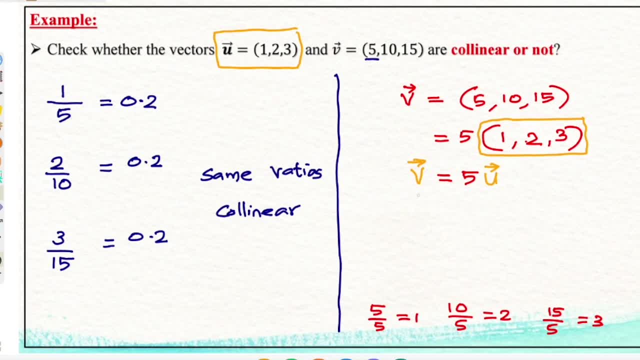 a number multiply vector u. What is the meaning of that one? U and v are collinear vectors, So like this also we can do, Or like this also we can do. Both are Okay, We can use. This is the using the method 1 or condition 1.. Okay, Method 1: I am writing, Or this is: 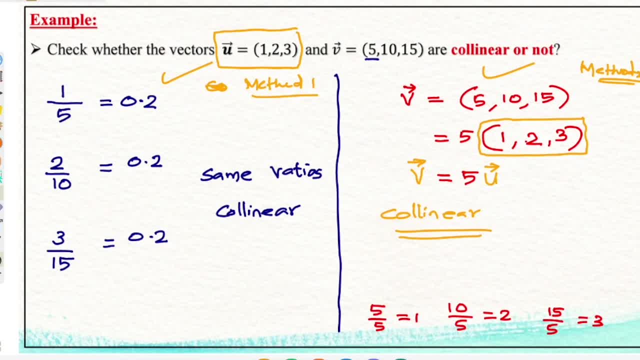 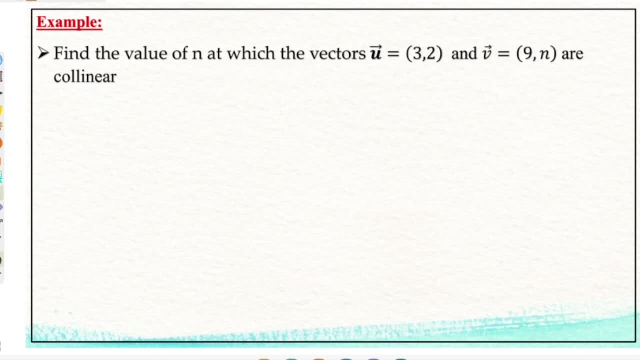 we can do by method 2. Like this also. Okay. So once you understood one of the easier way, you can follow. For example, find the values of n, at which the vectors u and v are collinear. Find the value of n. See, you can see vector v. We have n, is there? What is that n value? That is, 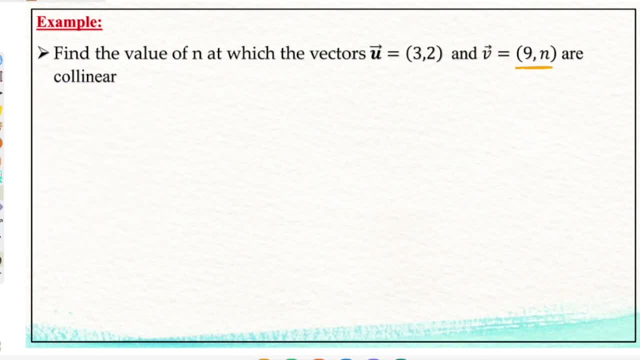 the question here. So we can use the ratio. We can find the ratio X component ratio correct: 3 divided by 9, equal to y component ratio. 2 divided by n: X number in the first vector, 3.. X number in the second vector, 9.. So 3 divided by 9.. 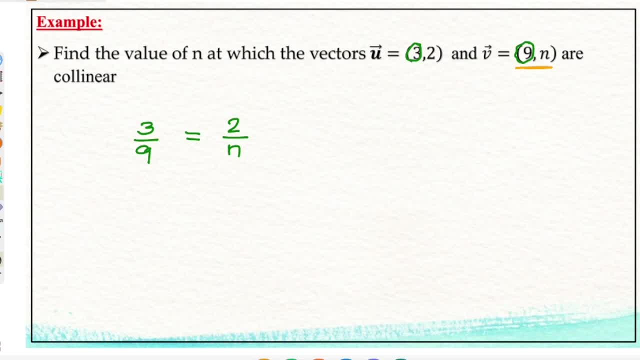 3 divided by 9 equals y component ratio. 2 divided by n. Now, when we are cross multiplying, you will get what is the n number, See 3 multiply n. 3 n equals 9 multiply 2, that is 18.. So 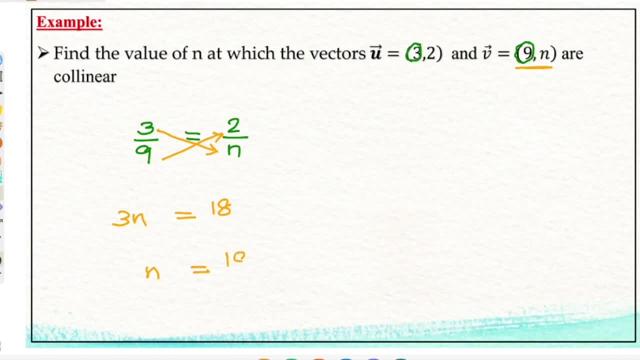 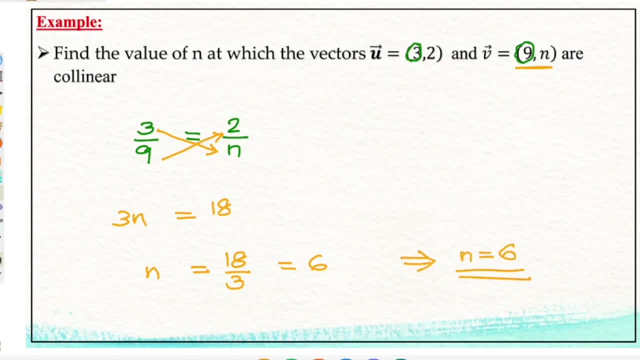 1 or condition 2.. Okay, So we can use the method 1 or condition 2.. Okay, So if n equal to 6, that 2 vectors are collinear. Okay, Condition is collinear. Collinear means the ratios of 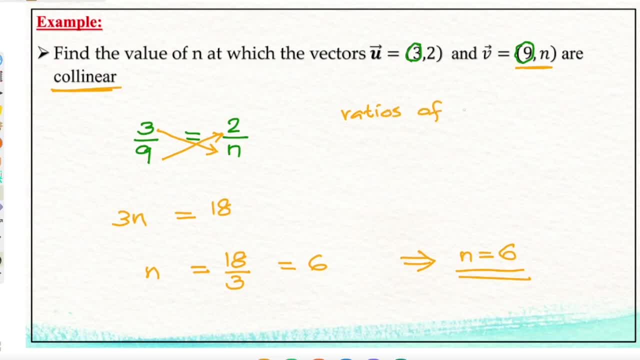 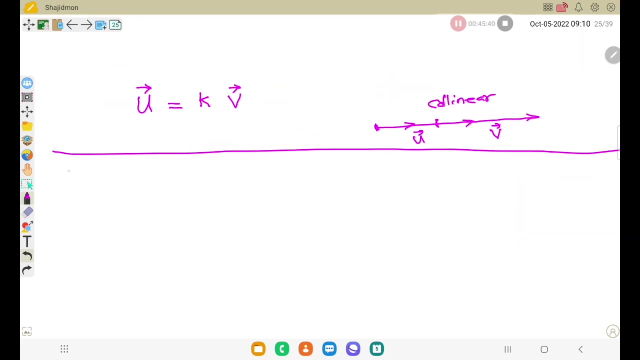 the components. Okay, Ratios of the corresponding components are same. Okay, I hope you understood these questions. Now, another important point: See if you have are taking the vectors from plane and space, for example. plane first, okay, then we need to discuss about space now. we just now we discussed what are the standard unit vector. standard unit vectors. 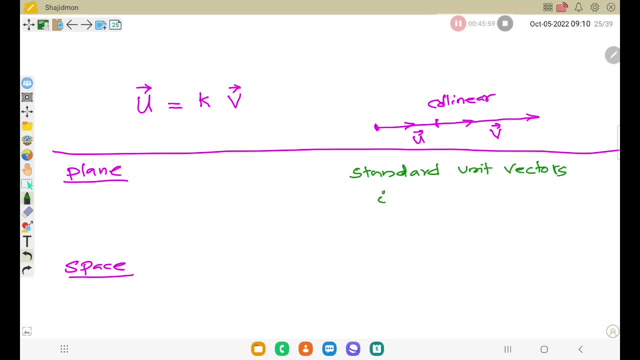 correct in plane and space. what are the standard unit vector? vector i equal to 1, 0. vector j equal to 0 and 1. what are the unit vectors in space? vector i equal to 1, 0, 0. vector j equal to 0 comma. 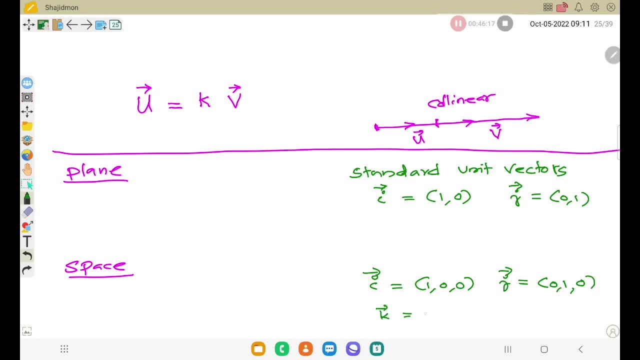 1 comma 0 and vector k equal to 0, 0 and 1. correct. now, if you are taking any vectors in the plane, for example, for example, 6, 8, okay, any other vectors in the plane, we can write this vector as a linear combination. 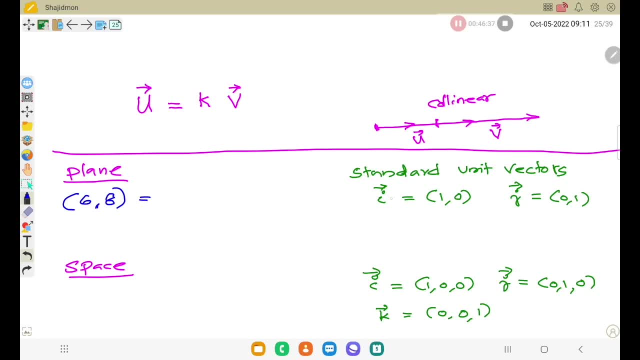 of standard unit vector. that means how to write the this vector in terms of i and j. it is easy. what is the x component here? 6. so 6. multiply x direction unit vector, that is i plus second number y, number y component: 8. multiply the standard unit vector in y direction, that is vector j. 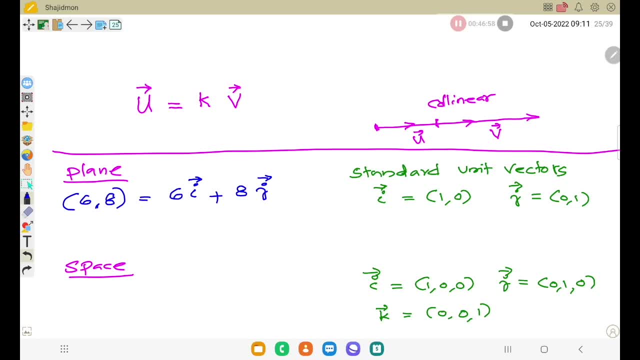 so this is the representation of a vector in terms of standard unit vector. okay, so any vector we can write like this: 6, 8 equal to 6, i plus 8, j. for example, 7, 9 is a vector in plane. how to write that one: 7 multiply i. x number multiply i, y number multiply j. okay, all of you, careful that one same. 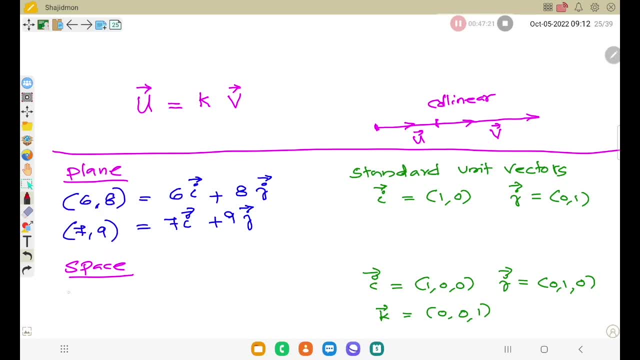 space also. for example, if i am taking a number from the space, space means three number, for example 2, 5, 8. okay, three numbers. how to write in standard unit vector: first number multiply i comma. i component multiply standard unit vector in x direction: i. second number: 5 multiply the standard. 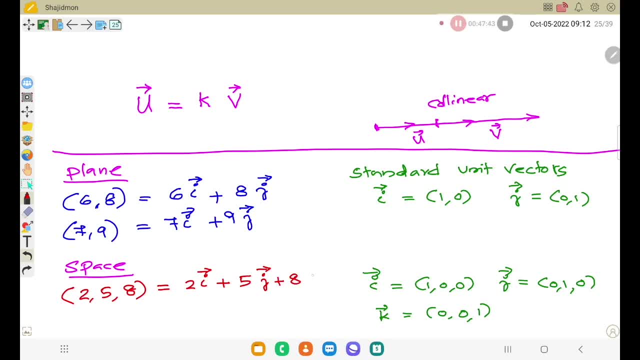 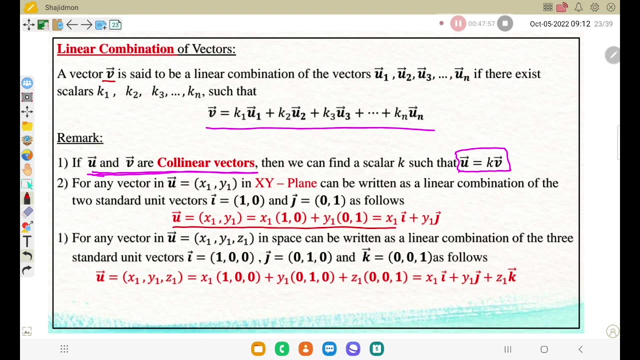 unit vector in y direction, vector j, plus third one, 8 multiply vector k. this is the representation in terms of standard unit vector. okay, so i hope you understood that one. so this is the idea here mentioned: how to write a vector in plane as a linear combination of standard unit vectors. 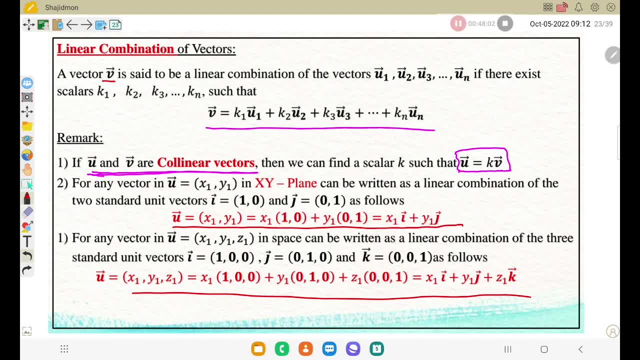 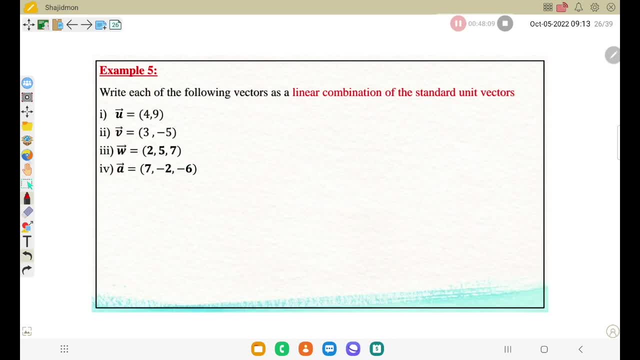 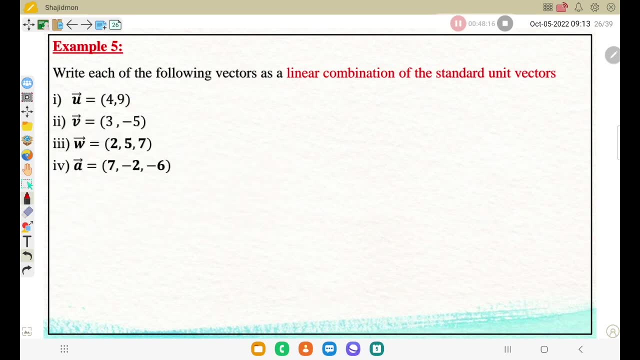 in plane and standard unit vectors in the space. okay, i hope you understood these definitions. now we will do some example here. example 5: write each of the following vectors: write each of the following vectors as a linear combination of standard unit vector. just now we discussed that means this vector we need to write in the unit vector, standard unit vector, for example here: 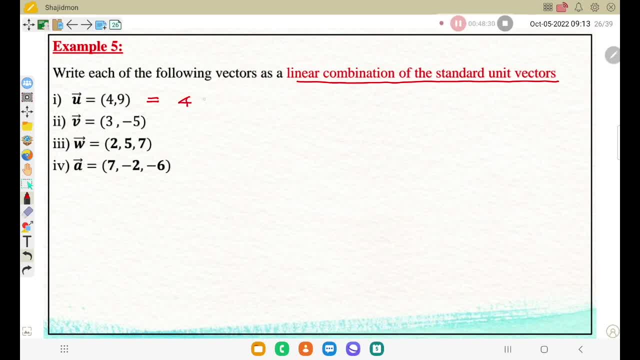 4, 9, 4, 9, 4, 9. how to write 4 times: i is the unit vector in x direction plus 9 multiply j. is the unit vector in y direction, 4 i plus 9, j, x multiply i plus y multiply j. okay, where i means. what is the i vector? 1 comma. 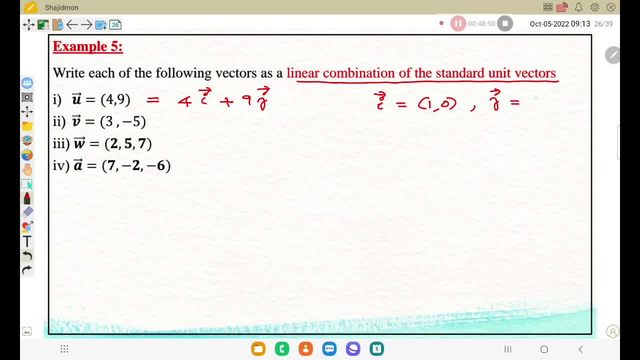 0, because in plane vector j means 0, comma 1 plane vectors same like second example. what is the answer? equals 3 x, x number i plus minus 5 times j. you can write like minus 5 j. okay, i means 1, 0, j means 0, 1 now in space. 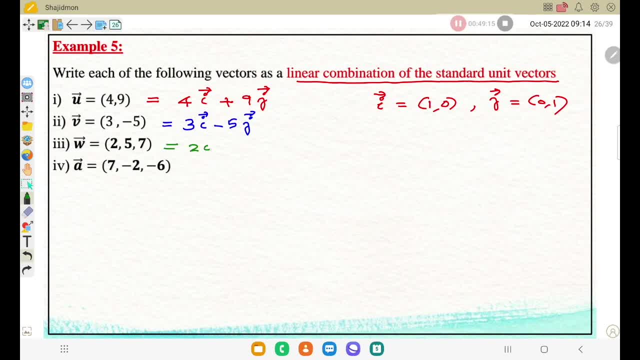 one vector: 2, 5, 7. how to write 2 times i vector plus 5 times j vector plus 7 times k vector correct: where i is vector i means 1, 0, 0 and vector 2 times i vector plus 5 times j vector plus 7 times k vector. 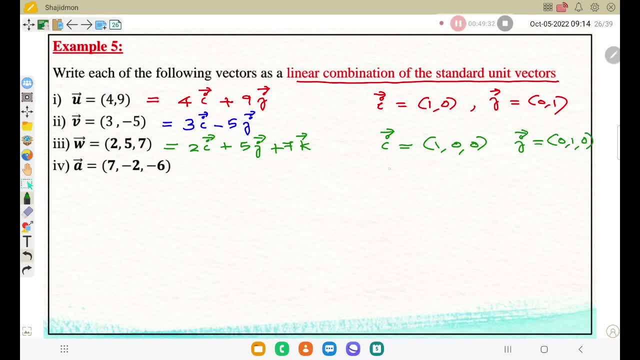 j means 0- 1- 0 and vector k means 0, 0 and 1. okay, so i hope you understood how to write a vector as a linear combination of standard unit vectors. now here this one: first number: 7, multiply i minus 2 times vector j minus 6 times vector k, where i and j and k we need to mention because 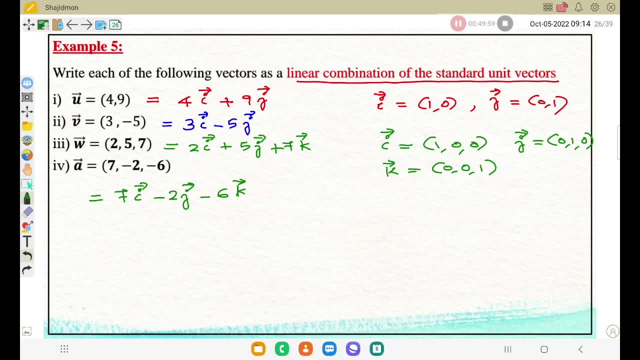 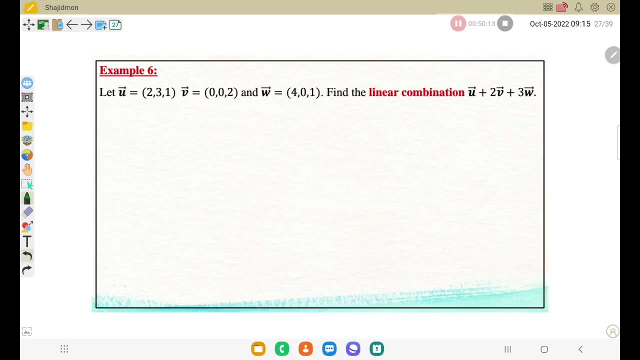 plane and space. it is different, so we need to write what is i, what is j and what is k. so i hope you understood the ideas in the first section, 1.1, correct. now we will go to the questions, exercise questions one by one from all these ideas. okay, yeah, before that we will do one example. 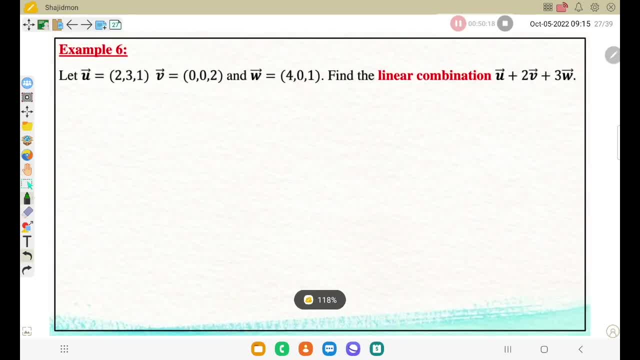 this question. then we will go to exercise after, for example, let vector u equal to 2, 3, 1, vector v equal to 0, 0, 2 w you equal to 4, 0, 1. find the linear combination. that is the question. linear combination, what linear? 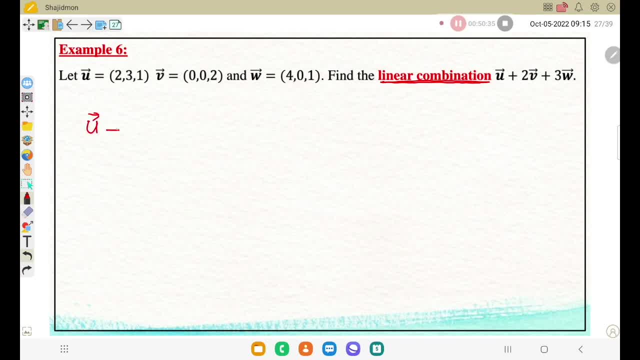 combination. we need to find vector u plus 2 times vector v plus 3 times vector w. what is this value, this linear combination we need to calculate? i hope you know that one see vector u means. what is that? 2, 3, 1 plus 2 times. what is vector v: 0, 0 and 2 plus 3 times vector v: 0, 0 and 2 plus 3 times? 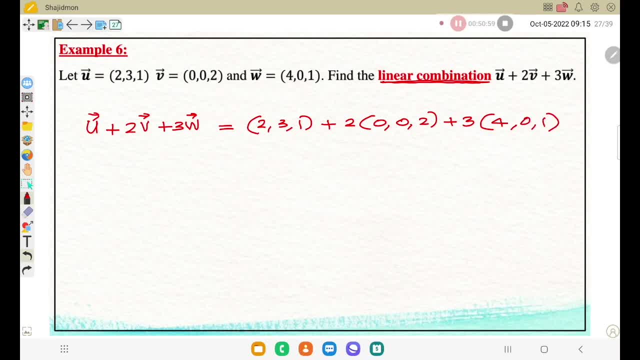 what? what is vector w, 4, 0 and 1? equal 2, 3, 1 plus. you know how to multiply 2 times this vector, correct each number. what is this answer number. so we will get 2 multiplied 0. to multiply 0, 2 multiplied 2 plus 3 multiplied 4, 12, 0 and 3. now add all these numbers equal to x嫩 with the 1 and 2fl нес. and the second factor to multiply 2: xстран 위ов. change 2 with the 2x, nowhere. so we will get 2 log x, энергicwei, 2 x, 21 x, 2 rises. that is, if you multiply each number two times, this vector correct each number. multiply without said number. so we will get you multiply estrena next two times, three times, 2 times two times. 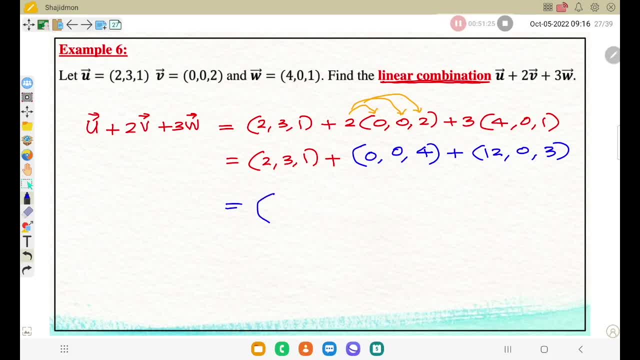 3. now add all these numbers, equal vector first numbers: add 2 plus 0 plus 12, 14, 3 plus 0 plus 0, 3, 1 plus 4 plus 3, 5 plus 3 is 8, so this is the linear combination: u plus 2, v plus 3 w. 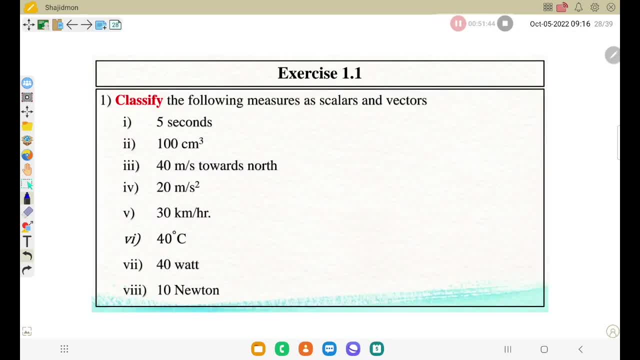 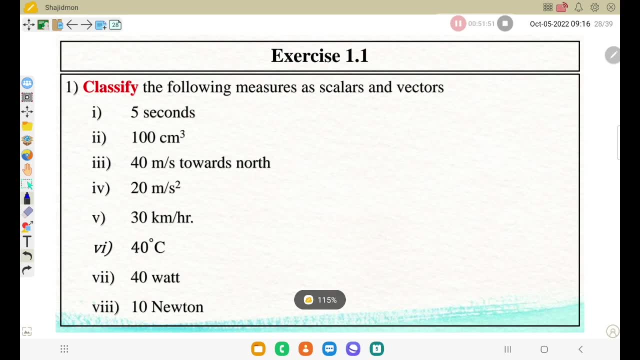 clear. okay, now we will go to the examples. exercise questions from these ideas. exercise 1.1: first question: classify, okay, the measures: scalars or vector. okay, which of the following are scalars and which of the quantities are vector quantities? this is the first question: scalars and vectors. 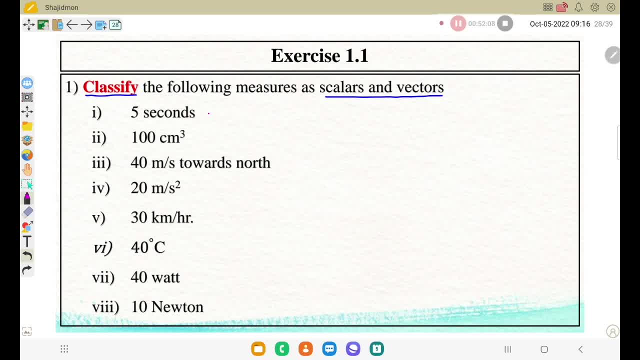 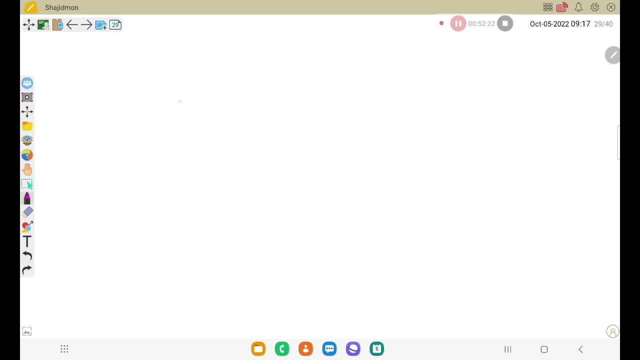 for example, the first one, 5 second, 5 second means it is time. correct time means which quantity. it is a scalar quantity, correct now, 100 centimeter cube. what is that 100 centimeter cube? before that you can see, for example, centimeter, centimeter. 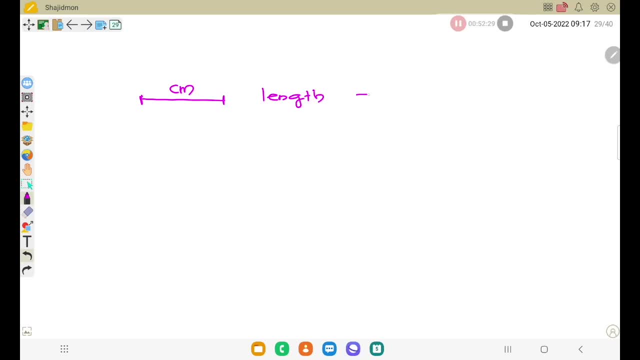 means what length? correct length means it is scalar quantity. now, if you are taking, for example, like this rectangle, what is the area it is calculating? length multiply width. correct length multiply width, so centimeter square, for example, this is centimeter, this is in centimeter and centimeter. 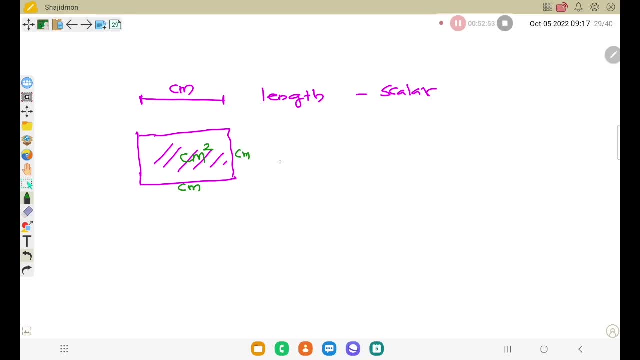 square, or meter square or feet square, like that. so this is area. area means always a scalar quantity: centimeter square- okay, now same. for example, if you are taking a cube like this: okay, if you are taking a cube like this, okay, now in the cube, this is centimeter. for example, this is centimeter, this. 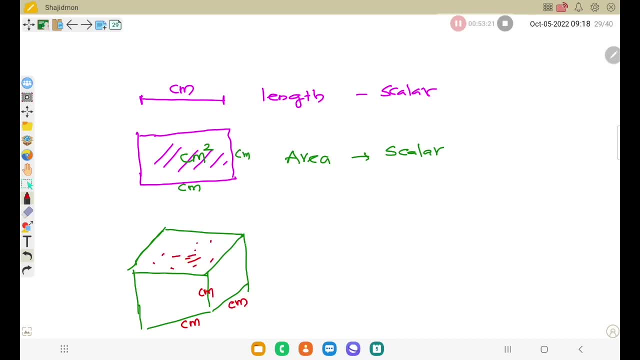 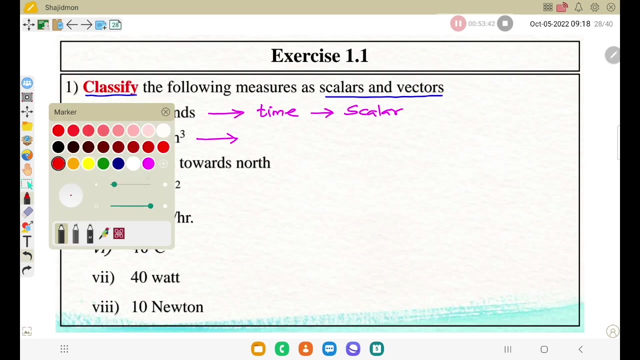 is centimeter. so what will be the oleum? oleum means centimeter cube, centimeter cube, okay. so oleum, oleum also a scalar quantity, okay. so keep in your mind centimeter or meter, whatever the unit. so length, area and square means area, cube means oleum, so we can go to this: one hundred centimeter. 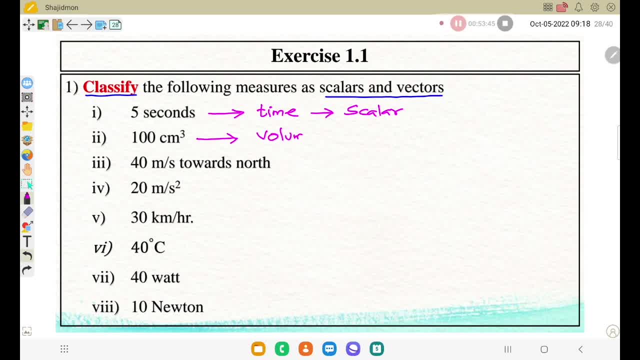 cube. cube means oleum, oleum means it is a, a scalar quantity. now, 40 meter per second towards north. 40 meter per second always when we are telling speed or velocity correct. now, speed with the direction we are calling velocity. so here, 40 meter per second means speed towards north, means direction. so it is velocity. velocity is a vector. 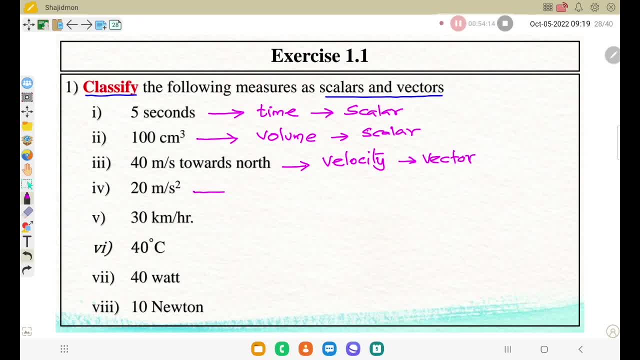 quantity now: 20 meter per second square. meter per second square means it is the unit of acceleration. so 20 meter per second square means it is acceleration. acceleration means it is a vector quantity, correct. now again. 30 kilometer per hour, 30 kilometer per hour. in a car meter you can see your speed: 30 kilometer per hour, 120 kilometer per hour, like so. 30 kilometer per hour means it is speed. there is no direction here. so speed speed means it is scalar quantity. so 20 meter per second square means it is acceleration, acceleration. acceleration means it is a vector quantity, correct. now again. 30 kilometer per hour, 30 kilometer per hour. in a car meter you can see your speed: 30 kilometer per hour, 120 kilometer per hour, like so 30 kilometer per hour means it is speed. there is no direction here. so speed. speed means it is scalar quantity. so 20 meter per second square means it is acceleration, acceleration, acceleration, acceleration means it is a vector quantity, correct. now again. 30 kilometer per hour, 30 kilometer per hour, 30 kilometer per hour. in a car meter you can see your speed: 30 kilometer per hour, 120 kilometer per hour, like so. 30 kilometer per hour means it is speed. there is no direction here. so speed speed means it is scalar quantity. so 30 kilometer per hour means it is speed there is. 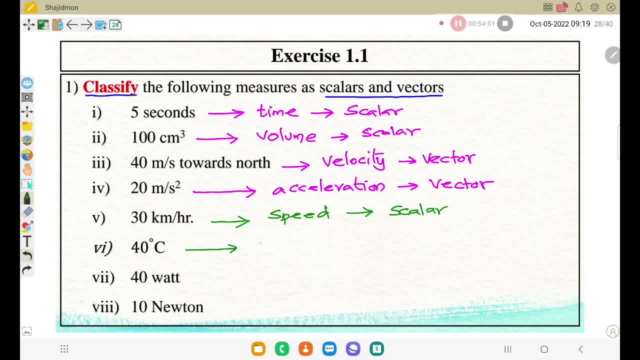 Okay, Now 40 degree Celsius. Degree Celsius means temperature, Temperature. Temperature is a scalar quantity. 40 watt, Watt means power. One electric bulb, How much watt? 40, something, Something different, 40 watt. So 40 watt is a power unit. Power means it is a scalar quantity. Now, 10 newton, Newton is the unit of force. Right, Force means it is a vector quantity. So these are the classification of this example. Whichever, Okay, What are the quantities of vector and scalars? 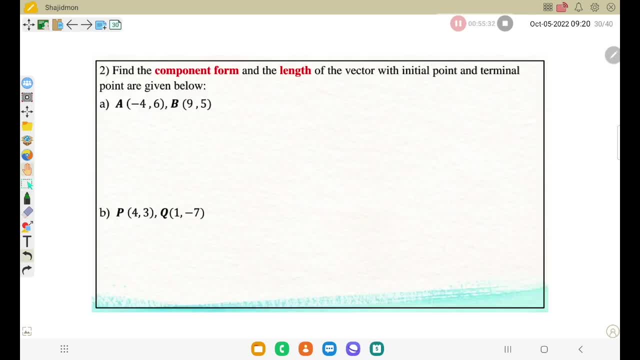 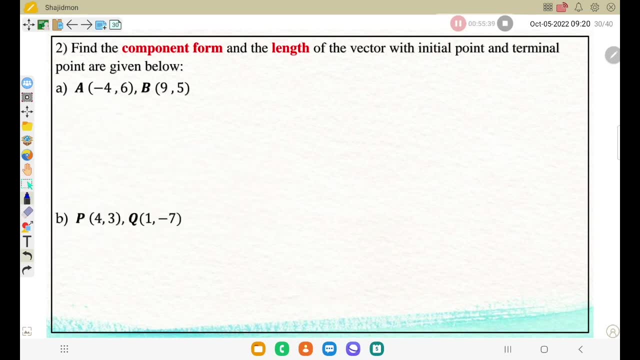 Now we will go to the second question: Find the component form and length of the vector. Find the component form and length of the vector. Find the component form and length of the vector. Initial point, terminal points, are given Component form we discussed We need to calculate x value, y value. Length means we need to calculate the magnitude of v or absolute v. Length of the vector. 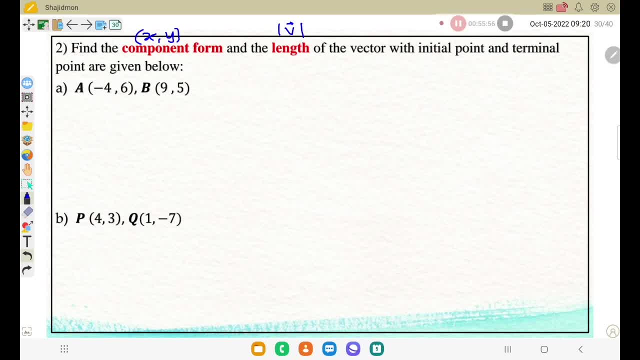 So first we do the component form. Okay, So starting point A minus 4 comma 6.. That vector, ending point B, 9 and 5.. Okay, So what is the component form? x1, y1, x2, y2.. Correct, Now what is the component form we studied? Vector AB equals x2 minus x1 comma, y2 minus y1. So what is x2 minus x1? x2 number is 9.. Minus x1, number is minus 4.. 9 plus 4.. y2 minus y1.. 5 minus 6.. 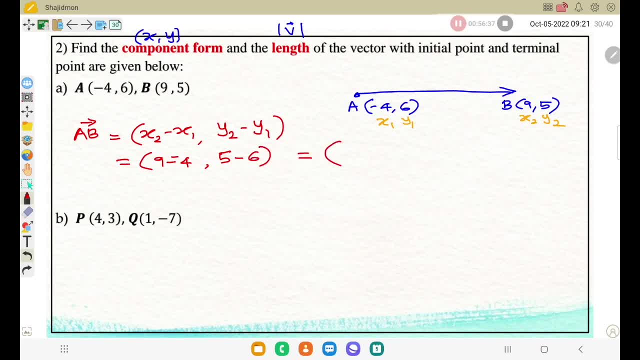 So what answer you got? Okay, You can check it: 9 plus 4.. That is 13.. 5 minus 6 means minus 1.. Correct. Now we will go to the second question. What is the magnitude? Length, Magnitude of vector AB equals. What is the rule? Magnitude of vector AB is root of x square plus y square. 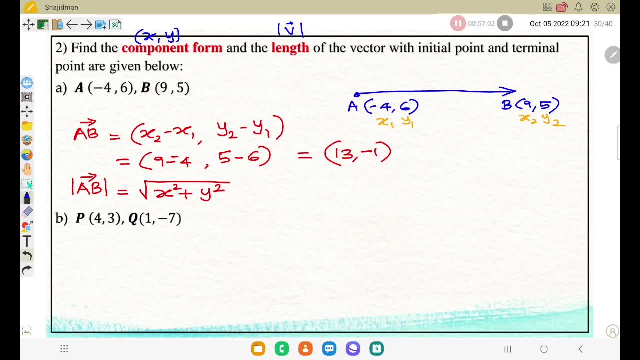 x means the x component. What is the x component here? and y component? x component of vector AB, That is 13.. y component of vector AB is minus 1.. So how to calculate Root of 13: x component square plus y component is minus 1 power, 2. Correct. 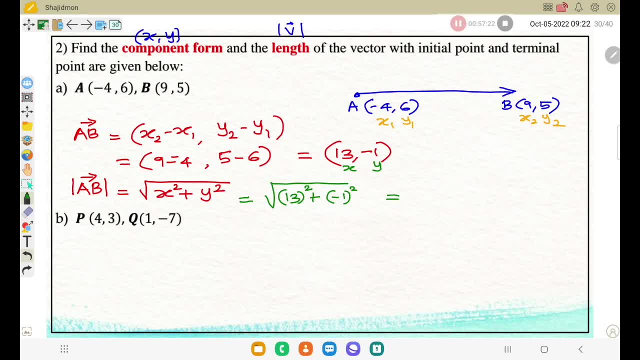 Now you can check that number 13, power 2. That is 169.. 169 plus 1.. Correct, So root of 1, 7, 0.. Whatever the number, Okay, Root of 1, 7, 0.. 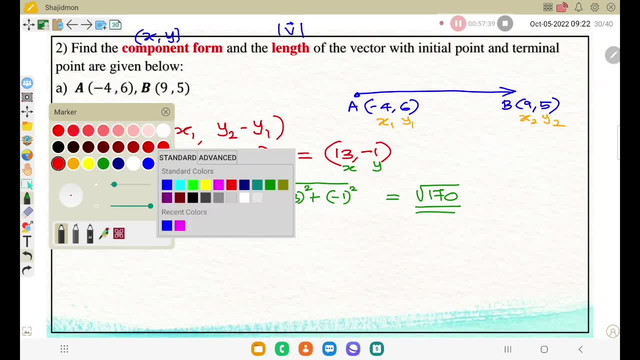 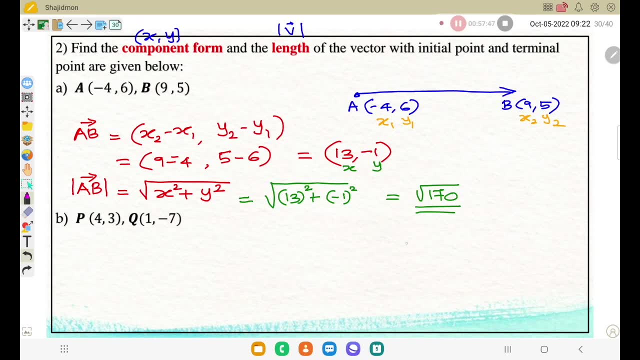 Now we will go to the second question. That is P equal to 4, 3.. Q equal to minus 1.. Sorry, 1, minus 7.. Vector P: Q: Correct: P is 4, 3. Q is 1, minus 7.. So this is x1, y1, x2, y2.. 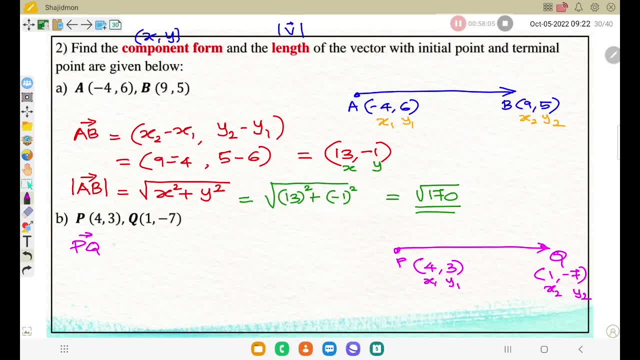 So vector P, Q, We need to calculate That is x2 minus x1,, y2 minus y1.. What is x2? x2 is- We can get it 1, minus 4, y2 minus y1.. Minus 7, minus 3.. So we will get the answer. 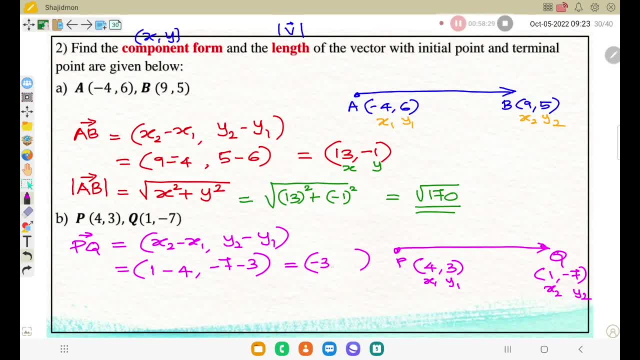 Audit pair: 1, minus 4 means minus 3.. And minus 7, minus 3 means minus 10.. Hope you understood. Now we can calculate Absolute of vector P. Q equals root of same rule: x2 plus y2.. x2 means minus 3 square plus y2.. That is minus 10 square. So minus 3 square means 9.. 10 square means 100.. So what is the number Root of 1, 0, 9.. Hope you understood these questions. 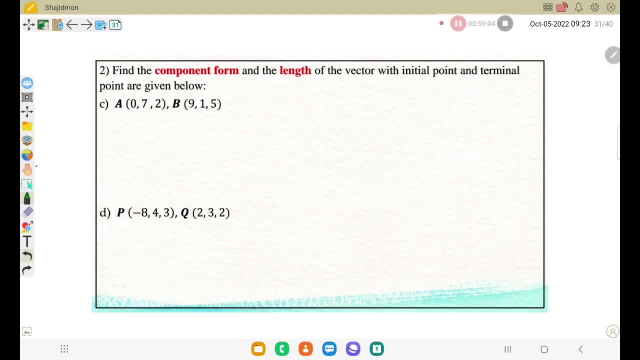 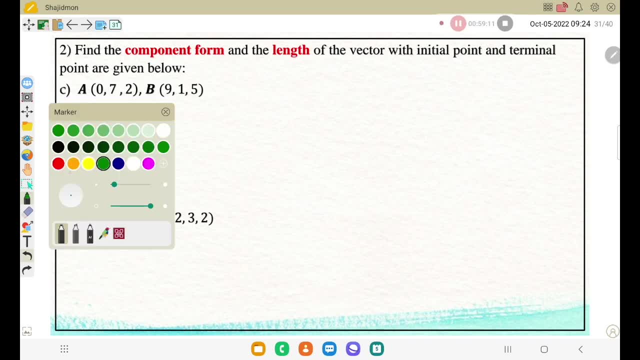 Now question number 2.. C part, Same model 3D In space. For example A is the number 0,, 7,, 2. And B 9,, 1,, 5.. Find the component form. Component form means x, y, z. We need to calculate Because in space And after that magnitude of that vector Correct. So here x1 is 0,, y1 is 7,, z1 is 2.. x1, 9.. Sorry, x2, 9.. y2, 1.. z2, 5.. So we will go to the calculation. 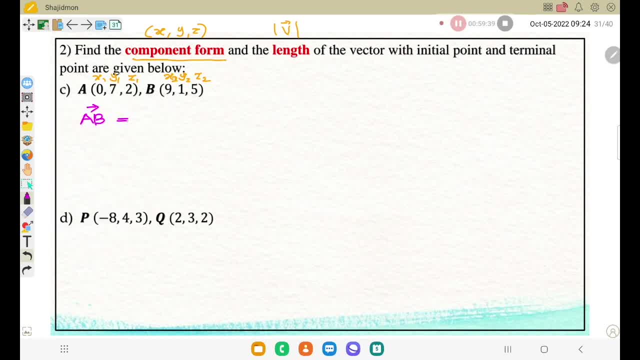 Vector AB equals. So what was the idea? x2 minus x1.. y2 minus y1.. z2 minus z1.. Correct Apply the number. What is x2 minus x1?? 9 minus 0.. y2 minus y1.. 1 minus 7.. z2 minus z1.. 5 minus 2.. 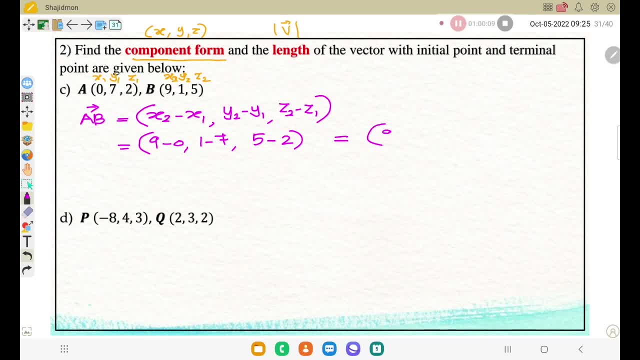 Correct. What will be the answer? 9 minus 0.. 9. 1 minus 7. Minus 6.. 5 minus 2. 3. Okay, So in that question what is the x component? 9. y component Minus 6. z component, That is 3. Correct. 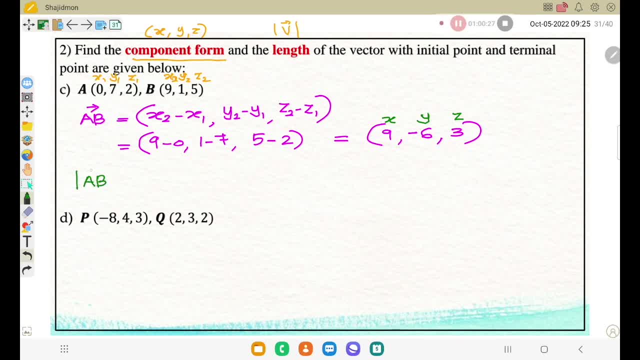 Now we need to calculate what is. magnitude of vector AB equals. Magnitude of the vector AB equals. So what was the rule? Root of In space means x power 2 plus y power 2 plus z power 2.. Correct, So equal root of What is the x number: 9 power 2 plus y means minus 6 power 2 plus z means 3 power 2.. 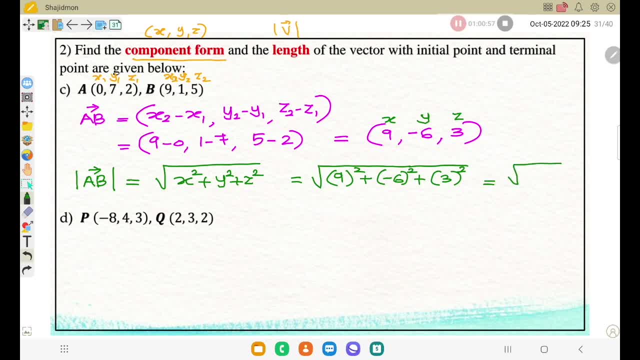 You can check this number in your calculator: 9 power 2 means 81.. Correct: 6 power 2 means 36.. 3 power 2 means 9.. Root of 126. We will get root of 126. I hope it is clear to you. 3 root 14.. Otherwise, 11.2, approximately 11.2.. Okay, Now go to the next question. 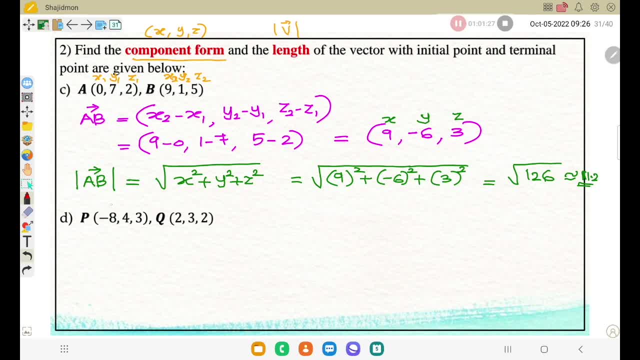 P, Q. P is given, Q is given. So in P, x1 number is minus 8. y1, 4.. z1, 3.. x2, 2.. y2, 3. z2, 2.. So we need to calculate what is vector. P. Q equals x2 minus x1.. 2 minus minus 8.. y2 minus y1.. 3 minus 4.. z2 minus z1.. 2 minus 3.. Rule is same. before we wrote. 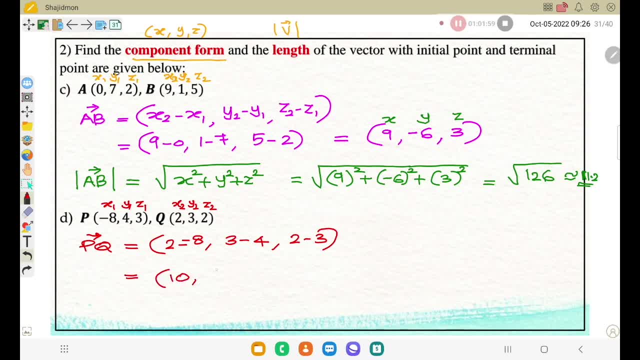 So 2 plus 8 means 10.. 3 minus 4 means minus 1.. 2 minus 3 means minus 1.. Now, absolute of the vector P Q. Absolute of vector P Q equals root of x component 10 power 2 plus y component minus 1 power 2 plus z component minus 1 power 2.. 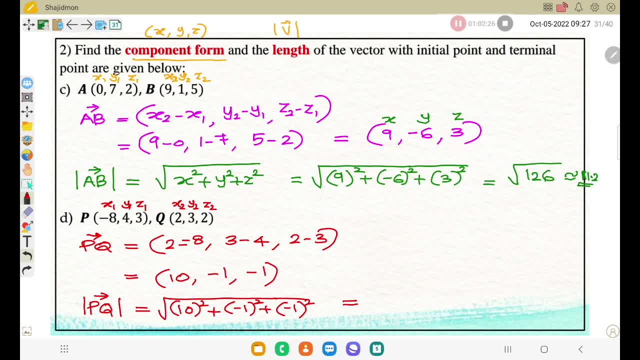 So we can check 100.. 10 square is 100.. Plus 1: power 2.. Minus 1 power 2 is plus 1.. Minus 1 power 2 is 1.. So root 1, 0.. 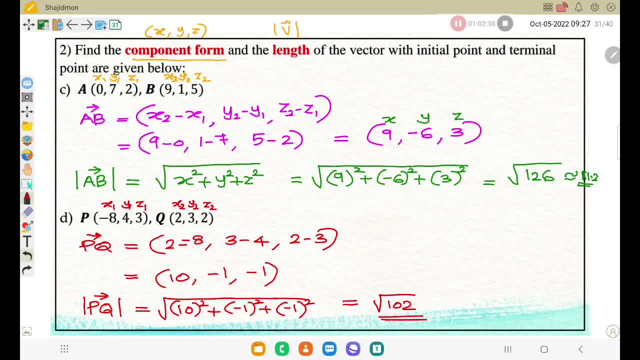 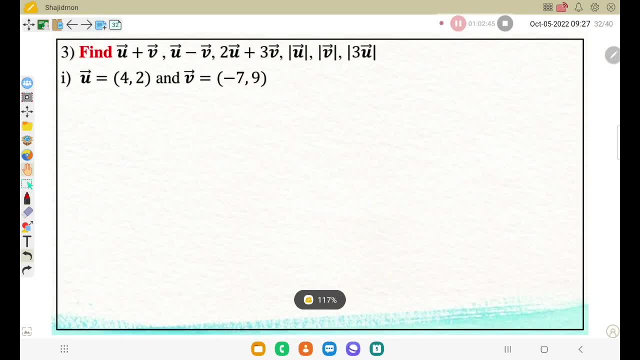 2 is the answer. Hope you understood this question. Component form and length Correct. Okay, Now the second third question: Find u plus v 2, u minus v. 2u plus 3v. absolute v. absolute u absolute 3u. 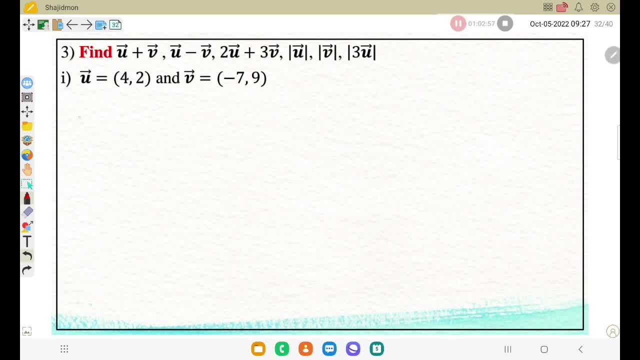 u vector is given and v vector is given. So we will do one by one First part of the question: u plus v vector. So we need to calculate What is u vector 4 comma 2.. Plus, what is v vector Minus 7 comma 9.. 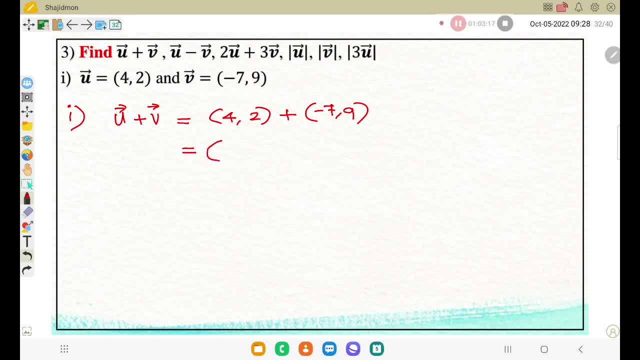 You know how to add these two X number. add 4 plus minus 7.. Correct, 4 plus minus 7.. That means minus 3.. Now 2 plus 9.. That is 11.. So we will go to u plus v. Now we will go to the calculation. 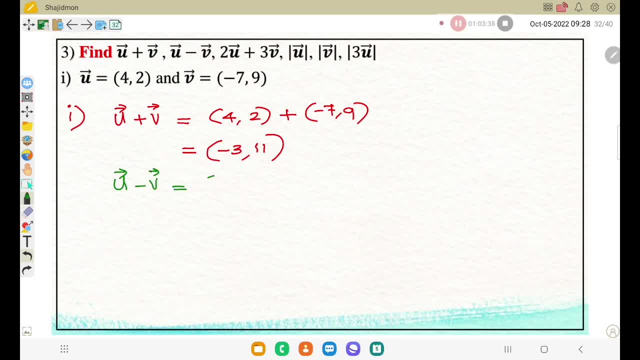 Minus vector v. What is u minus v? u means 4, 2.. Minus v means minus 7 and 9.. So what? we will get it 4 minus minus 7.. That means 4 plus 7.. 11, 2 minus 9.. Correct: Minus 7.. 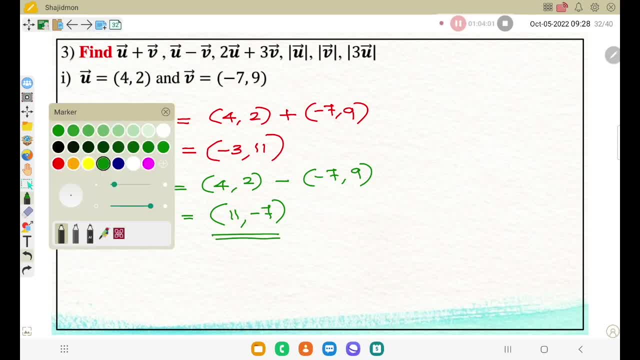 Now what is the third question? We can calculate the third one. We can do: 2 vector u plus 3 times vector v. that means 2 times what is vector u, 4 comma 2, plus 3 times what is vector v minus 7 comma 9. you know how to multiply that one correct multiply here, multiply. 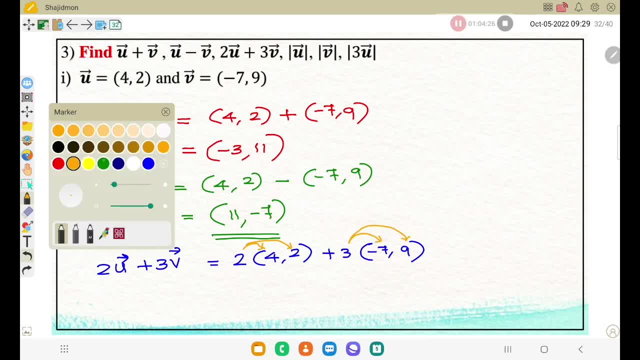 here. same multiply here and multiply here. so what we are getting equals 2 multiply 4, 8, 2 multiply to 4 plus 3, multiply minus 7 minus 21, 9 multiply 3, 27. now add that to equal the vector. so first, 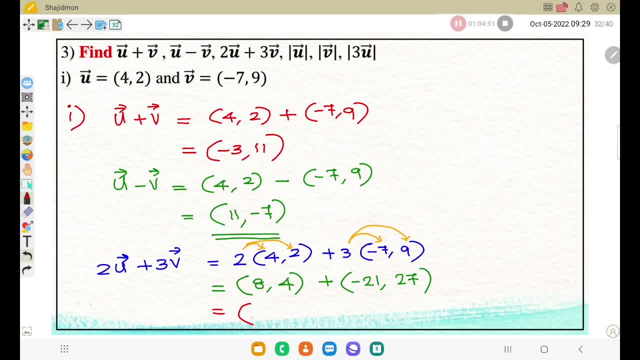 one, 8 plus minus 21, minus 13, then 4 plus 27, correct 31. so this is the vector 3, 2 u plus 3 v. now now absolute of u, absolute of v. that question we need to do now, okay, so first we do what is. 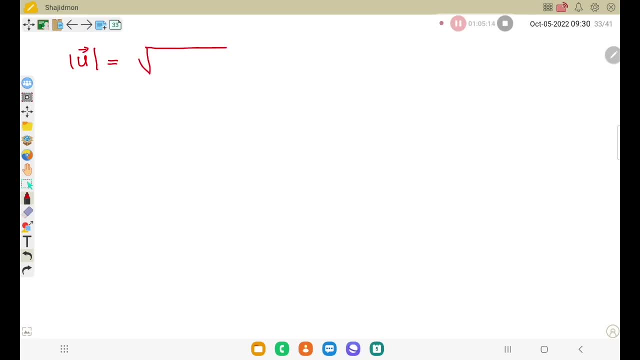 absolute of vector u equal. what was the rule root of? correct here the point is in plane root of x square plus y square. so what is the x value in vector u? equal 4 power 2 plus 2 power 2, correct because you know x number 4. 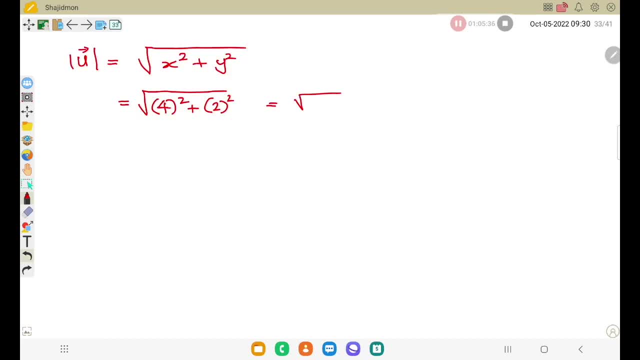 y number is 2, so you can check by calculator: 4 power 2 means 16, 2 power 2 means 4. root 20. now absolute of vector v equal. okay, again, root of x square plus y square x means minus 7 power 2. 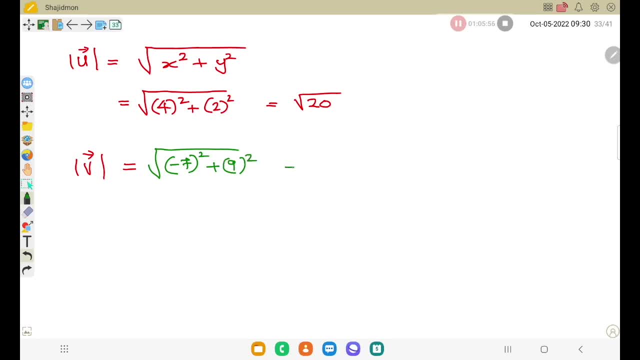 y means 9 power 2- you can check the number- 7 power 2 means 49 plus 9 power 2 means 81. so root 130 point number. also, you can write now absolute 3 times vector u. this is the next one, 3. 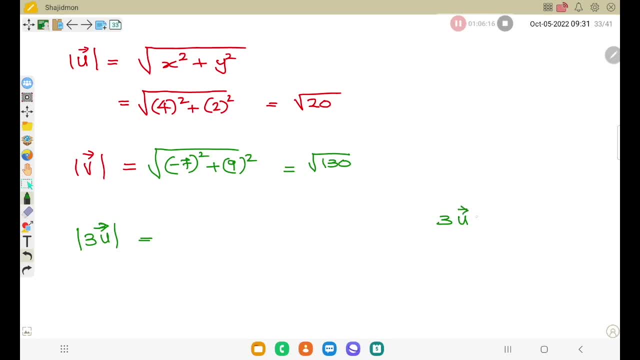 times vector u. so first we can calculate what is 3 times of vector u. we can do simply like this: so 3 times vector u means 4, 2, so 3 multiply 4, 2 means 3 multiply 4, 12 comma. 3 multiply 2 is 6, so we can. 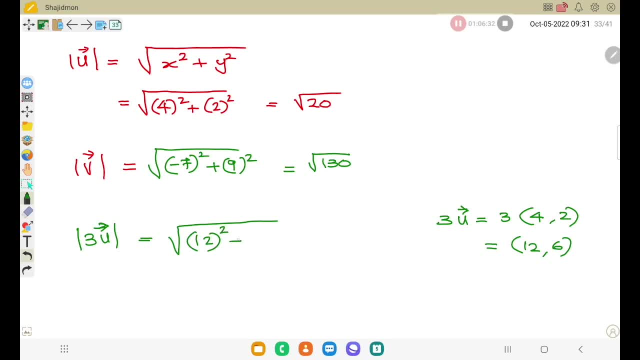 do root of 12 power 2 plus 6 power 2 correct. you know what is 12 power 2, 144. so root 144 plus 6 power 2 means 36. so finally we will get the answer: 144 plus 36, 180. root 180 correct. 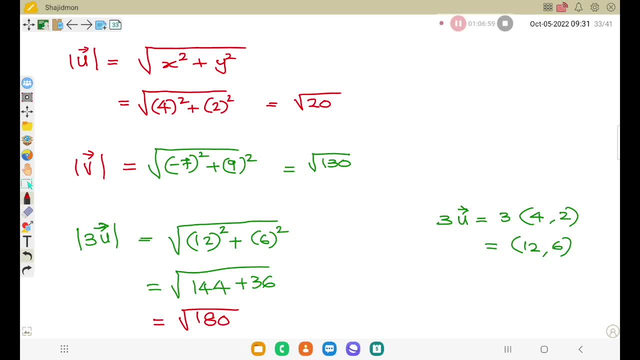 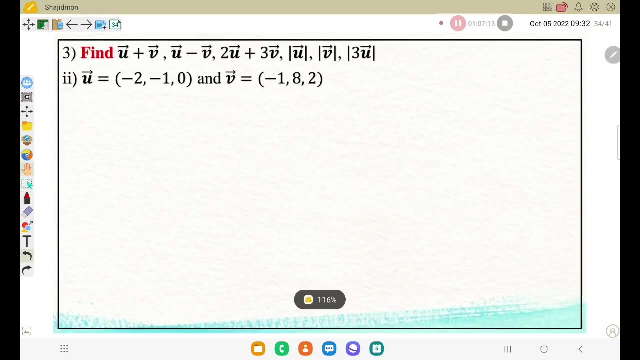 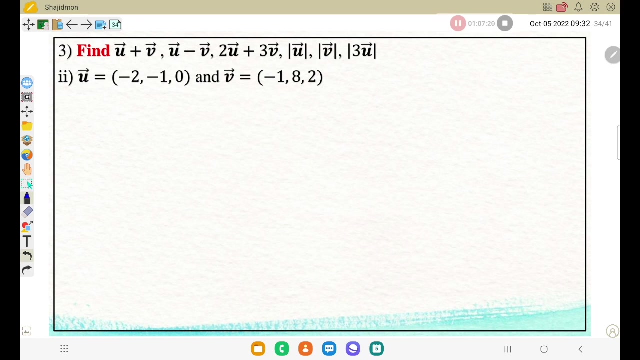 you can write the point number also like 13.4, approximately, okay, 13.4. hope you understood this question. what to do? okay now. question 2, 3, 2. question number 3, second part. now you can practice. okay, as much you want. so vector u plus v: first calculate vector u. 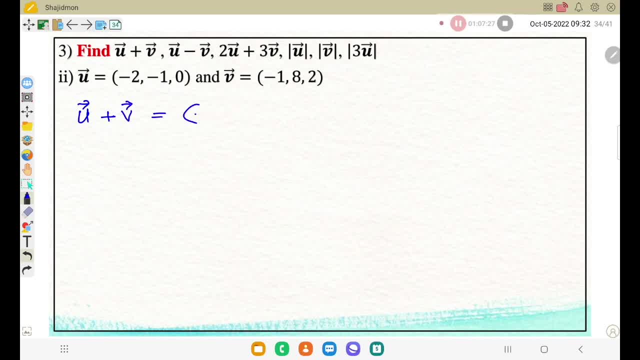 plus vector v, equal what is vector u minus 2 minus 1, 0 plus minus 1, 8 and 2. so add the number first, minus 2 plus minus 1, minus 3 minus 1 plus 8, 7, 0 plus 2, that is 2 correct. 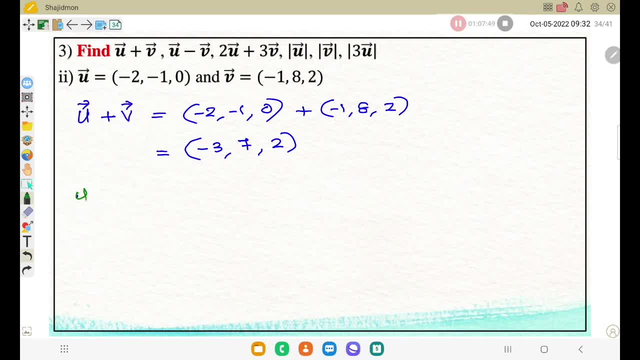 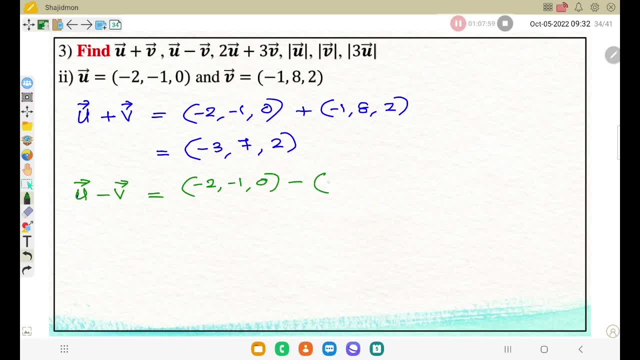 minus 1, 0, minus vector v means minus 1, 8, 2.. So when we are getting subtracting minus 2, minus minus 1,, correct Minus 2, minus minus 1, that is minus 2 plus 1, minus 1, minus 1,. 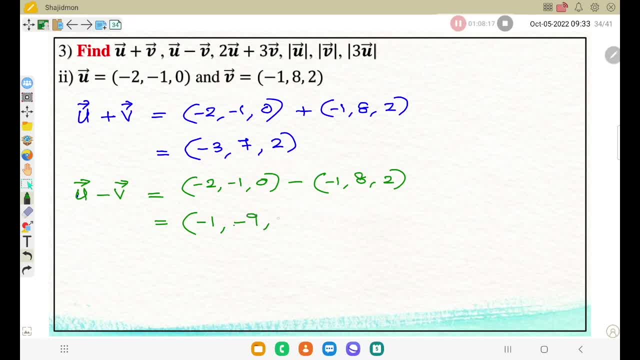 minus 8, minus 9, 0, minus 2, minus 2.. Now 2 times u vector plus 3 times v vector. So we can write 2 times what is the u vector Minus 2, minus 1, 0, plus 3 times v vector. 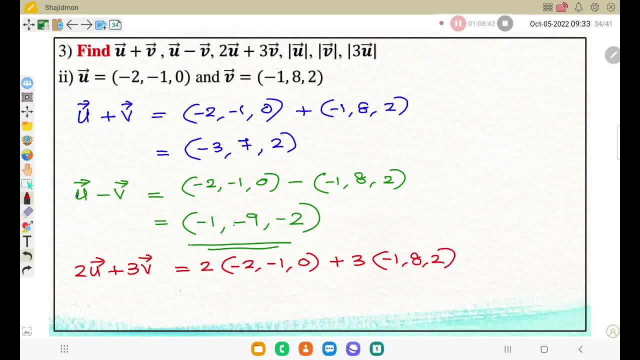 minus 1,, 8 and 2.. Simplify First: 2 multiply minus 2, minus 4,. 2 multiply minus 1, minus 2,. 2 multiply 0,. 0 plus 3 multiply minus 1, minus 3,. 3 multiply 8, 24,. 3 multiply 2, 6.. Now you can add these two vectors: 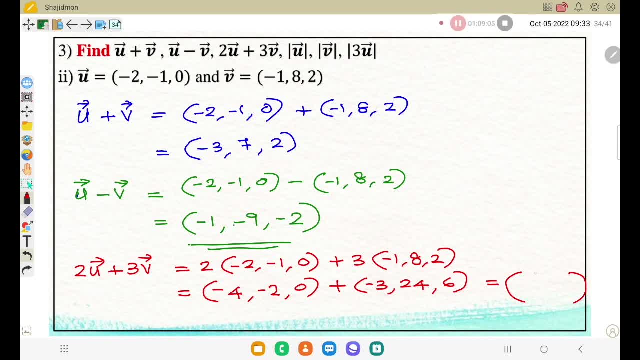 you will get the number, For example, minus 2 plus minus 3, sorry. minus 4 plus minus 3, minus 7, minus 2 plus 24.. That means 22.. Then minus 2,- sorry, 0 plus 6, that is 6.. So this is the 2u plus 3v. 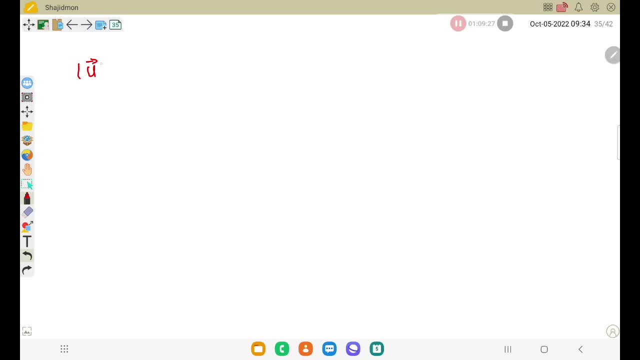 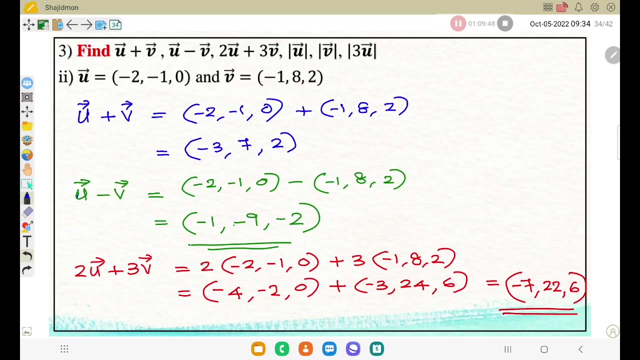 Now we will go to what is vector u magnitude and what is vector v magnitude and what is vector 3u magnitude, correct? So first we will do u magnitude root of x square plus y square plus z square, correct, Because the point in space, So u vector x component, what is? 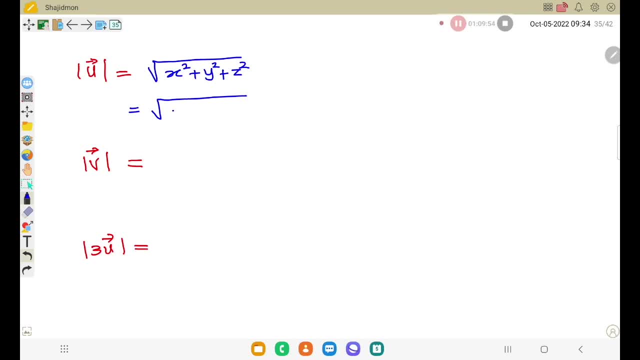 the u vector x component. Root of minus 2 power 2 plus y component. minus 1 power 2 plus 0 power 2.. That means root of 4, 2. power 2 means 4, plus minus 1. power 2 means 1, 0. 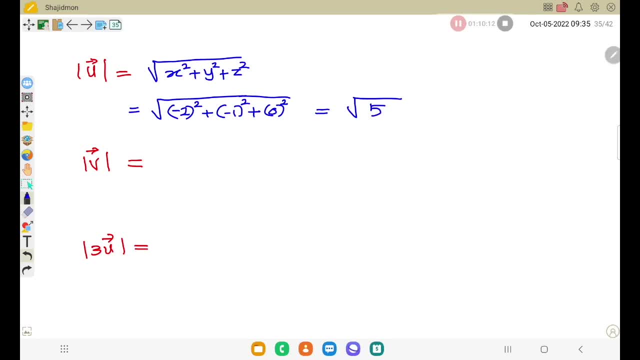 power 2 means 0,, so root 5.. Now we calculate what is the absolute of v, So root of same x square plus y square plus z square. Here the vector minus 1, 8, 2.. So minus 1 power 2 plus 8, power 2 plus. 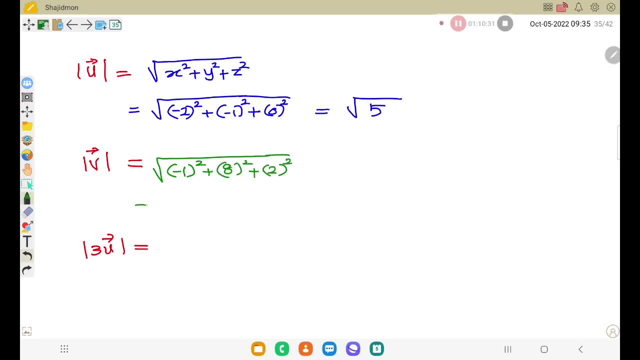 2, power 2,. okay, We can check the calculator: Minus 1, power 2 means plus 1, 8 power 2 means 64,, 2 power 2 means 4.. So you will get root 69.. 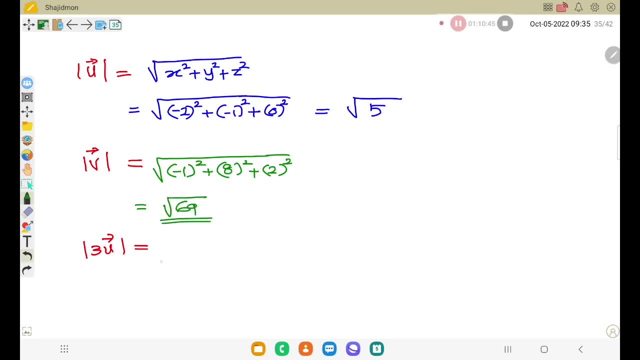 Okay, Now magnitude of 3 times vector u correct. So first check 3 times of vector u. 3 times what is vector u Minus 2, minus 1, 0. So you can multiply 3 minus 2,, multiply minus. 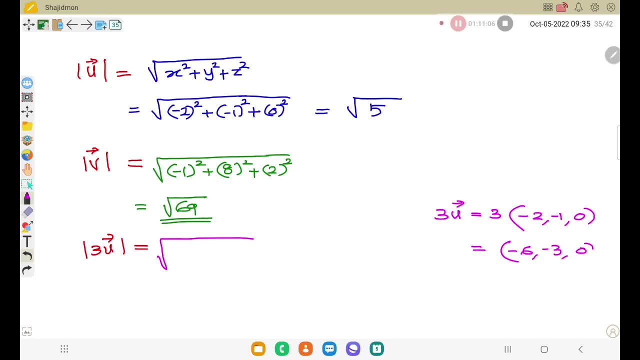 2, minus 6, minus 3, 0.. So minus 6: power 2 plus minus 3: power 2 plus minus 3: power 2 minus 0, power 2.. That means 6, minus 6, power 2 means 36.. 3 power 2 means 9.. So root. 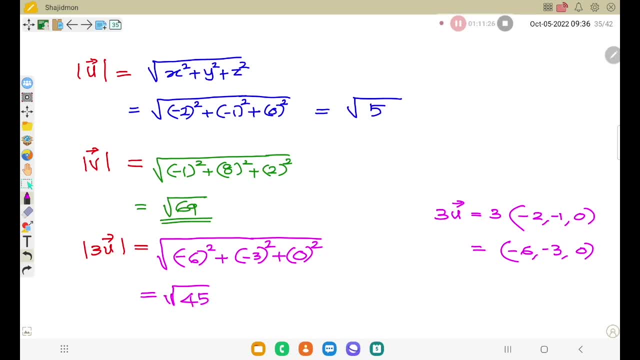 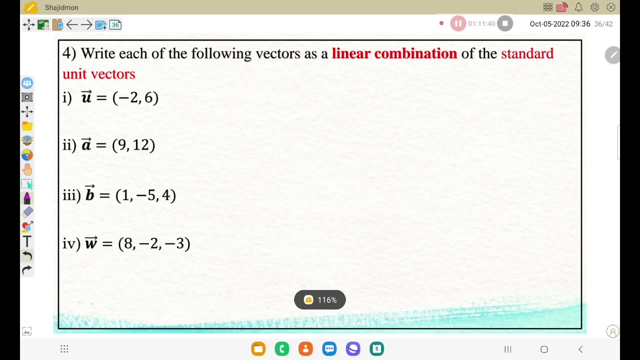 45. Root of 45. You can write the point number also, So root 45.. Hope you understood this type of questions. Now go to the next one, question number 4.. Write the following vectors as a linear combination: 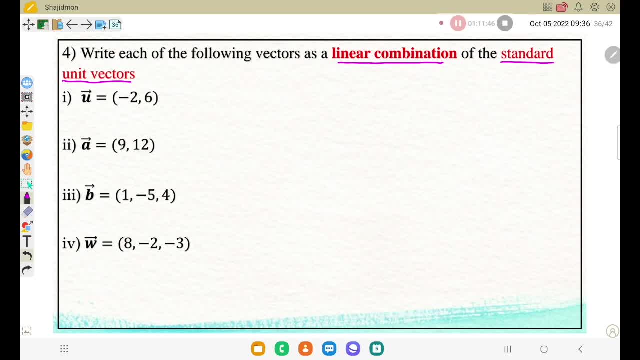 of standard unit vector. You know what are the standard unit vectors. correct Vector i means 1, 0. Vector j means 0, 1.. Standard unit vectors in plane Space. what are the unit vector? Vector i equals 1, 0, 0.. Vector j means 0, 1, 0.. And vector k means 0, 0,. 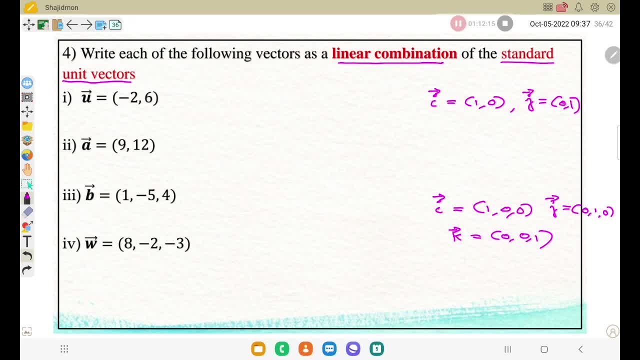 1. So we need to write these vectors as a linear combination of standard unit vectors. That means these vectors For example: first one Minus 2, 6. X component is minus 2. Y component is 6.. So x component, that is minus 2, multiply i vector plus y component, that is 6, multiply. 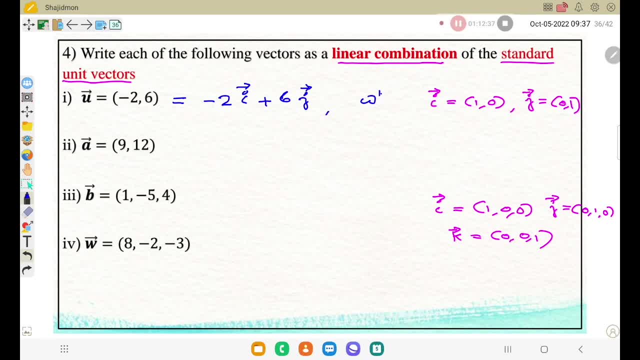 vector j, Where vector i means 1, 0.. Vector j means 0, 1.. Don't forget to write that. vectors, okay, You know space vector and plane vectors. Now second one, 9, comma 12.. So 9 multiply i vector plus 12 multiply j vector, It is 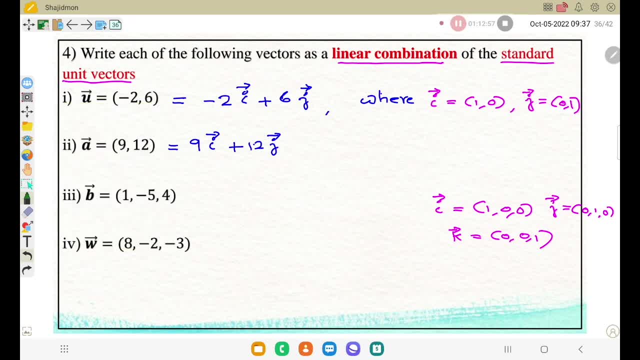 easy to write the vector in standard unit vectors Now in space 1 vector 1 minus 5, 4.. 1 minus 5, 4.. So 1 multiply i vector minus plus. minus means minus 5 multiply. 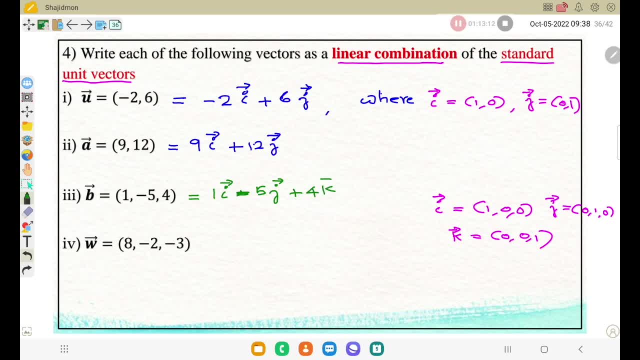 j vector plus 4 multiply k vector, Where i vector means 1, 0, 0. And j vector means 0, 1, 0. And k vector means 0, 0, 1.. Okay, We need to mention that one. Now, third, one, last one: 8 multiply i plus minus 2 multiply. 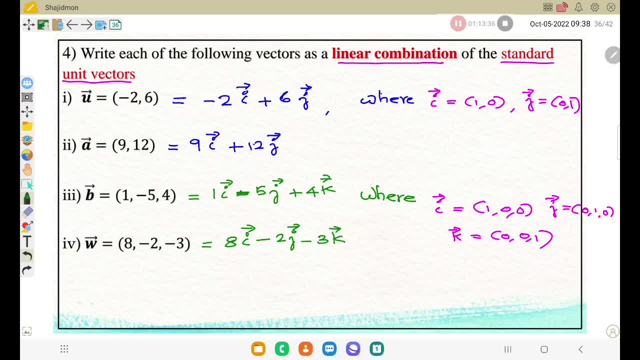 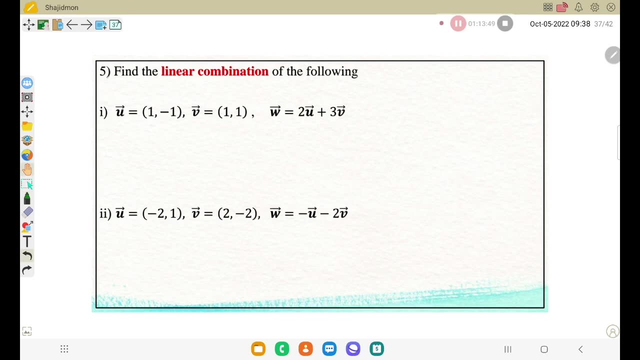 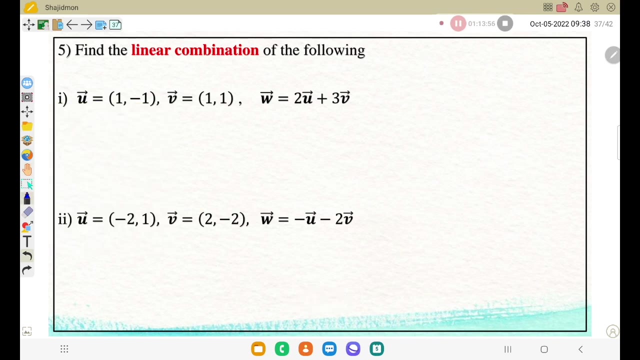 j minus 3 times vector k. So this is the vector representation in standard unit. I hope you understood this one. Okay, Now let me go to the next question, Question number 5.. Find the linear combination of the following: Find the linear combination We need to calculate. 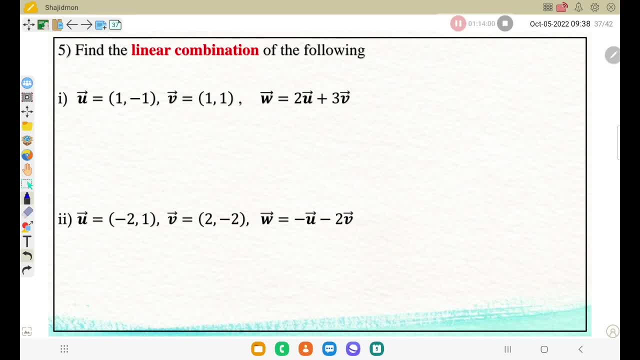 what is the linear combination? Not writing standard unit vector, Just calculate the linear combination. Okay, U means 1 minus 1.. V means 1, 1.. What linear combination we need to calculate This one? This one equal to how much? That is the question. 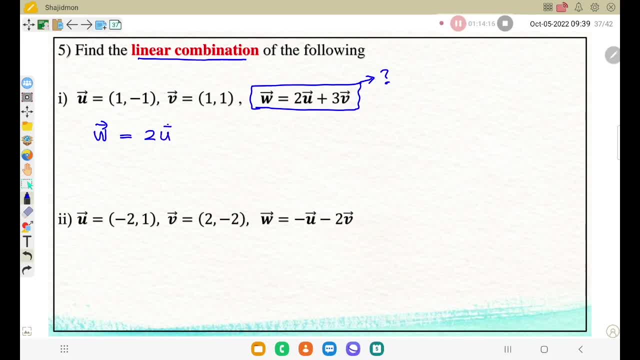 U equals 2 times vector u plus 3 times vector v. That means 2 times What is vector u: 1 minus 1.. Plus 3 times Vector v means 1, 1.. You know how to multiply 2, multiply 1,. 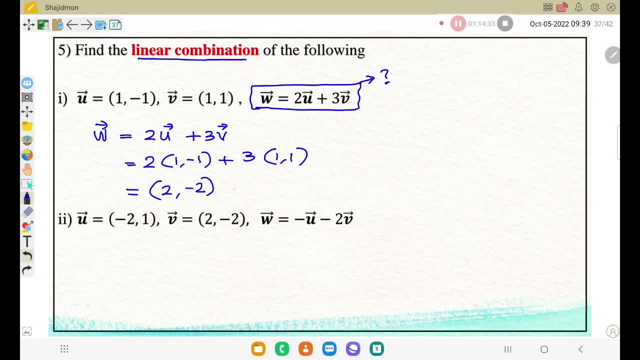 2. 2 multiply minus 1, minus 2. Plus 3 multiply 1,. 3. 3 multiply 1,, 3. After that add First number. add First number x component: 2 plus 3, 5. Minus 2 plus 3,, that is 1.. So this is the linear combination: 2 u plus 3. 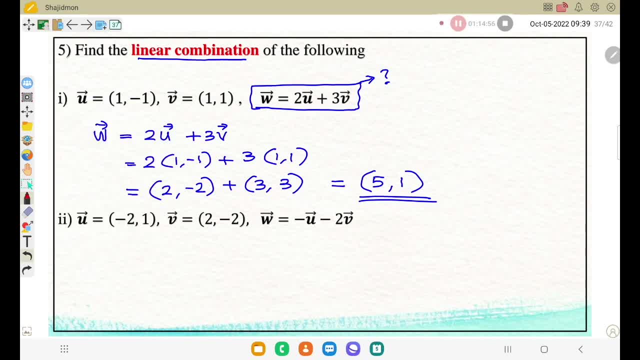 v or w vector, Say. one more model is here: W vector equals minus vector u, minus 2 times vector v. So minus What is vector u, Minus 2 comma 1.. Minus 2 times vector v, 2 comma minus 1.. From this vector, from this vector we can. 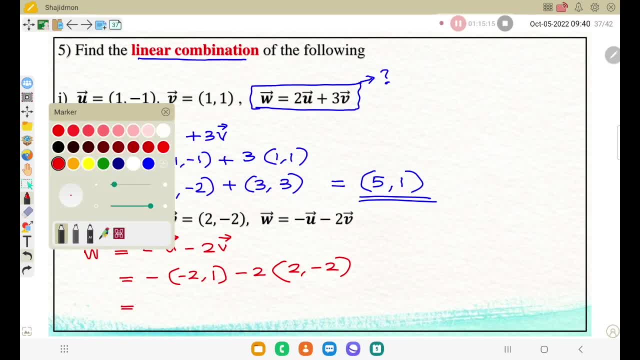 minus 2. you can expand that one. you can distribute this to here. so what will be the answer? getting equals minus multiply minus 2 plus 2 minus multiply 1 minus 1 minus. i am here distributing only that 2. you can distribute minus 2 also. so 2 multiply 2, 4. 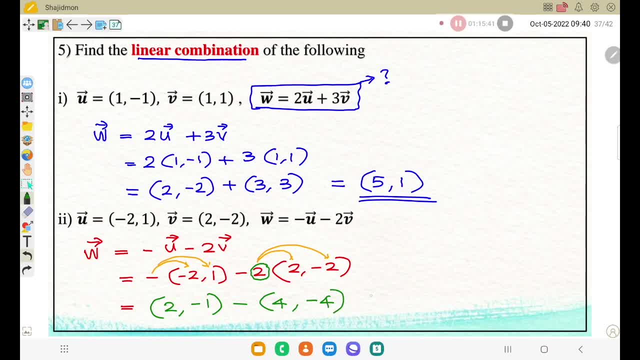 2 multiply minus 2 minus 4. now subtract these two vector. what answer you can get it: 2 minus 4 minus 2 minus 1 minus minus 4. that is minus 1 plus 4, that is 3. so this is the. 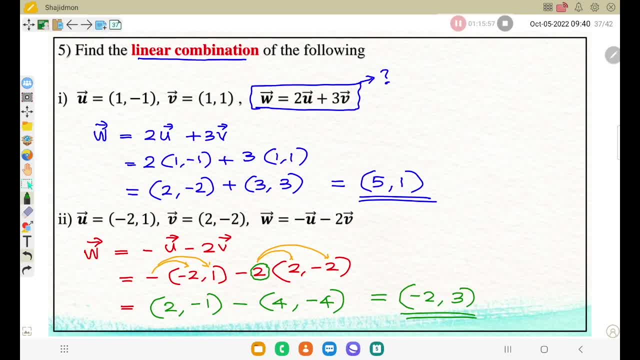 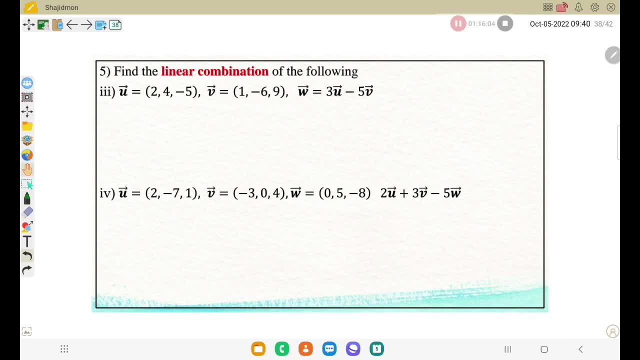 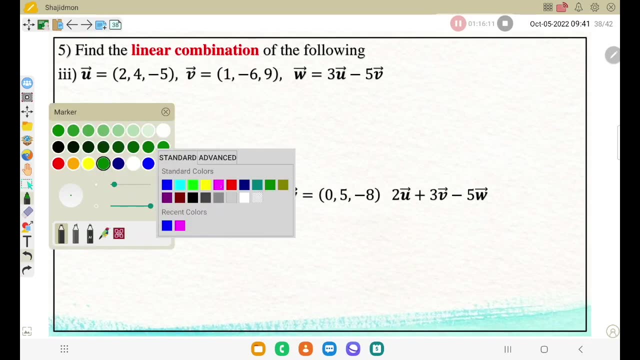 linear combination minus u plus minus u minus 2 v. i hope you understood. go to the next one, question, number 5, same model question, question number 5. you, okay, find the linear combination again. what linear combination w equals 3 u minus 5 v, correct? 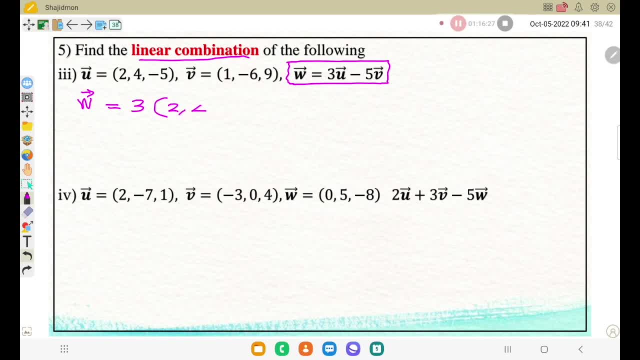 so 3 times u vector 2, 4 minus 5 minus 5 times v vector 1 minus 6, 9. so you will get 3 multiplied to 6, 6, 3 multiply 4, 12, 3 multiply minus 5 minus 15, minus 5, multiply 1. 5. okay, 5 multiply 6. 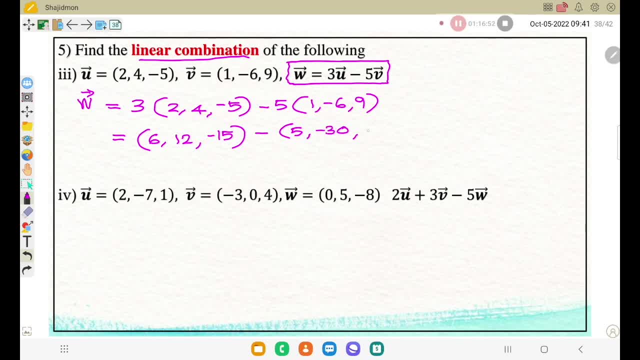 minus 30 and 5 multiply 9: 45, this minus i am not distributed. if you want, you can do minus also inside. then you can add later now what answer we will get: equal this vector minus this vector, correct. so first one: 6 minus 5, so 1. now next one: 12 minus minus 30. that means 12 plus 30. 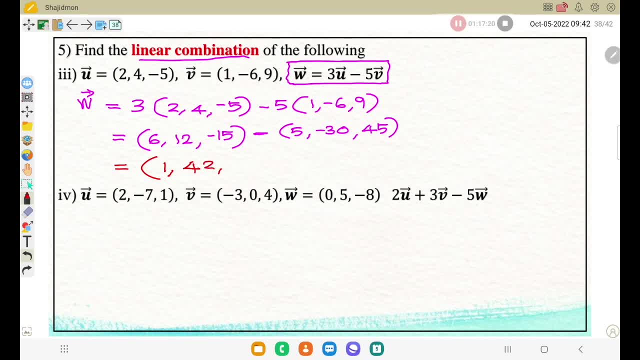 42, then minus 15 minus 45. okay, consider that minus correctly. so minus 15 minus 45, that means minus 60. so this is the linear combination: 2, 3 u minus 5 v. okay, okay, now we will go to this linear combination. we need to calculate this. this equal to how much? 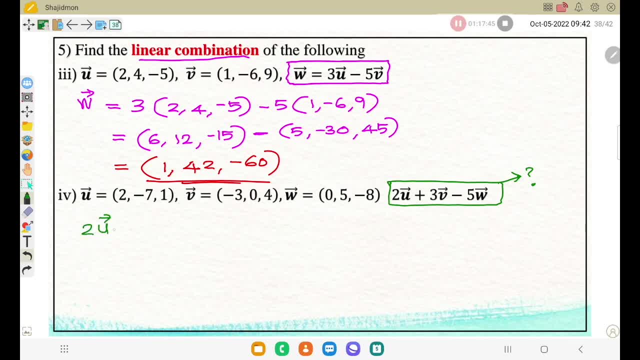 2 times vector u plus 3 times vector v minus 5 times vector w, equals so 2 times what is vector u 2 minus 7, 1 plus 3 times what is vector v minus 3, 0, 4 minus 5 times vector w. 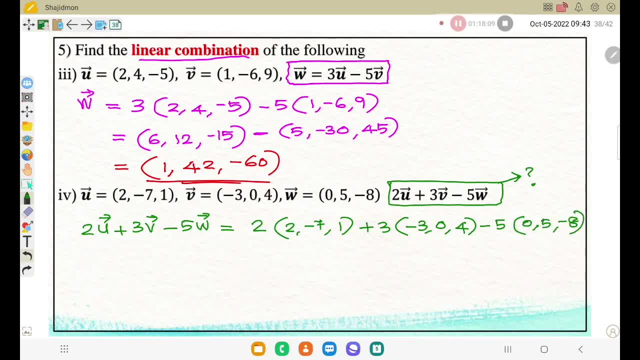 we are. İşte, that is 0, 5 minus 8. so calculate that Meredith Equals 0, 5 minus 8. so calculate first: multiply 2 to the vector, so 2 plus 3. multiply minus three: 7 minus 1, 2 plus 3. multiply minus 3 minus 9, three multiply zero. zero 3 x 4. minus 5 x 3 x 0 zero, 3 x 3 x 12 plus 3 x 4 x 12 top scale upThat is 1 and i comma grinder and that is 28, and then from this ich by 0, we will get as 8 times that times the vector 5, so 2 x 10. 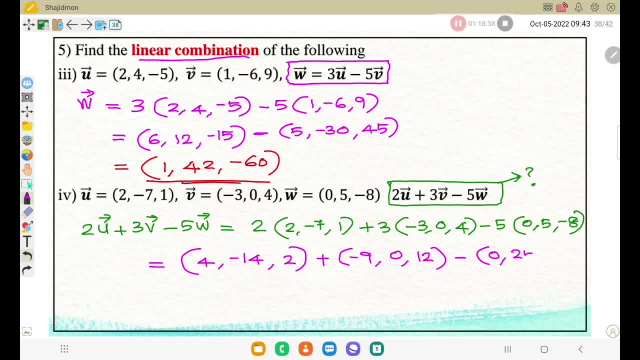 5 multiply 0,, 0,, 5 multiply 5, 25,, 5 multiply minus 8, minus 40.. Now you can write in single vector first two vector add and third vector subtract. So 4 plus minus 9 plus 0, minus 5.. 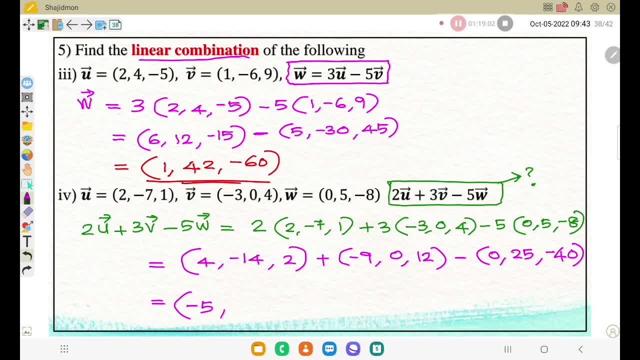 Second one minus 14 plus 0, minus 25,, correct, Minus 39.. Third one: 2 plus 12,, 2 plus 12, minus minus 40. So plus 40, 54. So this is the linear combination of that vectors. 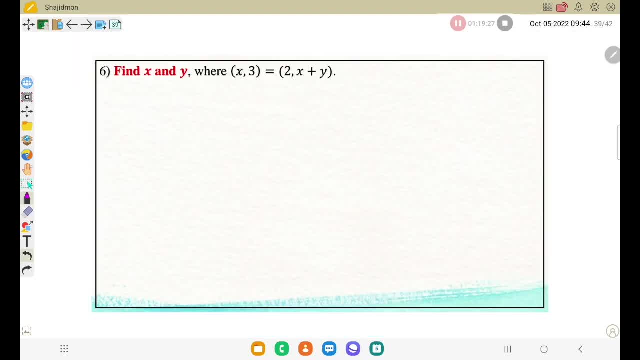 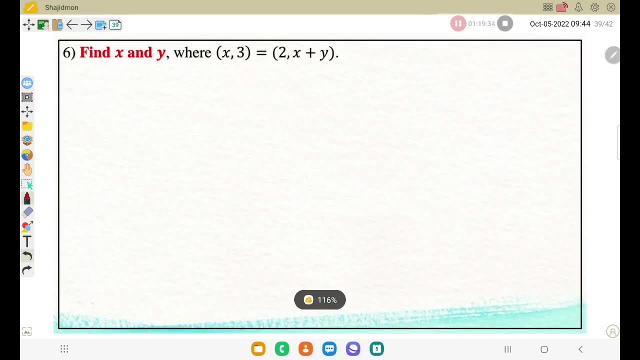 Hope you understood. Now we will go to the next one. Find the values of x and y. Find the values of x and y Where x, x3, vector x3 equal to 2 comma 2x plus y. That means one vector x3 should be equal to the second vector, 2x plus y, correct? 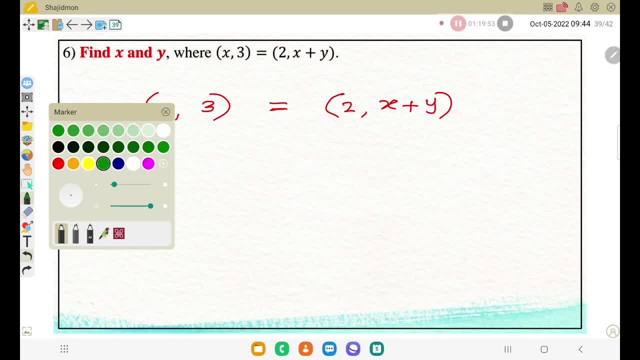 You know, two vectors are equal. we studied When we are telling two vectors are equal, vector having same magnitude, same direction. So for example, here this is vector first one, x3, correct, And 2x3.. So this is equal. 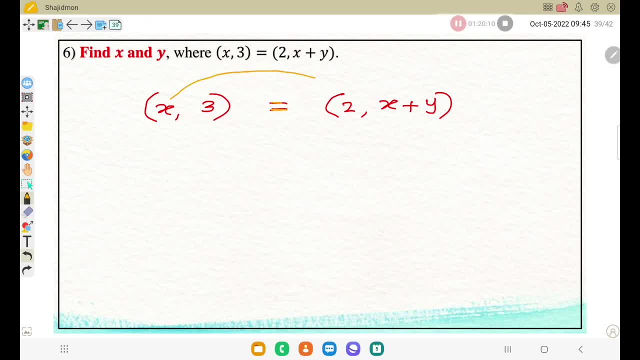 You can see this is equal to symbol. Equal means first number should be equal, second number should be equal. That is the meaning: equal vectors. okay, Now what is the first number? x? What is the first number there? 2.. 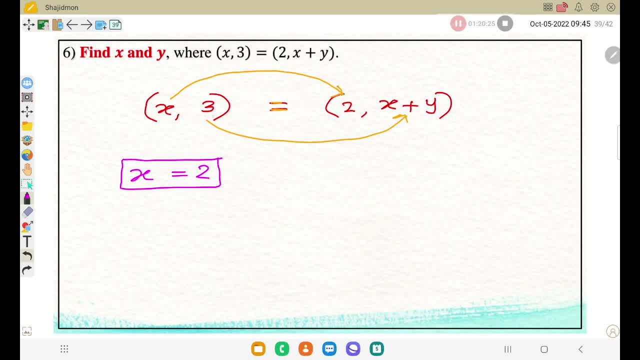 So what is the first answer: x equal to 2, okay. Now second one: 3 equal x plus y. 3 equal x plus y. That means 3 equal, You know, x number, 2 plus y. So what will be the y value? 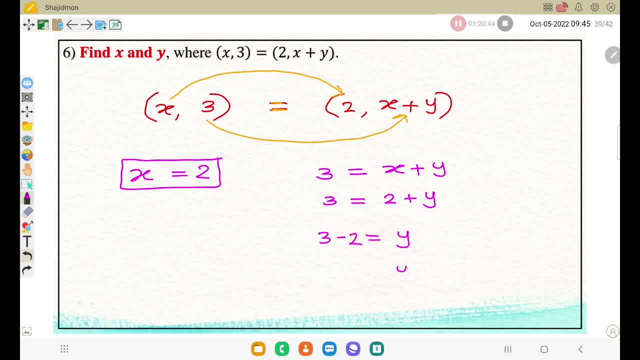 2. take to the next side, 3 minus 2.. So y equal: 3 minus 2 means 1.. So just the idea. equal vector: okay, Equal vector When we are telling two vectors are equal. this is the idea in this question. 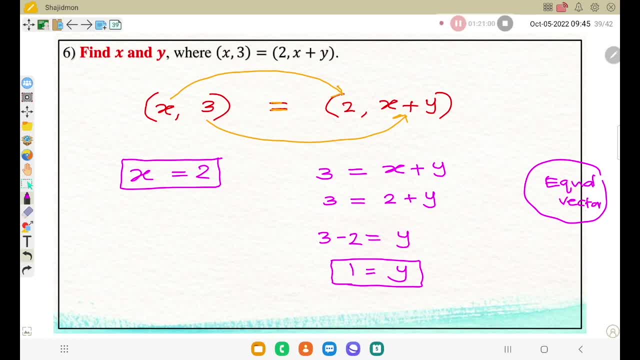 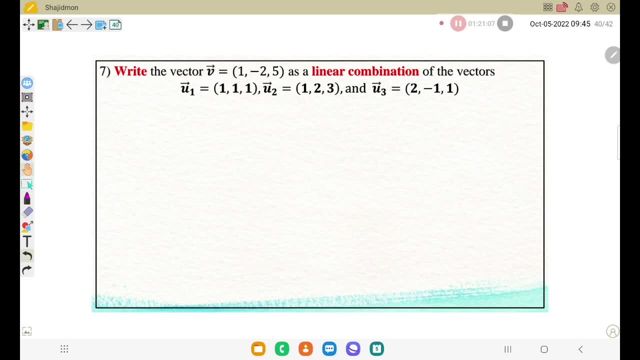 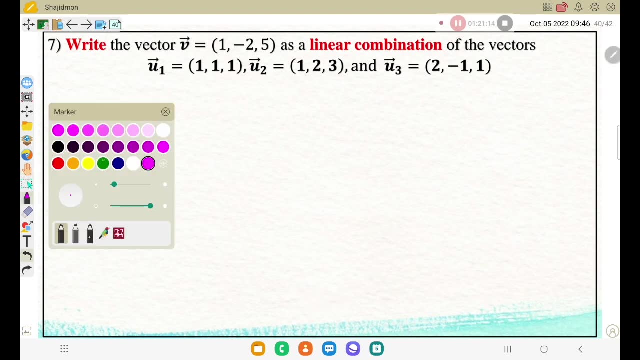 So same magnitude, same direction or components should be same. Hope it is clear to you. Now we are going to the seventh question. This is what the important question, this section: Write the vector. Write the vector as a linear combination of the vectors u1, u2 and u3. 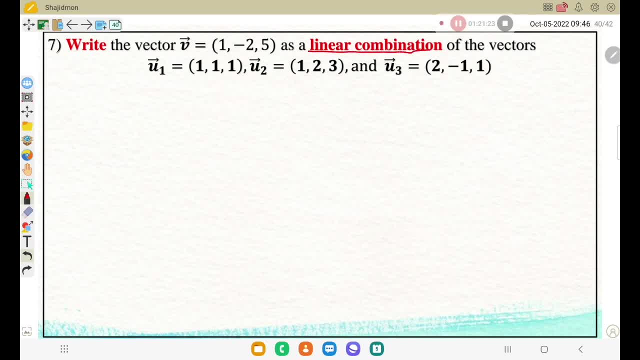 Write the vector, vector v, as a linear combination of the vector u1,, u2 and u3, okay, We discussed it. When we are telling linear combination of vectors in the plane, linear combination of the vectors. Okay, Remember this idea. 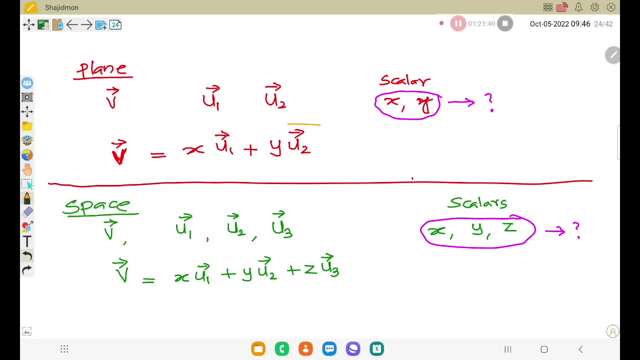 Plane means what is the linear combination we studied: Vector v equals x multiply vector u1 plus y multiply vector u2.. In space means how we are writing: linear combination: Vector v equals x multiply vector u1, plus y multiply vector u2 plus z multiply vector u3.. 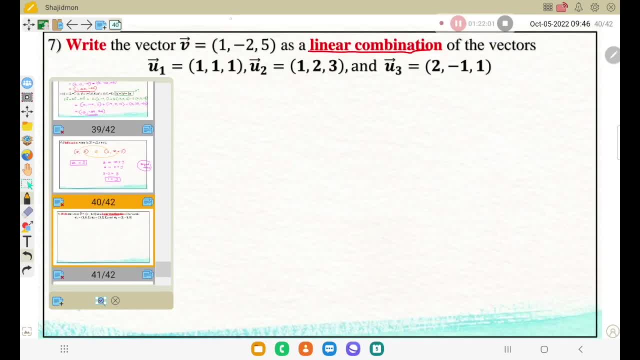 Correct, So we can go to this question using that one here. The vectors in the space: Three numbers. They are there, Correct? So linear combination means how to write the linear combination vector v as in u1, u2, u3.. 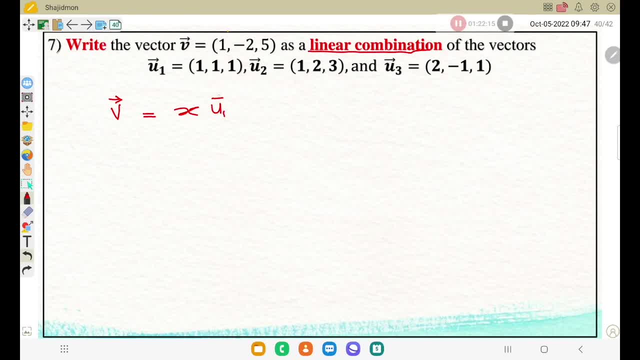 Vector v equals x multiply vector u1 plus y multiply vector u2 plus z multiply vector u3.. Okay, This is the linear combination of the vectors u1, u2, u3.. Okay, Vector v in linear combination of u1, u2, u3.. 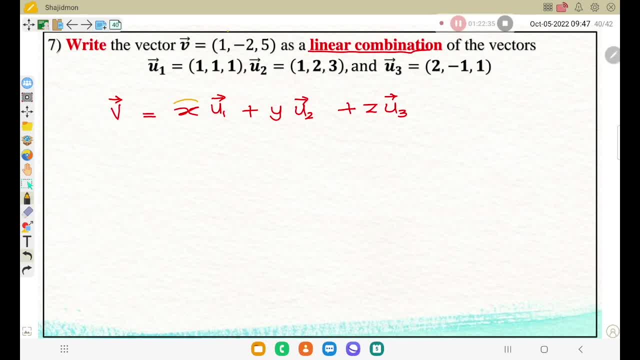 Now here, what is our aim is? We need to calculate what is x, What is y, What is z. If you are getting these three numbers, linear combination exists. We can write the linear combination. Otherwise, there is no linear combination, So we can check this one. 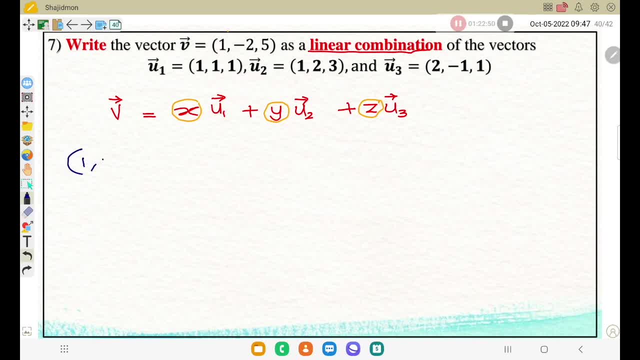 First apply vector v value. What is vector v? 1 minus 2, 5 equal x. We need to calculate u1- vector 1, 1, 1 plus y, u2- vector 1, 2 and 3.. 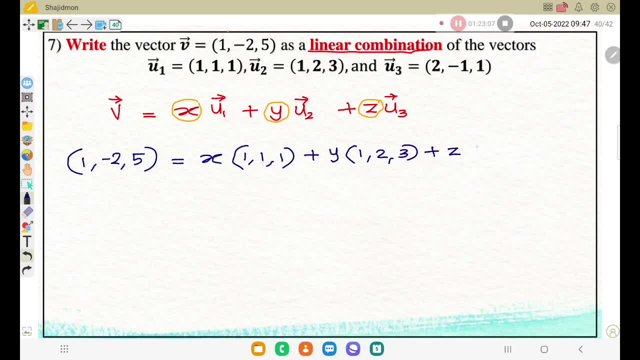 Plus z multiply what is u3, 2, minus 1 and 1.. Correct, Just apply there. That means 1 comma, 2 comma 5 minus 2 comma 5 equals x. multiply to the bracket or vector First: 1,, second, third. 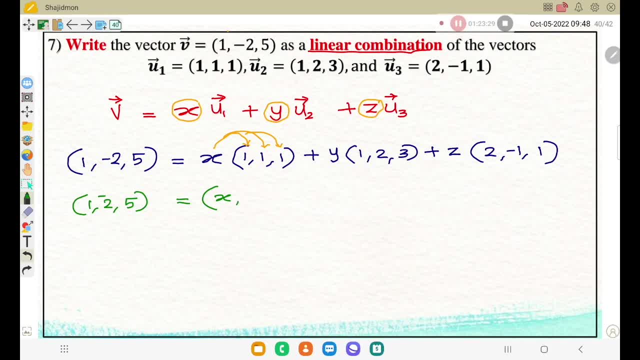 Correct, So we can write x multiply 1, x, x, x Plus y. multiply 1 means y, y multiply 2 means 2y. y multiply 3 means 3y plus z. multiply 2 means 2z minus 1z, 1z. 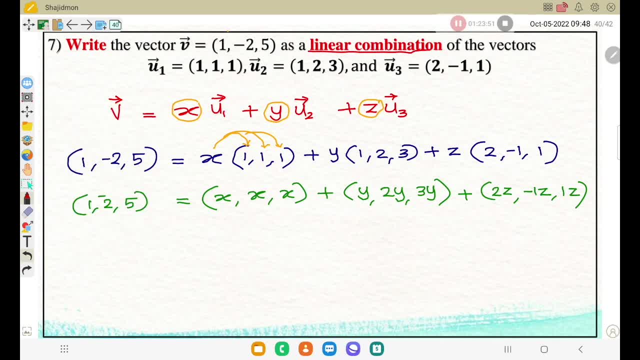 Correct, That means equals 1 minus 2, 5. vector equals: add these three vectors. First components: add first component. What is the first component here? x? What is the first component here? y? What is the first component here? 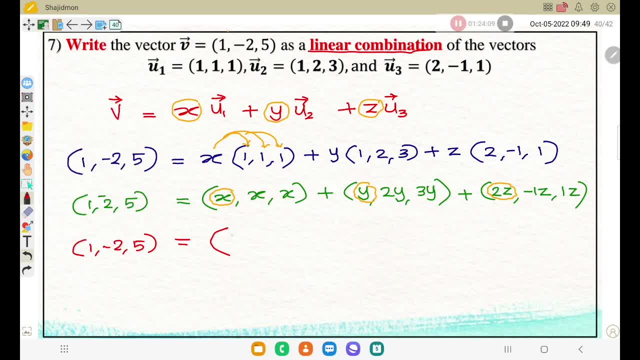 2z. Add these three Correct, So we will get x plus y plus 2z. Comma. Second components: add x plus 2y minus z. Comma. Third components: add x plus 3y plus z. 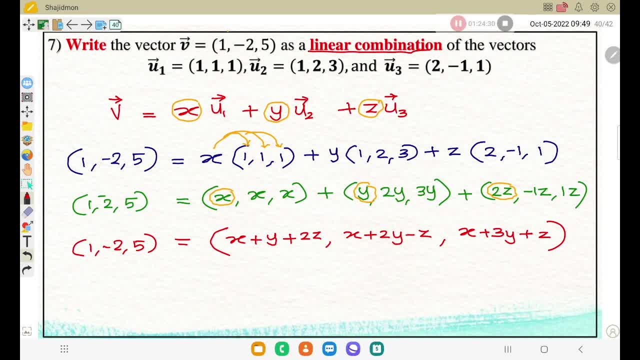 Correct: 1z means z. So what we got now We got this vector, This vector equal to this vector. Correct: This vector equal to this vector. These two vectors are equal. Equal sign. you can see: Correct Now when we are telling two vectors are equal: first component should be same, second component. 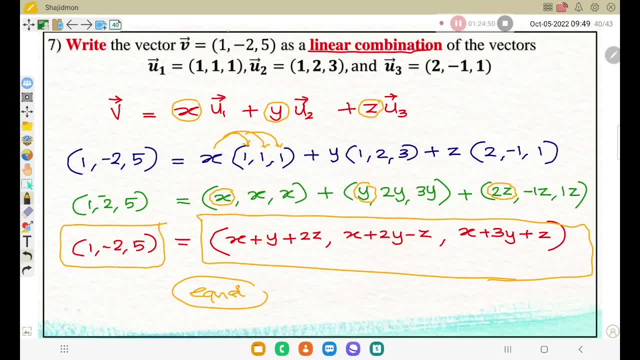 should be same. third component should be same. So what is the first component? you can see What is the first component Here: 1.. Here x plus y plus 2z, So we can write x plus y plus 2z, equal to 1.. 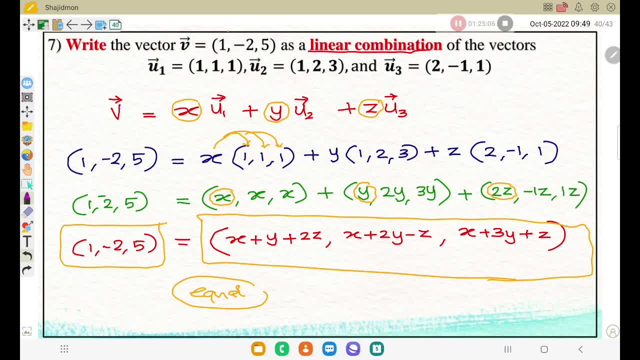 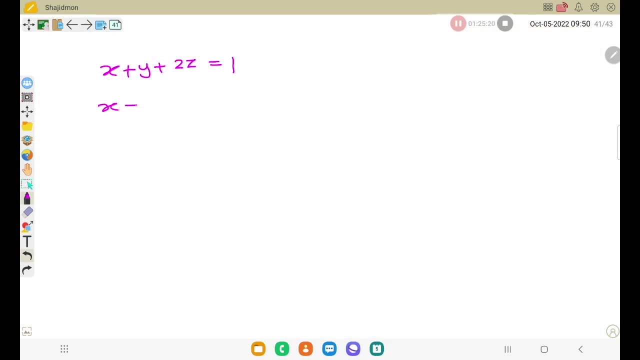 Correct. First component: equal Here: 1. First component Here: x plus y plus 2z. Correct Here: 1. These two are equal. Now second component: x plus 2y minus z. x plus 2y minus z, equals minus 2.. 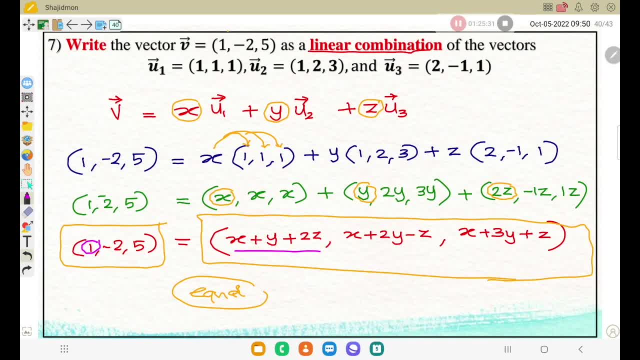 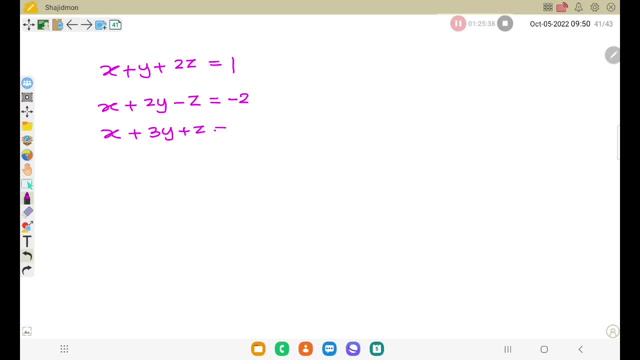 Now, third component. What are the third component, x plus 3y plus z? x plus 3y plus z equals. what is the third component here? 5.. So we can write: it is 5.. So we got one system of equation now. 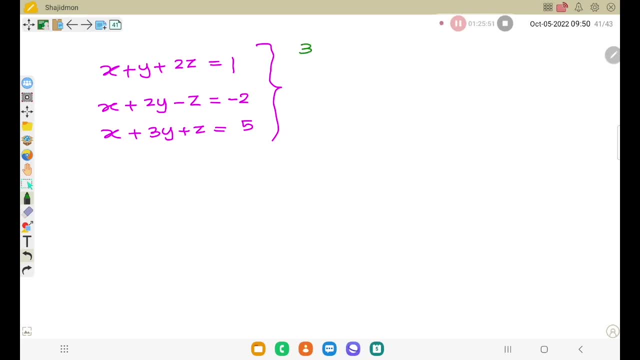 How many equations are there? Three equations. How many unknowns are there? We have three unknowns: x value, y value, z value, Three unknowns, We don't know that value Correct. So it is. we are calling a 3 by 3 system. 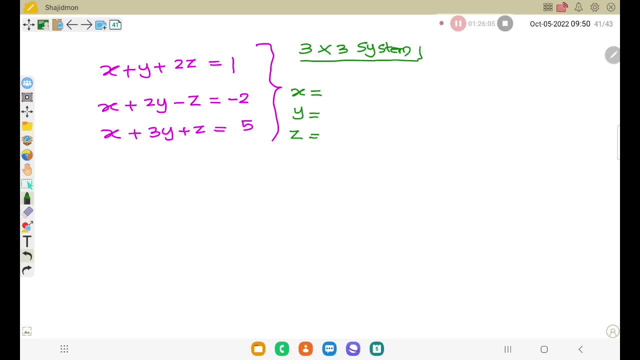 What is we are calling 3 by 3 system, Because 3 equation and 3 unknown. From this 3 by 3 system, we need to calculate what is our x, what is our y and what is our z. This is we are doing by using calculator. 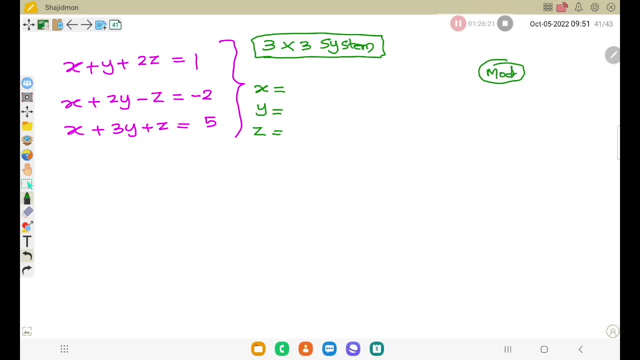 So, just to go to the calculator, you can just press the mode button. After that, number 5 equation. Number 5 equation After that. After that you can see one option: anx plus bny plus cnz equal to dn. Correct, Because here we have, we need to find three variable: x, y and z. 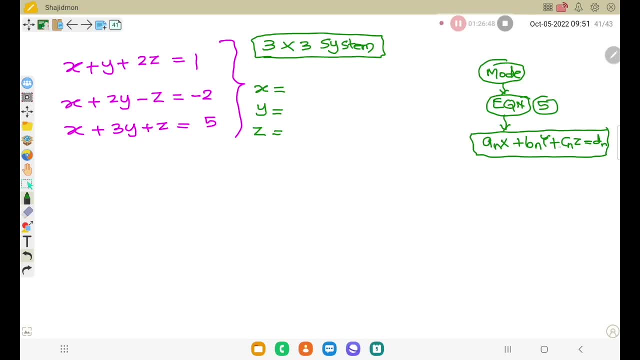 That is why we are choosing anx, bny, cnz. That is number 2 in your calculator, Number 2.. So once you are clicking number 2, calculator is asking some numbers. Okay, These three equations behind numbers we need to enter there. 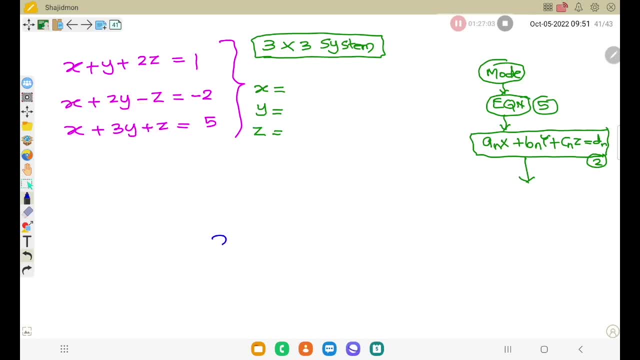 Enter there For example: first equation: x plus y plus 2z equal to 1.. What are the behind number? you can check What is the x behind number 1.. So you can press 1.. Equal to. After that press equal to. 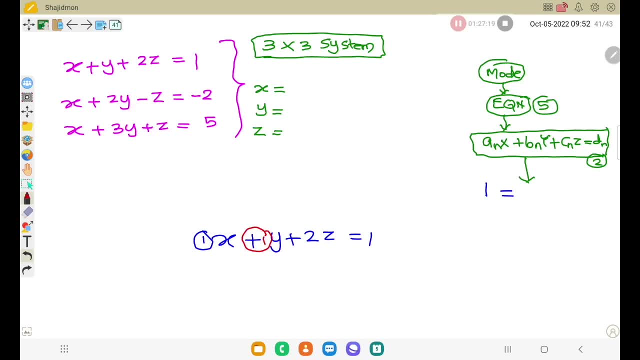 Okay, Then y behind number. What is y behind number? 1. Press equal to Okay. After that, z behind number. What is that? 2. Press equal to Right side number. 1. Press equal to Okay. 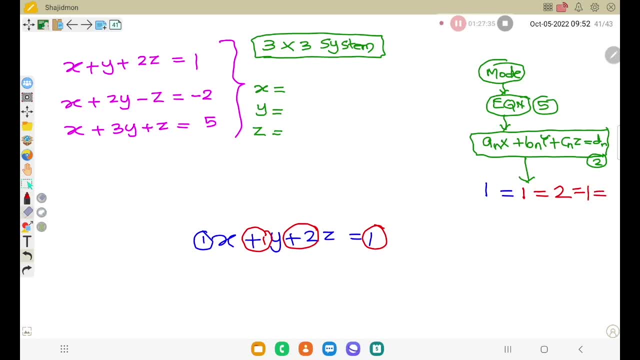 Like this. continue in the second equation also. Second equation: also same thing we are doing. What is second equation: x plus 2y, minus z, equal to minus 2.. So what is x behind number 1. So press 1 equal to. 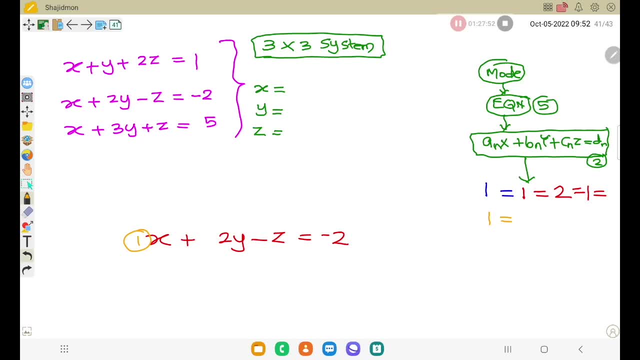 Okay, You can calculate same like this. Okay, So press 1 equal to After that y behind number 2.. Press equal to After that z behind number minus 1.. Don't forget that minus Minus 1.. 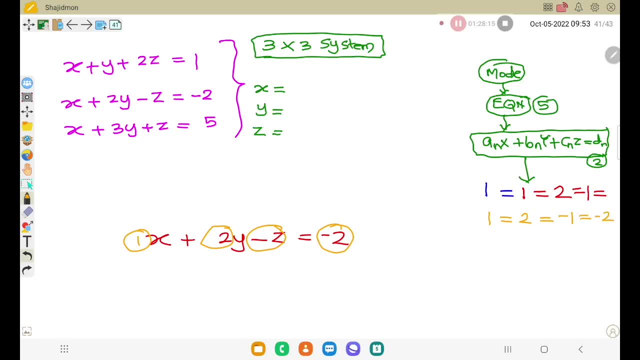 Press, equal to Right side number minus 2.. Correct, Then again, go to the third equation, Same like. go to the third equation: x plus 3y plus z equal to 5.. So what is x behind number? you can think 1.. 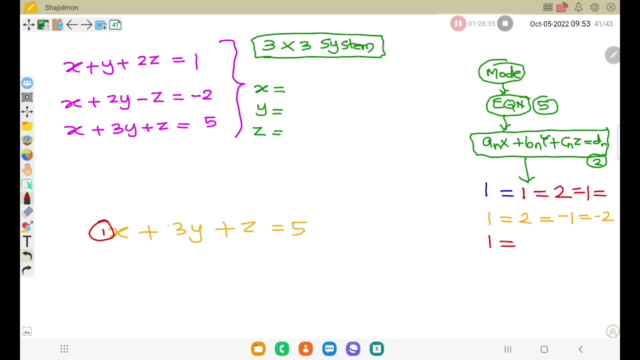 So press 1 equal to After that y behind number 3.. Press equal to After that z behind number 1.. Press equals After that right side number 5.. Then press equal to After that, Okay, 5.. 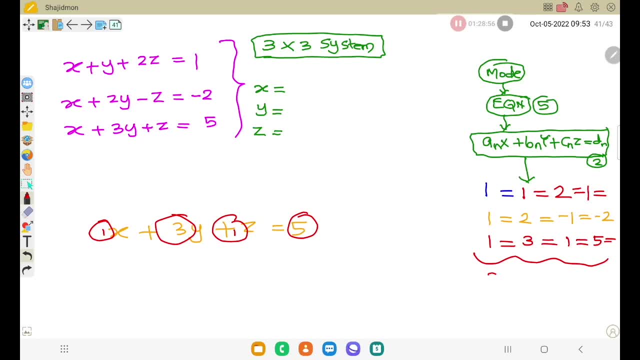 Press equal to So calculator immediately showing your x number minus 6.. Press equals, You will get y number. 3. Press equals, You will get z number, that is, 2.. We will get the solution easily from the calculator, Okay. 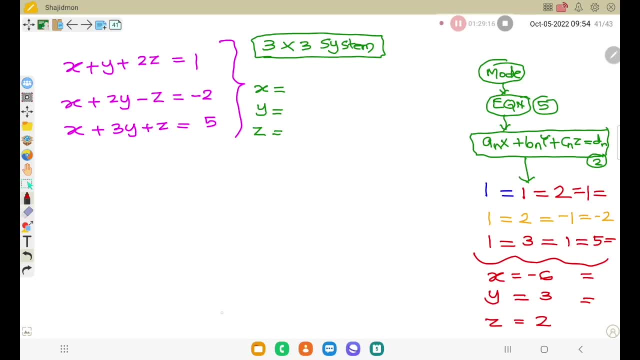 Now, if you want to return back same calculator mode, Return, Okay, Press the mode button And 1. Mode 1.. That is the normal computation mode, Mode 1.. Okay, So don't forget this step from calculator. Now see here we need to be careful, like here: 3 variables are there. 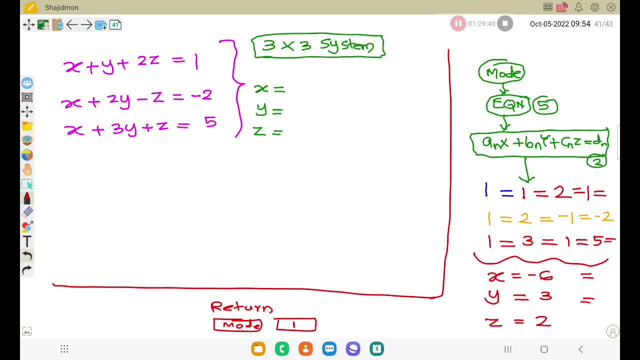 x, y and z. Okay, If it is 2 variable, you can use number 1.. Number 1 in the calculator Instead of 2, you can use number 1 in calculator. Okay, So that you will get it. So I am writing here the values now. 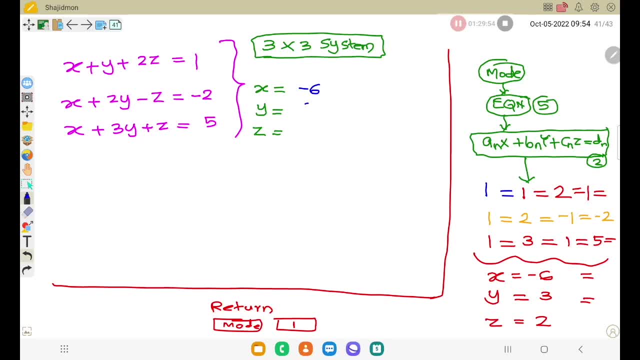 x value minus 6. y value, 3. z value: 2. If you are missing some numbers, answer will be different. So carefully enter Now. So x number, y number, z number, we got. So if you got y number, x number, z number, meaning is linear combination exist. 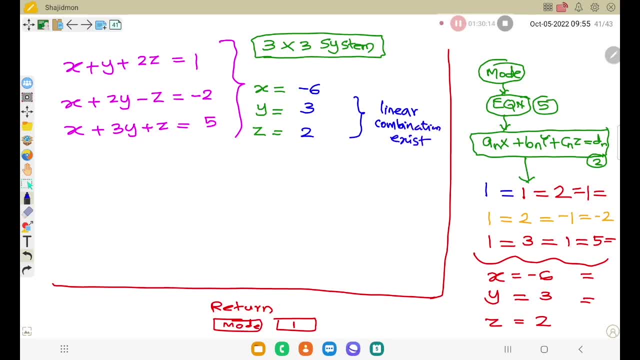 Okay, We can write the linear combination. Correct, Now we write the linear combination. See, this is the linear combination: v equal to x, u1 plus y, u2 plus z, u3.. So we are writing the answer. So we are writing the answer: vector v equal x. 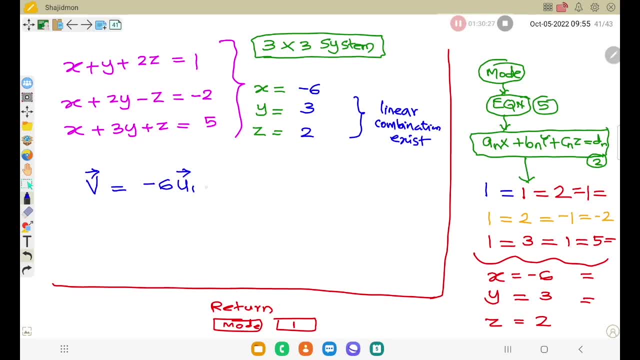 x means minus 6.. Multiply u1 vector plus y, that is 3.. Multiply u2 vector plus z, that is 2. Multiply u3 vector. So this is the linear combination Vector v as a linear combination of u1, u2 and u3.. 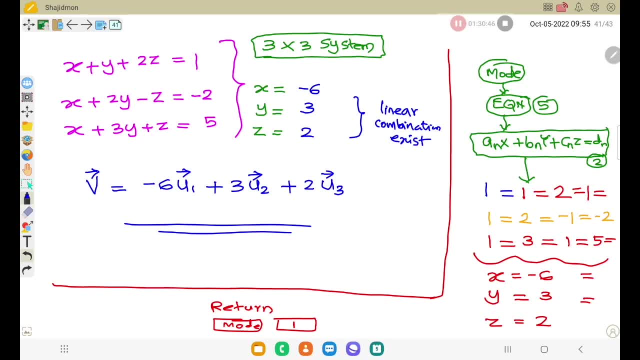 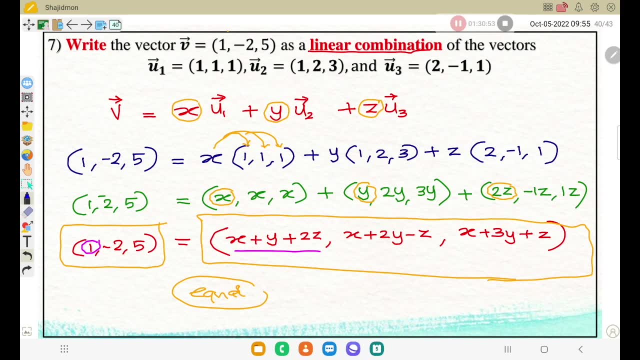 That means vector v. we are representing the vectors u1,, u2 and u3 in terms of Okay Linear combination, So I hope this question can practice same like this: This is in space Plane- means vector v equal to x- u1 plus y- u2.. 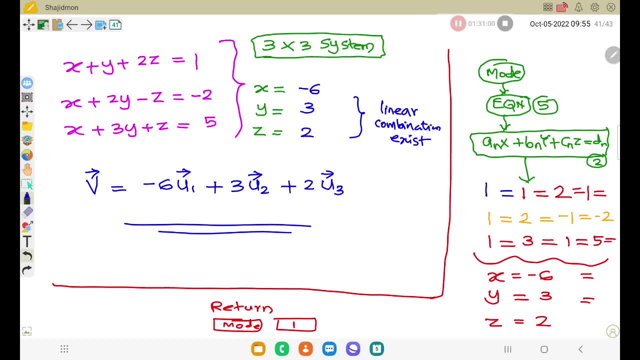 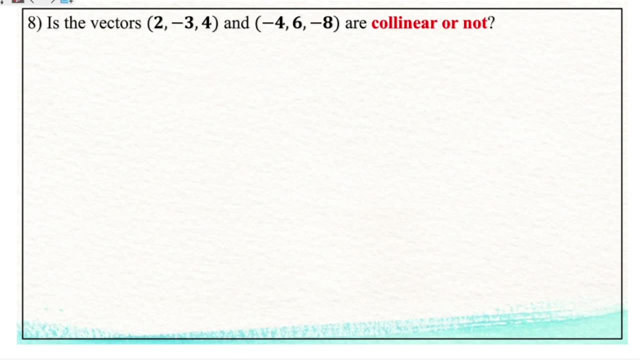 Only 2.. Correct, Here z also will come. So find x, y, z using calculator and apply there in the linear combination. I hope you understood this question. Okay, Now let me go to the question number 8 here. So is, the vectors 2, minus 3, 4 and minus 4, 6, minus 8 are collinear. 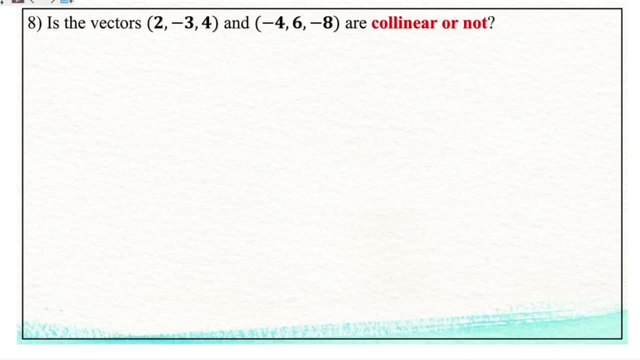 6 minus 8 are collinear or not, Correct? We are discussing what is the meaning of collinear, Correct? What is the meaning? vectors that are lie along the same line or parallel line? Correct? We are said to be collinear vectors. 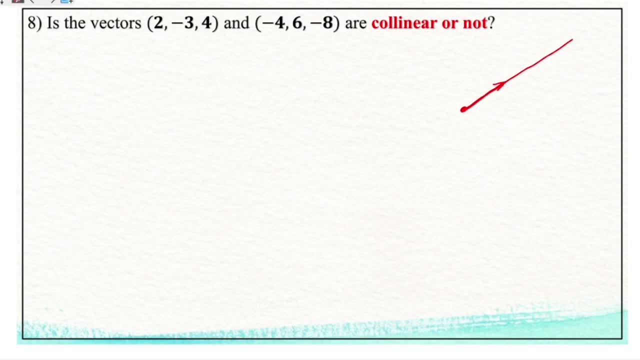 That means these vectors are coming along a same line. For example, this is vector u and this is vector v. So these are collinear vector, Okay, Vectors that lie along the same line, or parallel lines also, parallel vectors also. we can consider: 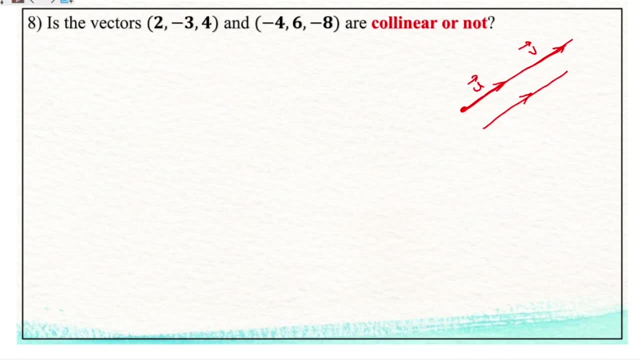 as the collinear vector. So we will check these two points. these two vectors are collinear or not. For example, first vector I am just taking as u equals 2, minus 3 and 4.. Second vector: I can take it as vector v equals minus 4, 6, minus 8 in component form. 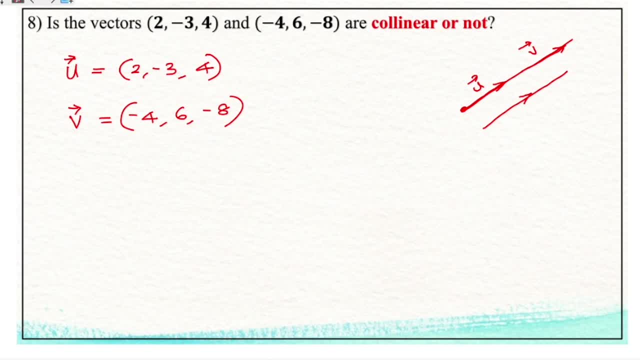 Correct. Now what we need to check, We can check two way. First idea is the ratios of the components. Correct, The ratios of the corresponding components. Okay, Are same. Components should be same. Correct, Are same. I am just doing that one. 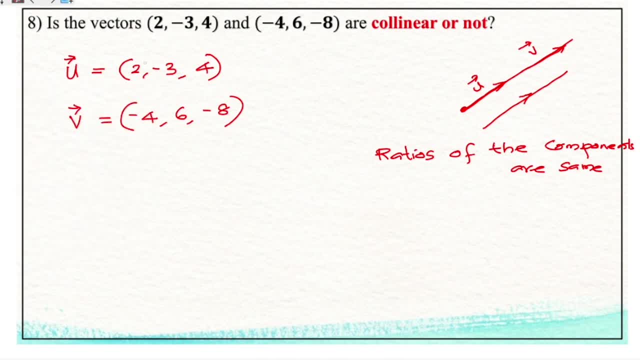 So we can check that one Is it same or no. For example, x component of the first vector, that is, 2 divided by x component of the second vector, minus 4.. So 2 divided by minus 4.. Correct, Minus 1 divided by 2, you will get minus 0.5. 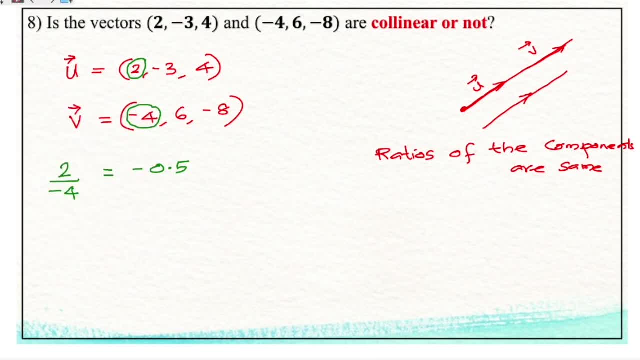 Correct. Now take the second components ratio: y components ratio Minus 3 divided by 6.. Correct: The y component in the first vector minus 3, second vector 6. So minus 3 over 6. also we will get minus 0.5. 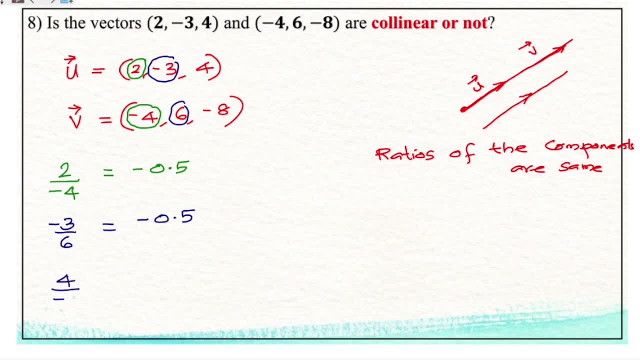 Same way. the third component, 4 divided by minus 8, also equal to minus 0.5.. So what is the conclusion? All these ratios are same, Correct: 2 divided by minus 4 is same as minus 3 divided by x. 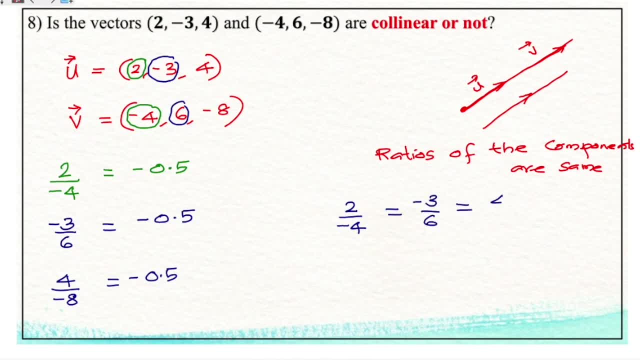 Correct: 6 same as 4 divided by minus 8.. All these ratios are same. Now the ratios of the components are same means that 2 vectors are collinear vectors. I hope you understood okay this way. And the same question. we can do the second way, as if 2 vectors are collinear, one of the 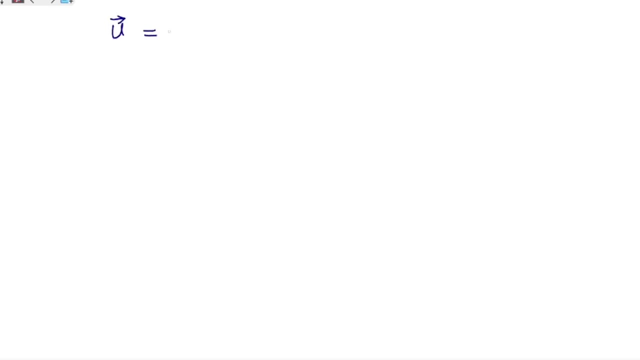 vector equal to, for example, vector u, equal to a scalar multiple of the second vector. Okay, So vector u is equal to vector u minus 3 divided by v. K means a scalar or a number multiplied with the second vector. If you are getting like this, that 2 vectors are collinear. 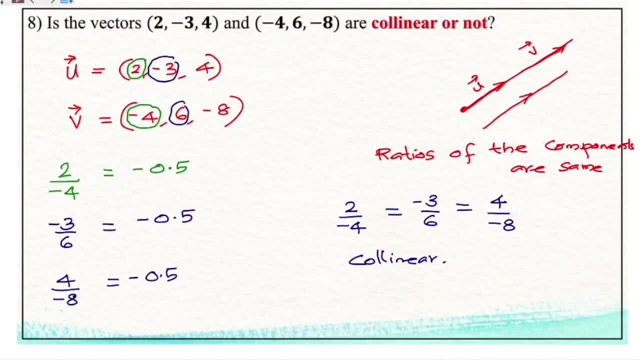 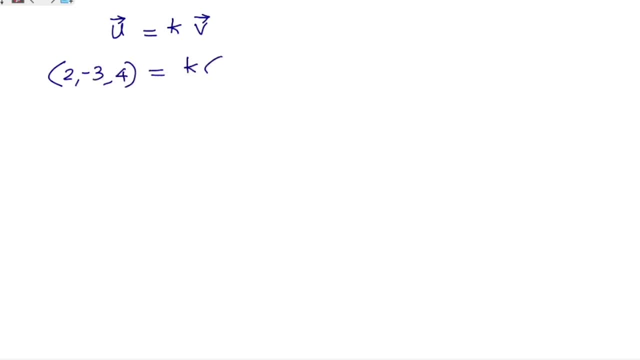 For example here: what is u here? 2 minus 3 and 4.. Correct: 2 minus 3 and 4 equals k multiplied. what is the vector v here? Minus 4, 6, minus 8.. 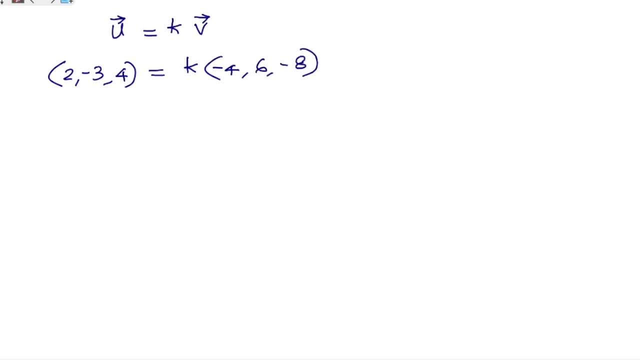 Minus 4, 6, minus 8.. Correct. Now just to simplify, if you are getting k value, that 2 vectors are collinear vectors, linear vectors, correct. so 2 minus 3 and 4 equal to k. we can multiply to inside minus 4, multiply k. 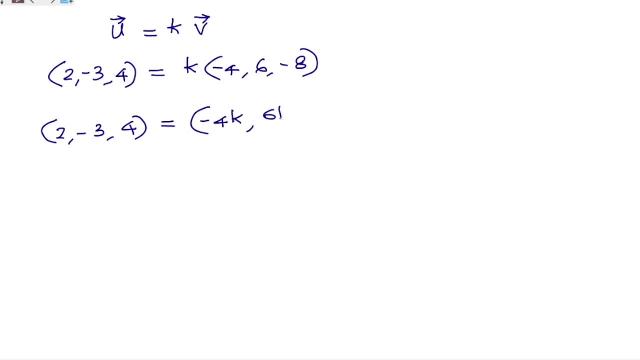 minus 4 k and 6 multiply k, that means 6 k and minus 8 multiply k here: minus 8 k, correct? now just check what is the value of k here. that means this vector equal to this vector, correct, equal. so what will be? what is the meaning of equal? we can take the first components. first components. 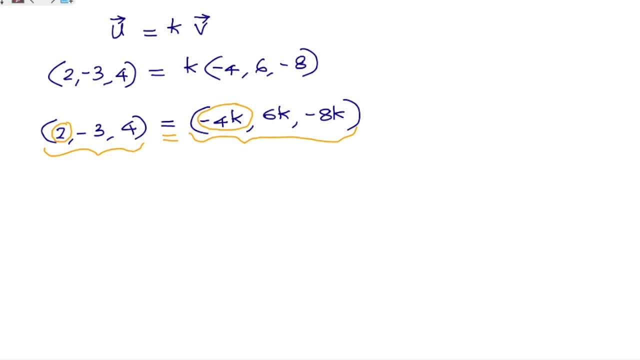 should be same. second will be same. third will be same. first component itself. we are getting k value. what is the k value? 2 equals minus 4 times k, correct? that means what will be the k value? k equals 2 divided by minus 4. that means the k number is minus 0.5. whatever the ratio we are, 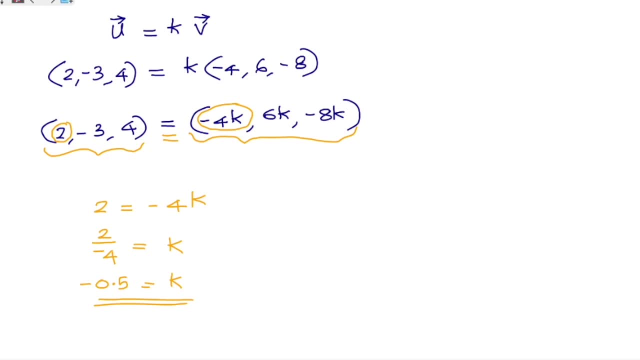 getting there that the same number, getting here k value, k equal to minus 0.5. see, here we are getting the ratio minus 0.5. that ratio is the k value, correct. so we got k equal to now. if you are getting second component, also same thing we are getting. 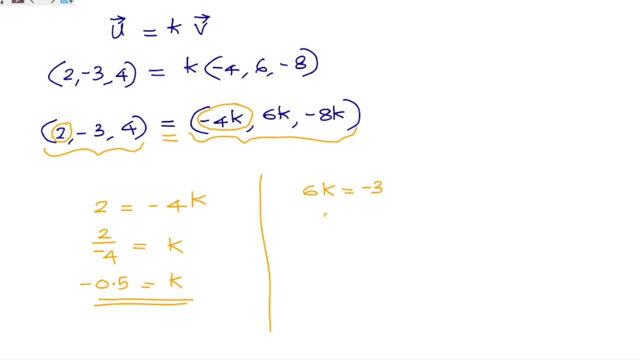 for example, 6k equal to minus 3, correct, so k equal to minus 3 divided by 6 and also equal to minus 0.5. and the third component, if you are taking minus 8k and equal to minus 8k, equal to: 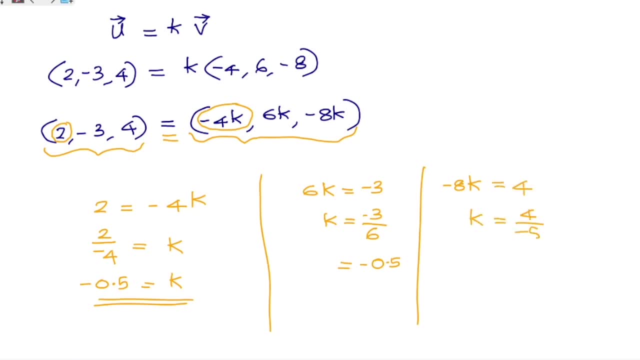 4. so same k equal to 4 divided by minus 8 equals minus 0.5, correct, so same idea. we are getting k value same, equal to minus 0.5. so these two vectors are said to be collinear vector. that means how can we write: vector u equals a constant. what is the k scalar number minus 0.5 multiply? 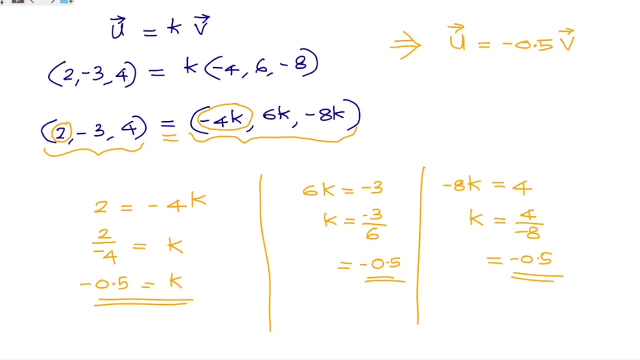 vector v correct, if you can write like this: one vector equal to a scalar multiplier. second vector means that two vectors we are telling collinear vectors. So this is the simple idea. here You can see the idea of the collinear, okay. Or when we are thinking itself: see, the idea is. 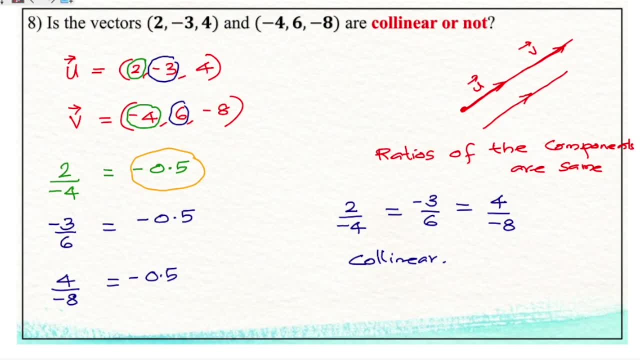 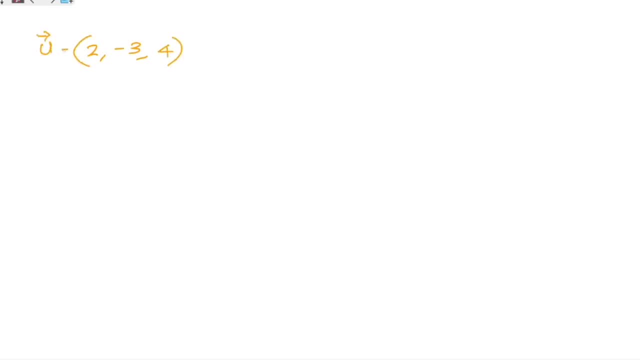 very simple, For example, this question: you can see first vector 2, minus 3,, 4, correct 2, minus 3 and 4.. This is vector u, okay, And vector v. what is vector v here? Minus 4, 6,, minus 8,, minus 4,.